I just need you to understand where it comes from. You got it? 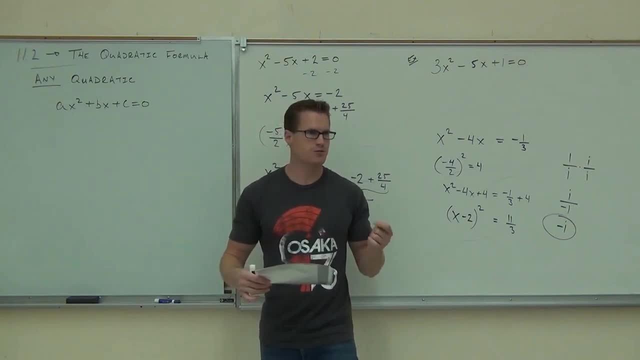 So take notes if you want, but I'm going to move pretty fast. I just want you following. 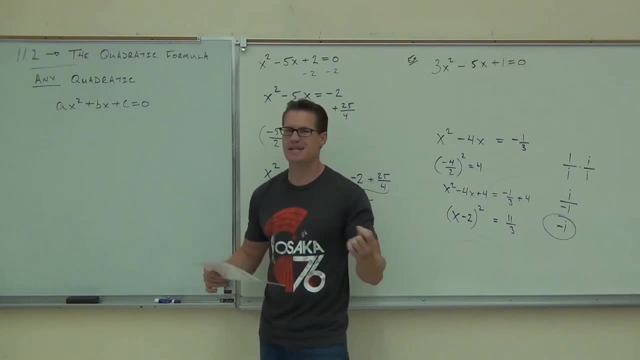 I want you to follow each step and see, oh, this is where it comes from. Because I always hated it when my teachers would give me formulas but never exactly explained how you got them. Like, well, fine, I can use that, but it doesn't make any sense. What we're doing here is we're going to solve this in general by completing the square. Notice, I haven't told you what A is. What B is. And what C is. I'm going to solve it anyway. It's not good like that, you know? Whatever. 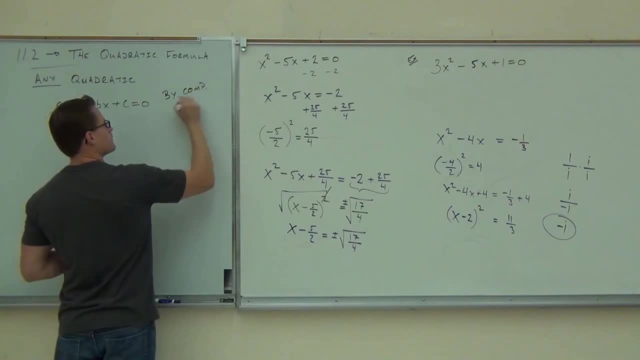 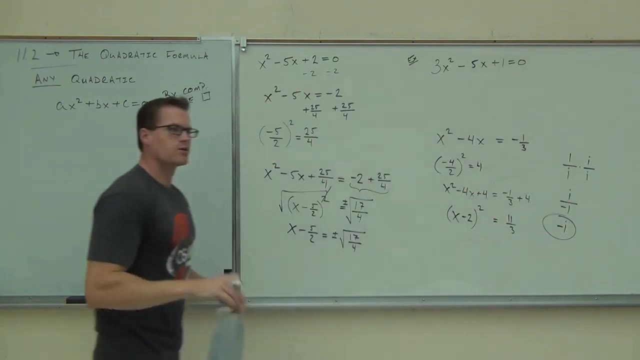 So this is by completing the square. We're going to follow the steps to completing the square right now. The steps to completing the square said, first off, you need to get your constant term off to the other side. You follow? What's my constant term here? Cb. I'm going to subtract c. 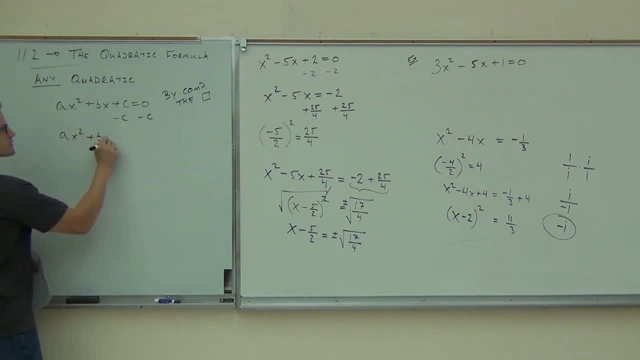 So I get ax squared plus bx equals negative c. True? 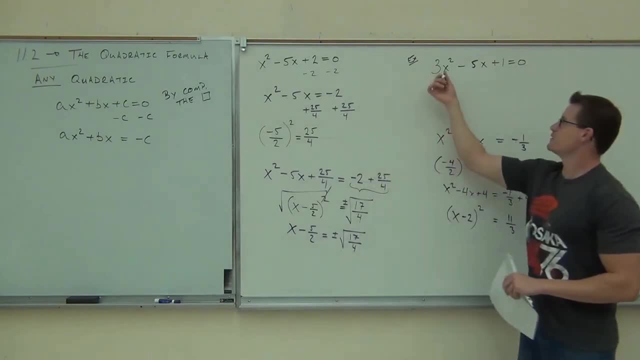 The next step was, step number two said, you need to somehow get rid of that coefficient. What's the coefficient I need to get rid of here? A. 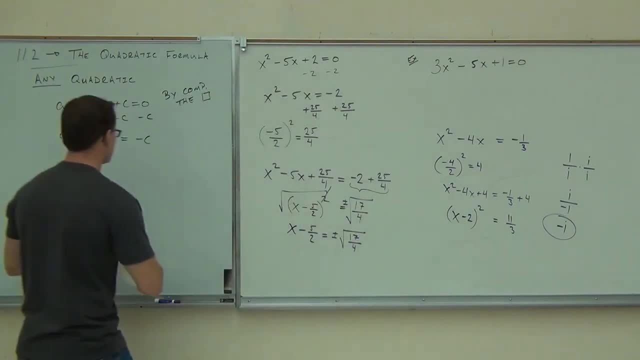 So I'm going to divide everything by a. What happens is I'm going to get x squared. What's the coefficient I need to get rid of here? I'm going to get x squared plus b over ax, notice how that's a fraction, equals negative c over a. 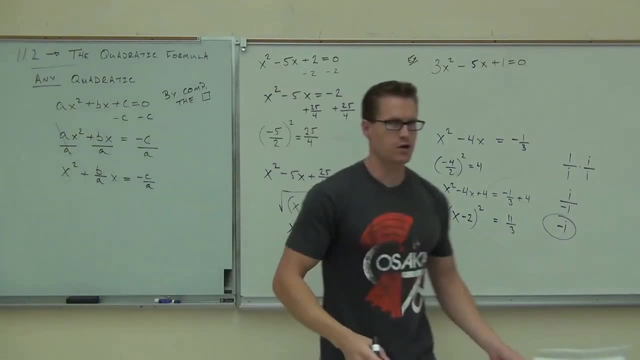 Are you still okay so far? Are you sure? 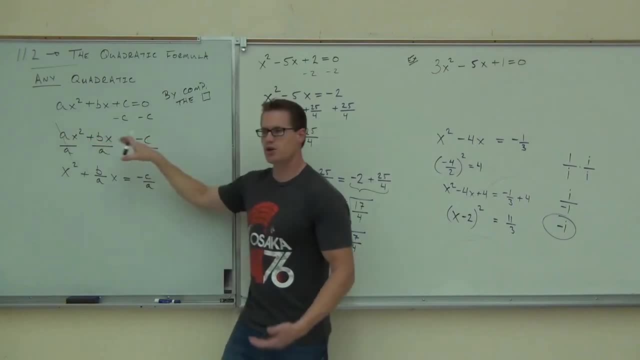 So constant term, gone. Divide by that coefficient, no problem. I have that. 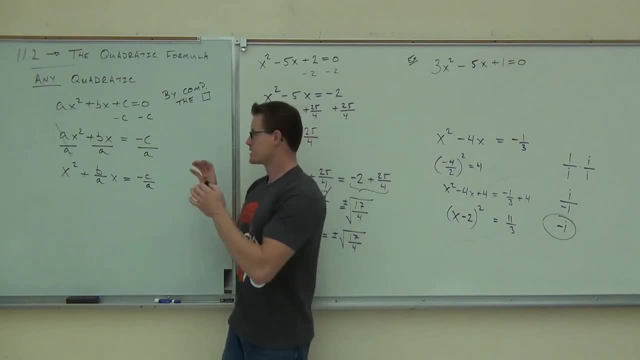 Next step was the moneymaker step. It said, take that middle term. This one. 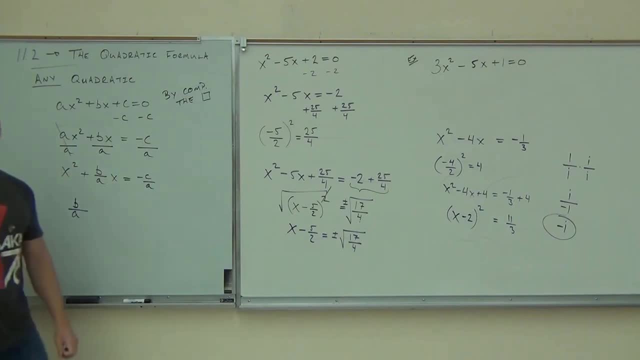 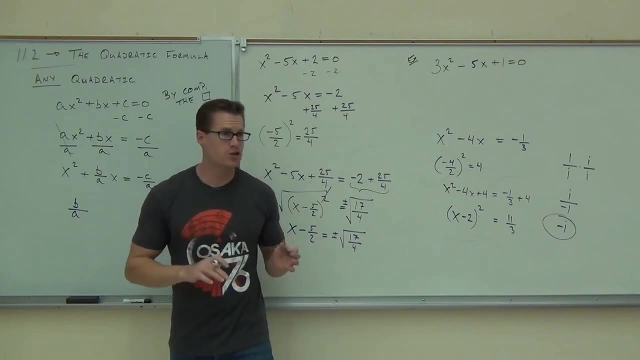 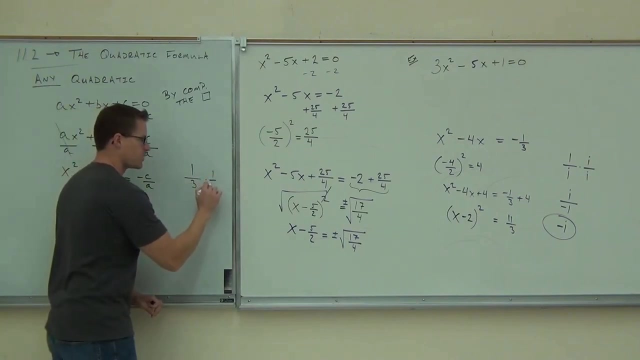 Take half of it. Now, let me show you something in case you never saw this before. If you want to take half of a fraction, for instance, if you want to take half of one-third, half of one-third would be the same thing as multiplying by one-half, right? That's going to be one-sixth. In other words, to take half of this fraction, you just put a two there. 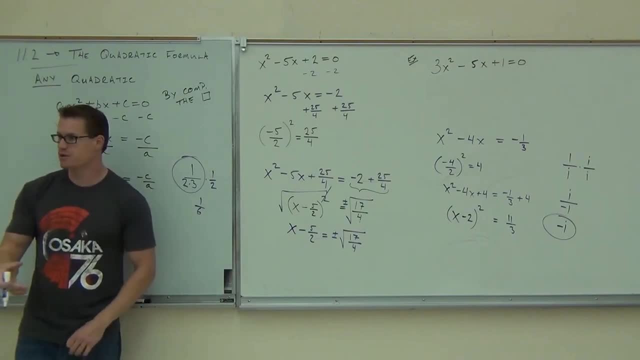 You multiply by two on the denominator, and that takes half of it. You're basically dividing by two. You okay with that one? 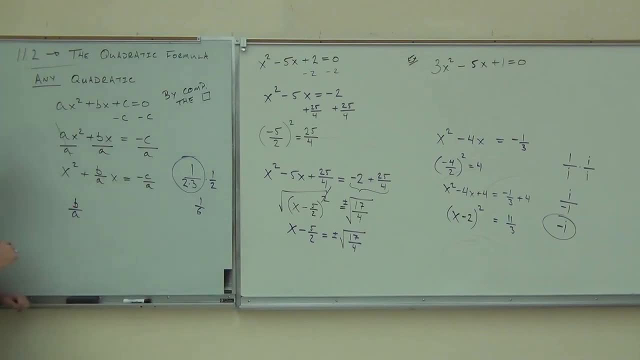 So if I want to take half of b over a, what I'm going to do is say, oh, b over a, half of that, is b over 2a. That's half of b over a. Are you okay on that one? 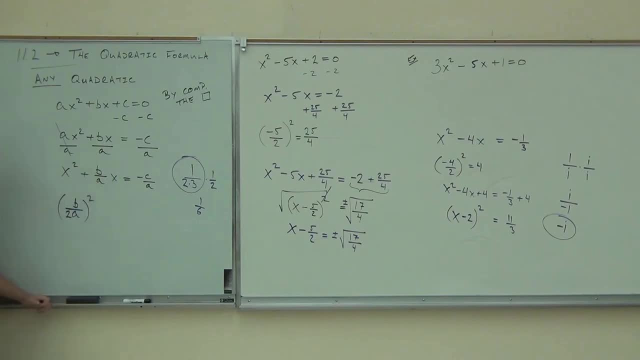 So I take half of this term, and I square it. That's exactly what we did here. We took half of this, divided by another two. 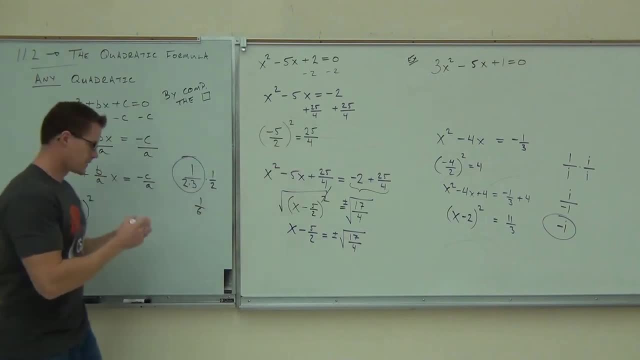 We divided by another two here. Then we squared it, and we got this thing. And we added that to both sides. So I'm going to add, so notice this is b squared over, what's this, b squared over, over how much? 4a squared. 4a, 4a? 4a squared. You agree that this is this? Remember, this is the key step here. 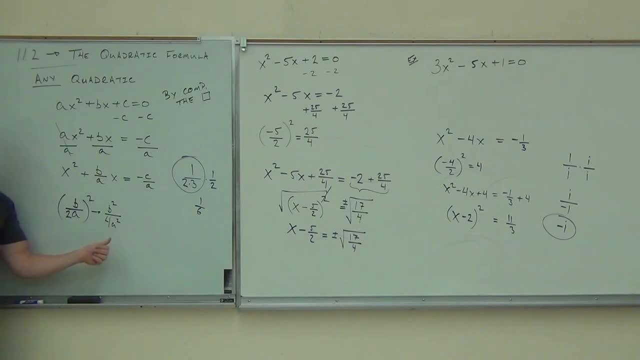 I've taken half of this, check. I've squared it, check. I've added it to both sides. Well, not yet. I'm going to add this to both sides. 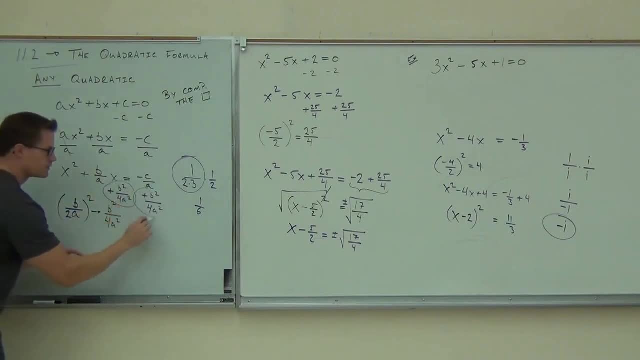 So I'm adding this, b squared over 4a squared, to both sides. Well, this is going to give me, watch carefully. On the left-hand side. I have x squared, plus b over ax, plus b squared over 4a squared, equals, on the right-hand side, 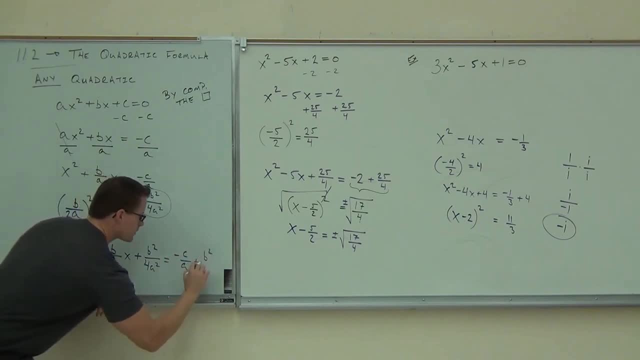 I have negative c over a, plus b squared over 4a squared. 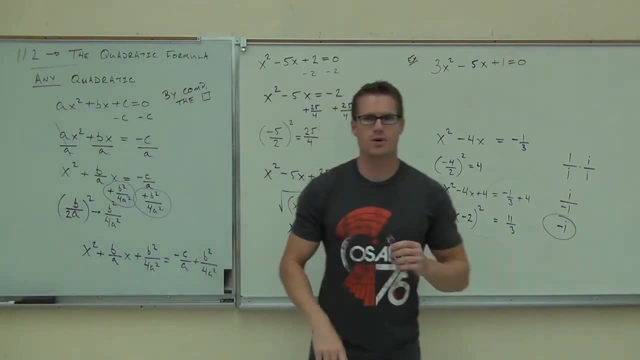 That was the hardest part. How many of you feel okay with the hardest part? Middle row, are you guys okay with it, where it's coming from? 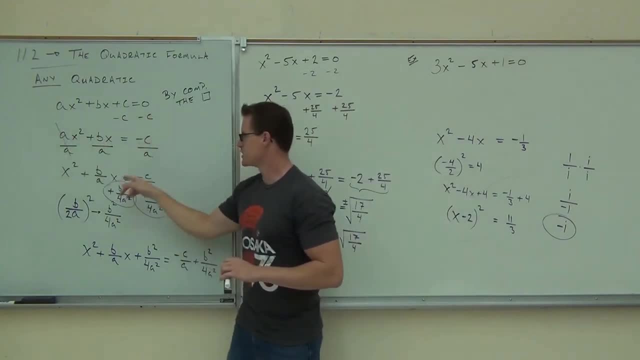 So, got rid of the constant. Divided by this coefficient. Taking this middle term, just like this one. Divided it by 2. That means you just have another 2 on the denominator. Squared it. 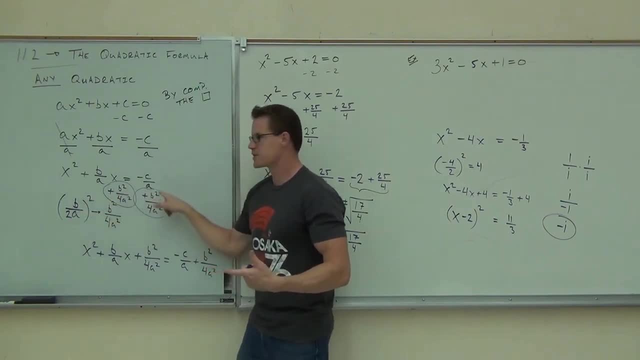 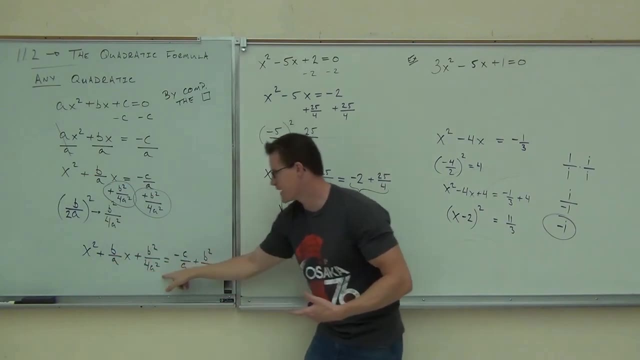 That means you're going to get b squared over 4a squared. Added it to both sides. That's the idea. We've added that to both sides. Here we have x squared, plus b over ax, plus b squared over 4a squared. Bang it. We got negative c over a, plus b squared over 4a squared. Got it. 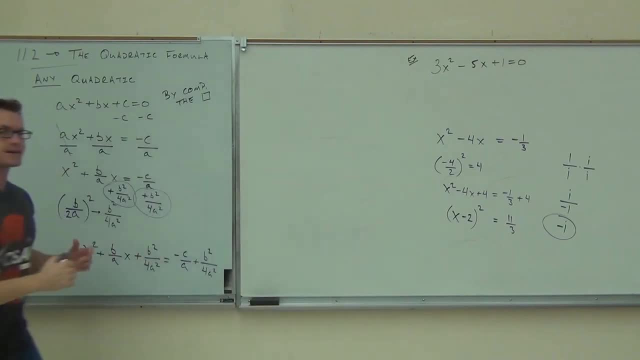 The next step is, I'm going to leave this alone for a second. 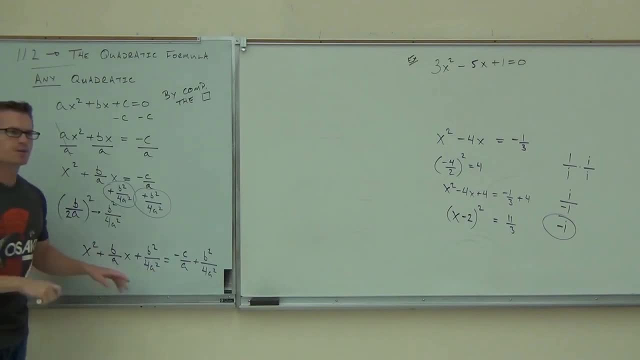 I'm just going to work on this left-hand side for one step. I'm going to factor it. Now, according to this, how we factor this thing, 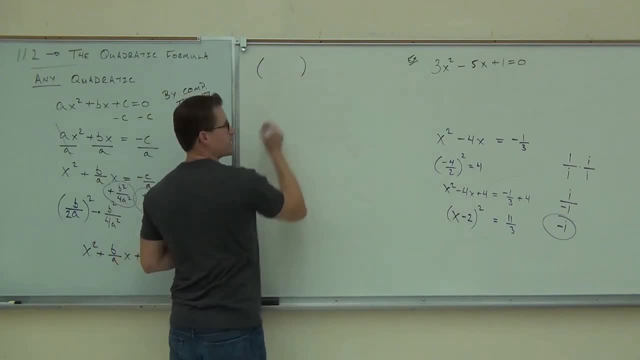 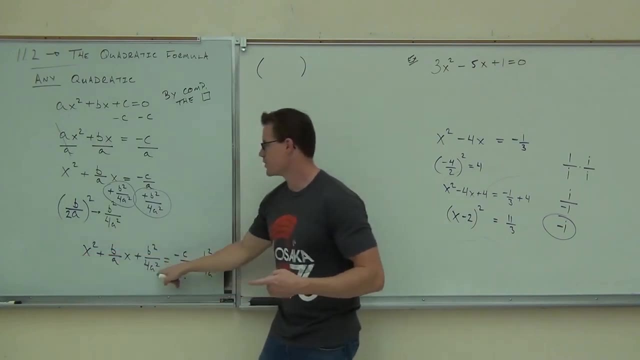 if you try to do a diamond problem on this one, you're crazy. All right? You can't do that. You have to know what a perfect square trinomial is. This is a perfect square trinomial. What it is, is x plus that middle term, divided by 2. That's the perfect square trinomial. That's the perfect square trinomial. Divided by 2. 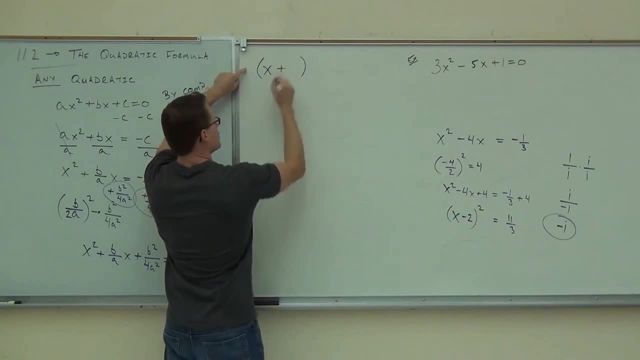 So, in our case, we're going to have x plus, what's going to go there? What do you, do you see it? It's on the board. 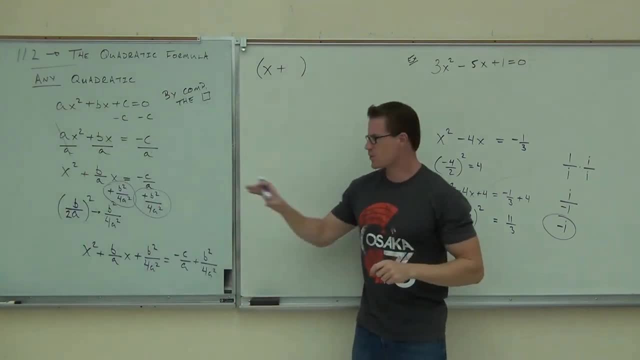 What's going to go, what's going to go right there? It's on the board right now. B over 2a. 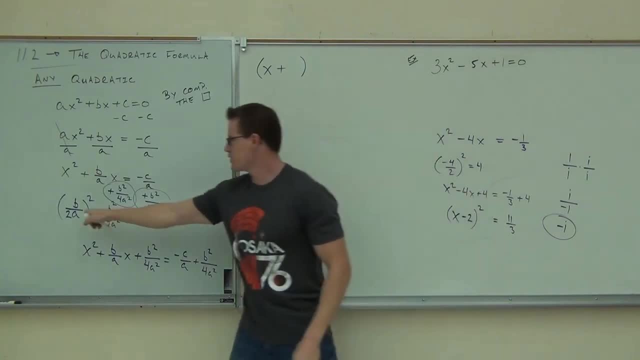 B over 2a. Do you see why b over 2a is going to go there? It's whatever you get before you square it. 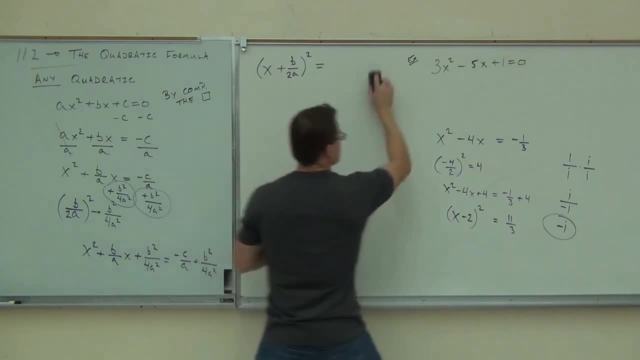 On the right-hand side, yes, it looks a little nasty. I'm going to work on that in just a bit. 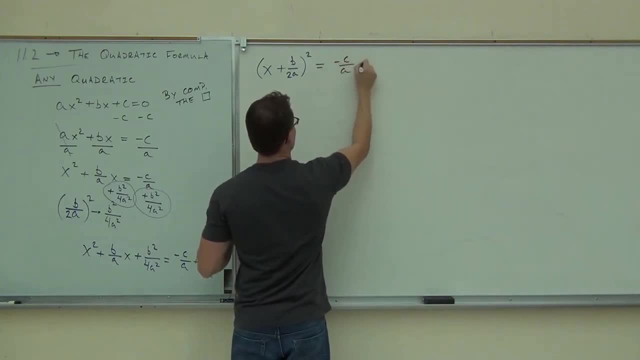 On the right-hand side, I have negative c over a, plus b squared, over 4a squared. Raise your hand if you feel okay getting down that far. Good deal. All right. Let's work on the right-hand side, because right now, that thing is just ugly. 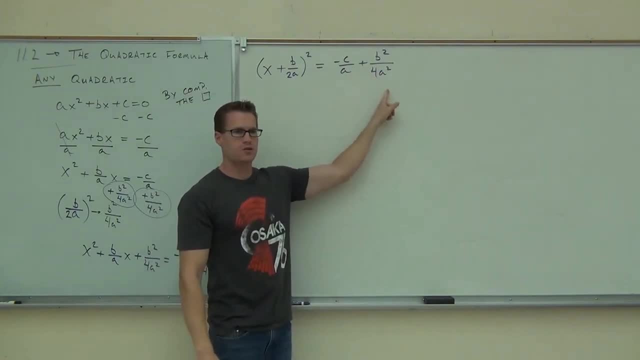 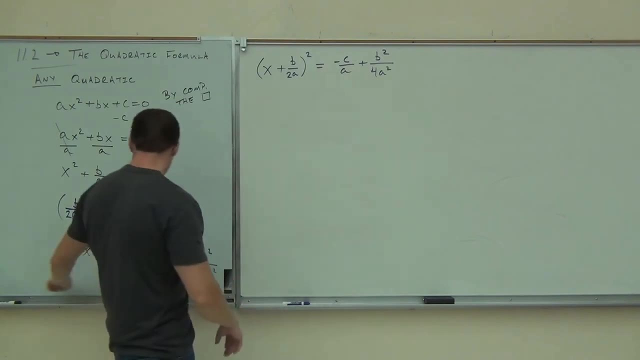 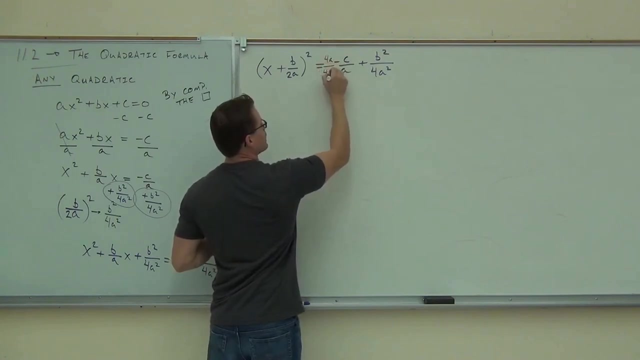 How do you combine two fractions? Common denominator. Now, fortunately, in chapter 7, you learned how to find a common denominator with this. Our LCD here would be 4a squared. Do you see that? So, what I'm going to do to find a common denominator, to get our common denominator, I'm going to multiply this by 4a over 4a. Do you see why? Left-hand side, I'm going to keep that the same for just a while. Right-hand side, I get notice. I still have a negative. 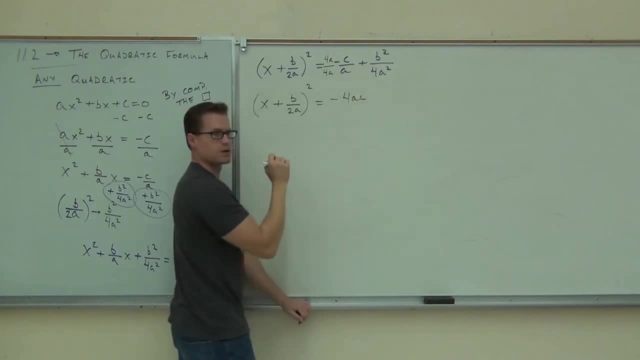 I've got negative 4ac. Do you see where the negative 4ac is coming from? 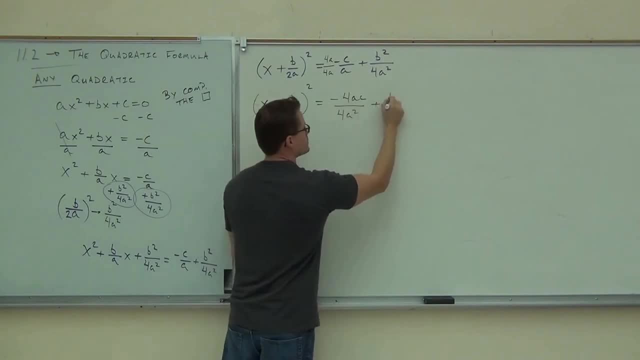 All over 4a squared, plus b squared, over 4a squared. Am I successful? Do I? Well, I know I'm successful. Do I have a common denominator is what I'm asking. Yes. Yeah, I do. I can make that into one fraction. 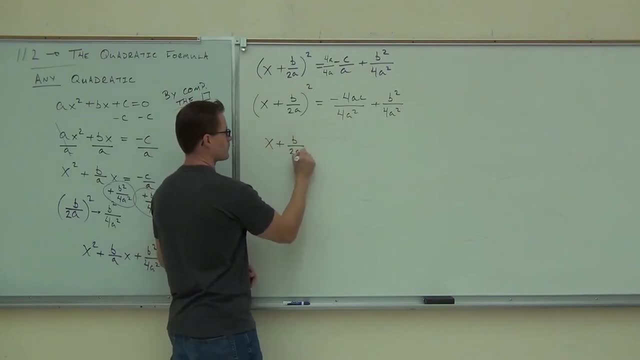 Now, when I do it, I know that my denominator is going to be 4a squared. True? 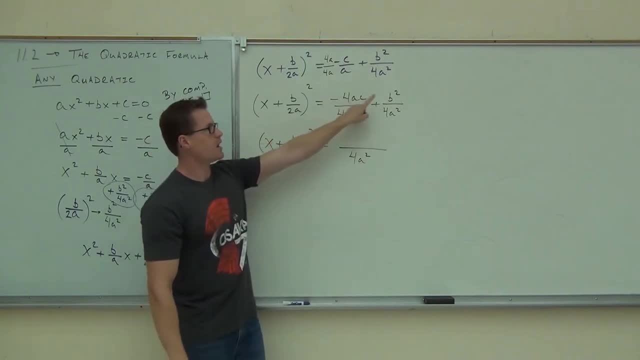 On my numerator, I've got negative 4ac. I've got plus b squared. Are you with me? But I'm going to write it differently. Watch the board carefully. 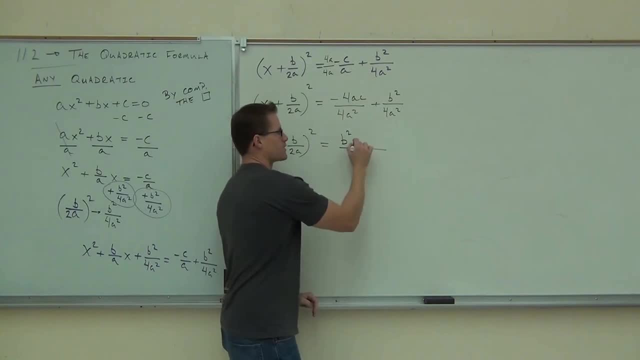 I'm going to write the b squared first. I'm going to write the minus 4ac second. Is that okay with you? Are you sure? 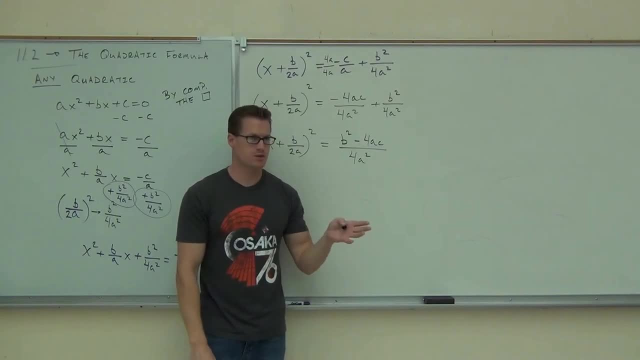 So, b squared first minus 4ac. Remember, you don't have to write this down. You're never going to have to do this in my class. If you want to follow, great. 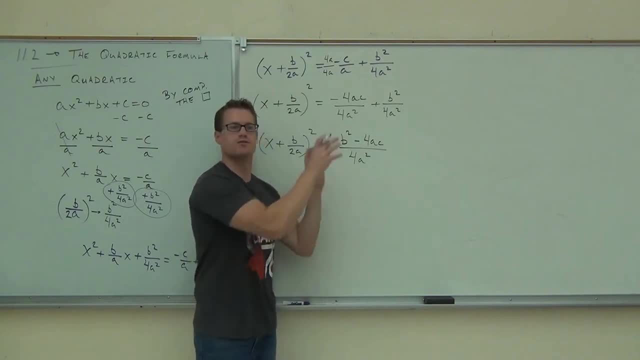 Write it down if you'd like to to look at it later. That would be fantastic. But I really do need you following here and being with me, okay? That's more important. Are you okay getting down that far? 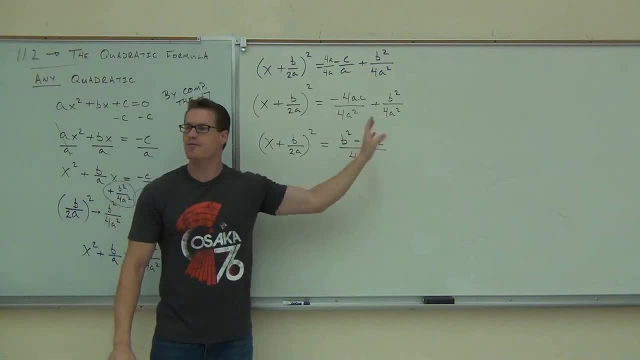 Right now, we're good enough to take the square root of both sides. We have this the way we want it. This right here, by the way, that little piece is called the discriminant. Can you say discriminant? Discriminate. Not discriminate. Okay, we're not discriminating. This is discriminant. 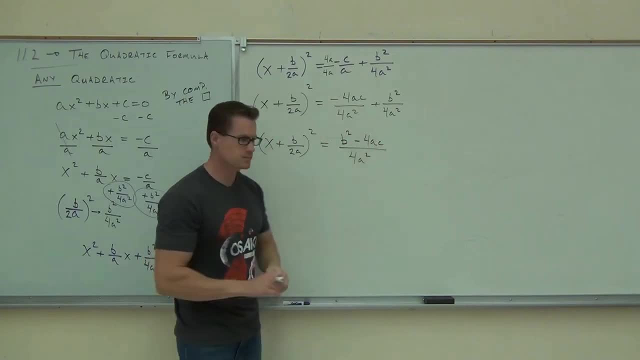 What it's going to tell you is how many solutions you're going to get and what type they are. It's kind of cool, isn't it? 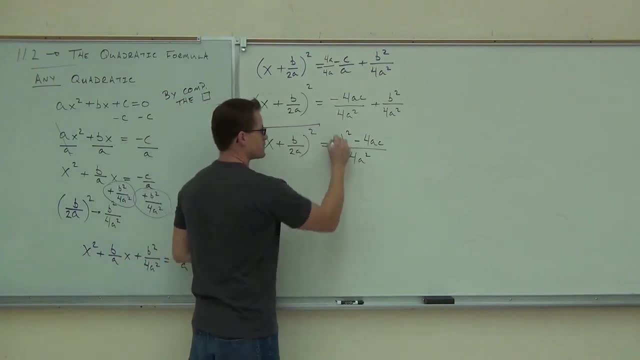 So, we're good enough right now to take the square root of both sides. Of course, when you take the square root of both sides, what must you have? Hey, you're going to have two solutions here just like before. 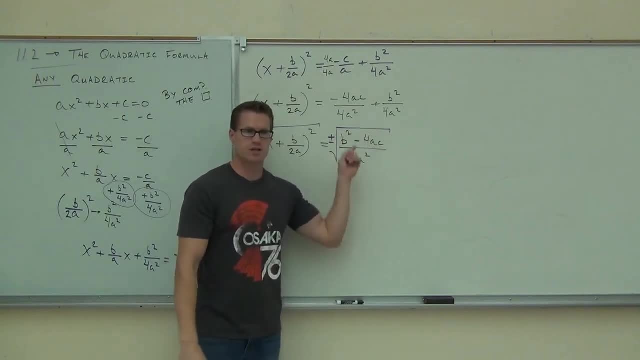 You're going to have a question. You're going to have a plus and minus. Now, I know this doesn't look that great, but you're going to see it in a minute. We're going to be able to work with it. On the left-hand side, what happens with the square and the square root? 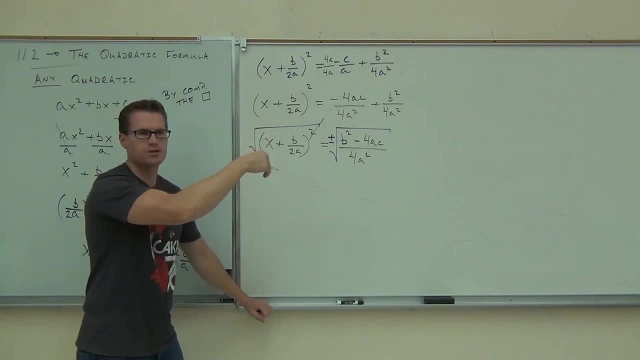 Gone. Notice how we're using like everything we've learned in this class, up to this point pretty much, everything we've learned besides like absolute value and inequalities to get to here, all the algebra. 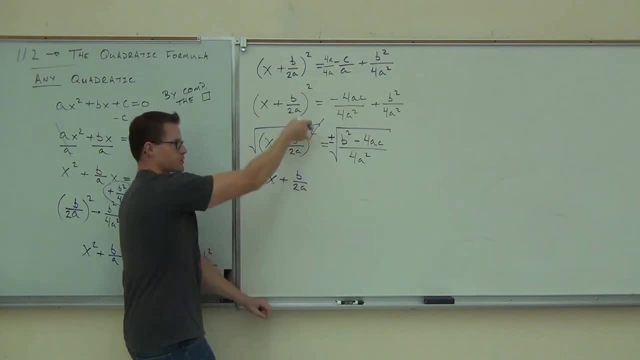 X plus B over 2A, those are gone. 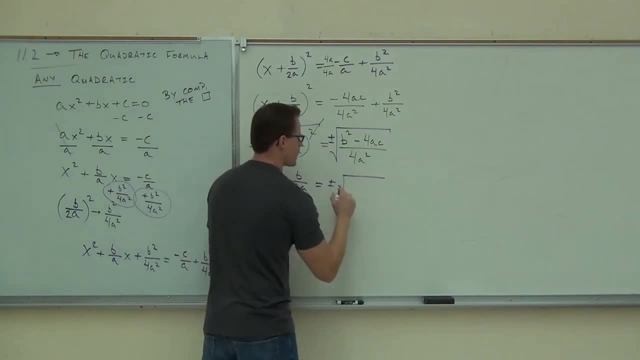 On the right-hand side, I have plus or minus the square root B squared minus 4AC all divided by 2A. 4A squared. So far, so good? 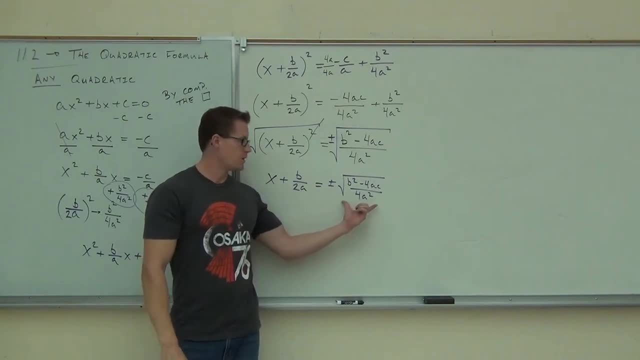 Now, you're going to see something that we've done before just a little bit earlier. Right here on this side, I'm going to split this up as the square root of the numerator over the square root of the denominator. We've actually done that already today. I'm going to show that step to you too. 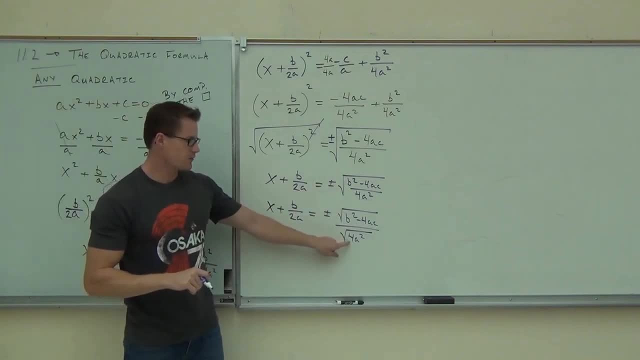 So I'm just splitting this up. What's the square root of 4A squared? How much is the square root of 4A squared? How much? 2A. Hey, we've done that in this class, right? Cool. 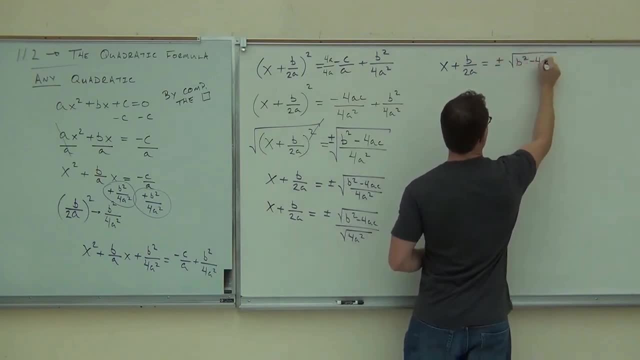 Plus or minus the square root B squared minus 4AC divided by 2A. Where did the square root go? You did it. Right there. 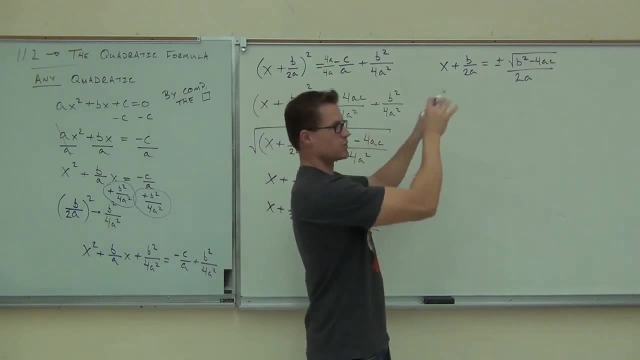 2A squared, 4A squared gives you, when you take the square root, 2A. You know what? There's only two more steps. 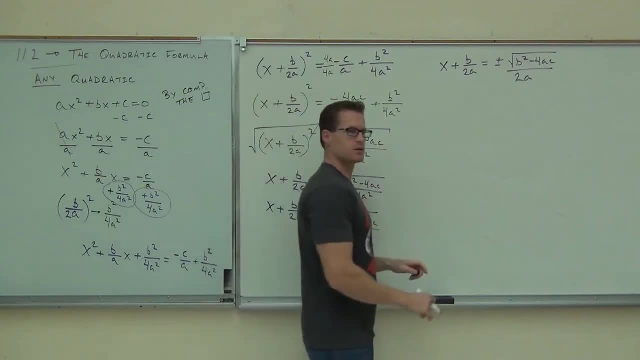 First step, solve for X. How am I going to solve that for X? Direct the B over 2A. 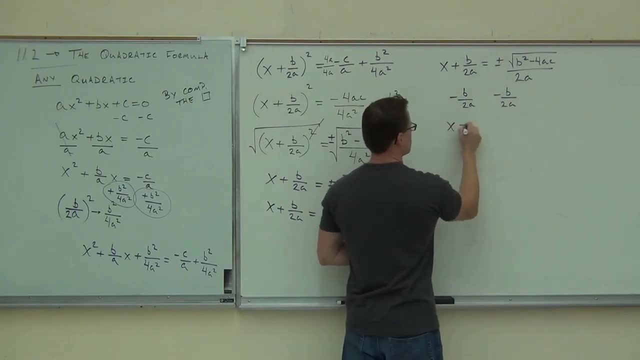 Of course, you mean by both sides. Of course. 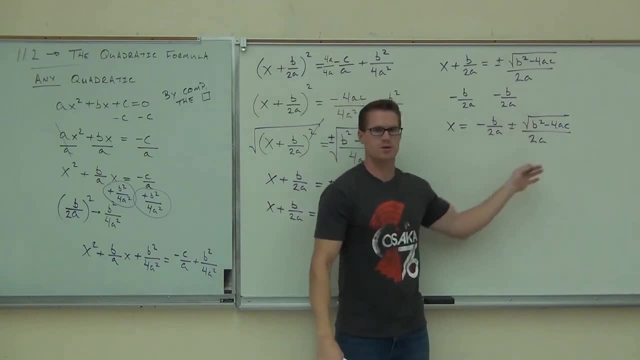 I know this, we haven't had this on the board, but does this look familiar? Compared to one of the problems we just completed? Yeah. 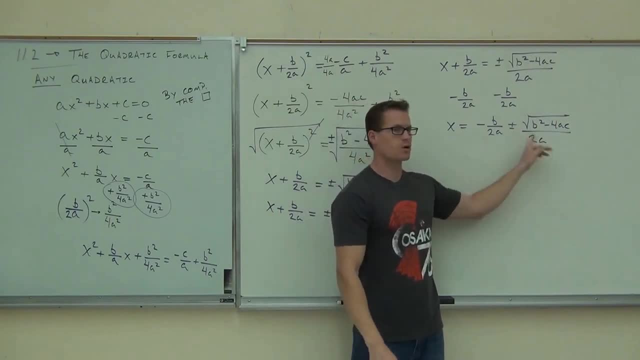 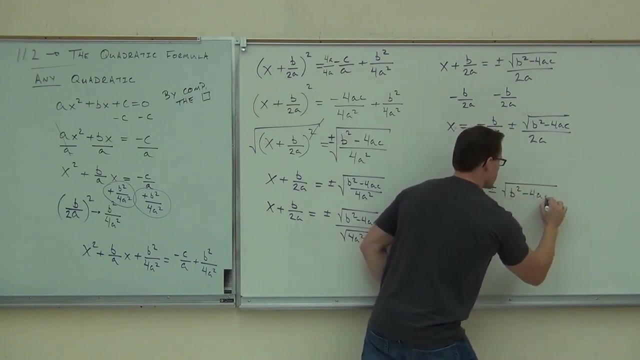 Kind of cool, right? We actually have a common denominator already. We're going to put this together as one fraction. When you put it together as one fraction, what you're going to get is, notice that negative, I can associate that with the numerator. I'm going to do negative B. Plus or minus is going to stay on the top of my fraction just like it did before. The square root of B squared minus 4AC. All right. Cool. 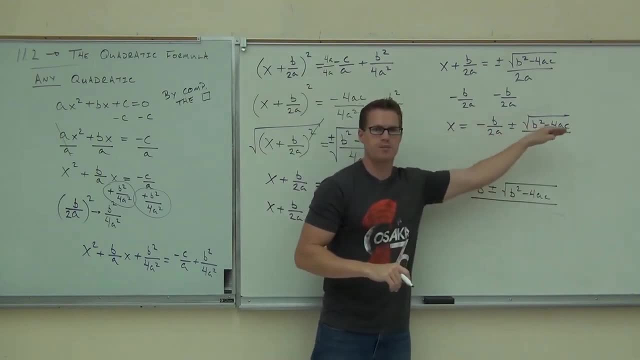 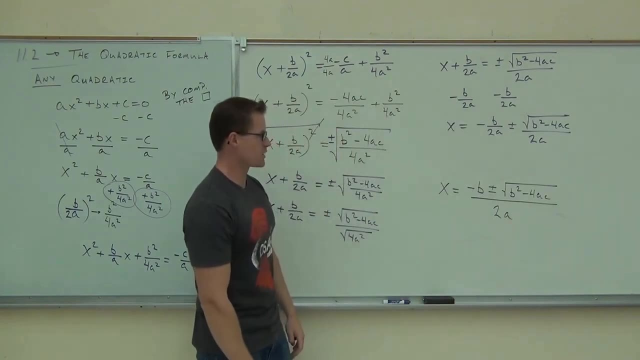 All divided by. Notice how this is a common denominator now. All divided by what's going to be on the bottom? 2A. Negative B plus or minus square root of B squared minus 4AC, all divided by 2A. 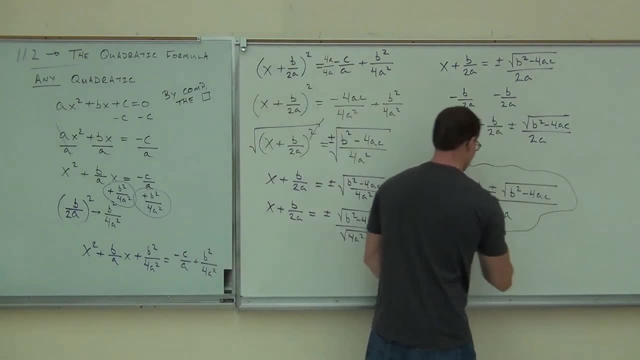 That's it. You said that almost easier. No, trust me. Trust me. This way is easier. I'll prove it to you in five seconds, yes. 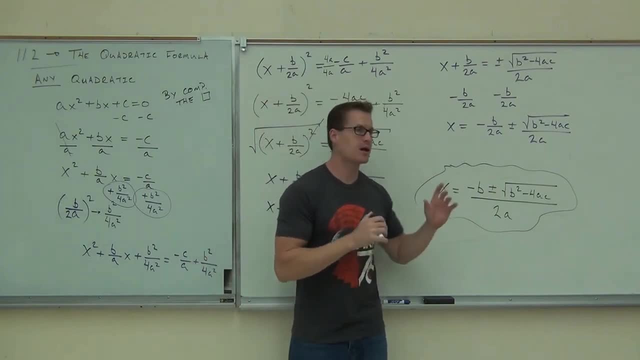 That B square, it stays in the square root? Yes. You cannot simplify that because it's connected with the subtraction. 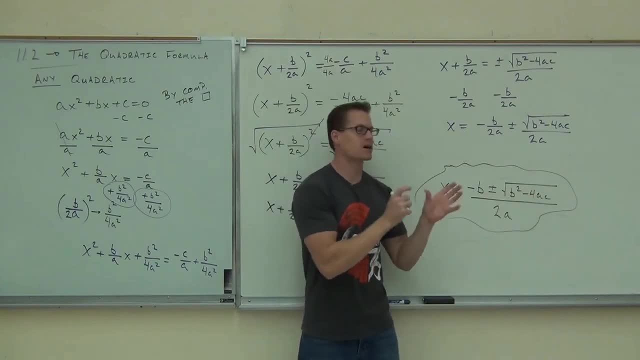 You can't split that up. That only works with multiplication if it's not connected by subtraction or addition. OK. 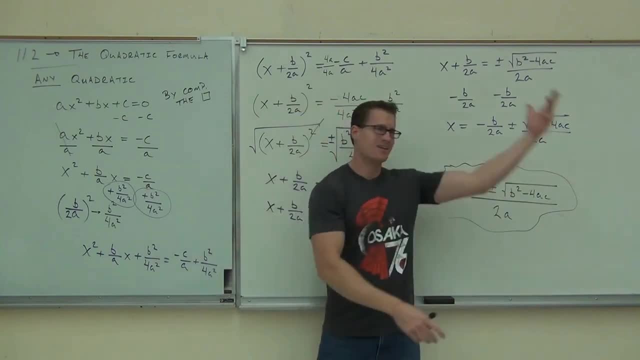 Now, why? Why am I struggling? Why? This sucks. Why? No, no, no, no, no. This doesn't suck. Trust me. 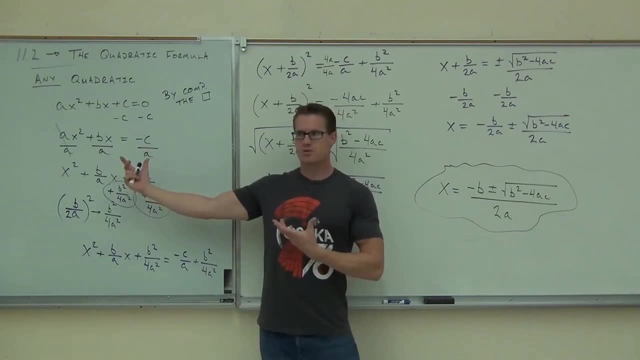 This right here completed the square, right? And it completed the square once and for all, which means you never have to do this again. 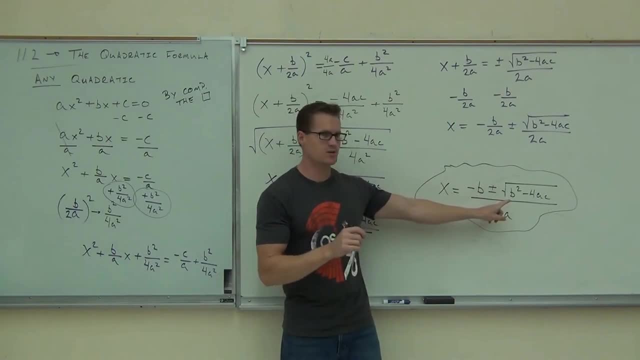 Which means that if you look at this, this is going to be very interesting to you. It will. Brainwash me right now. It will be interesting. 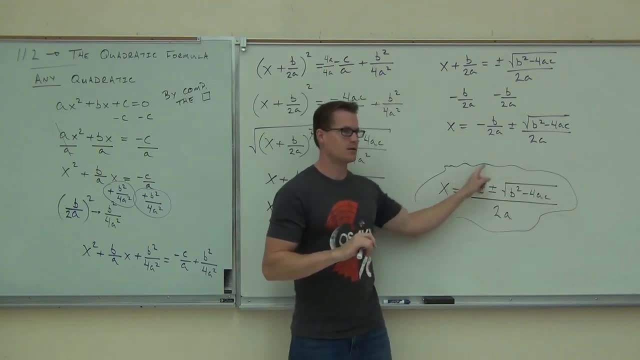 Does this have any x's in it? No. This just has coefficients. Notice A, B, and C are numbers. Right? Numbers. 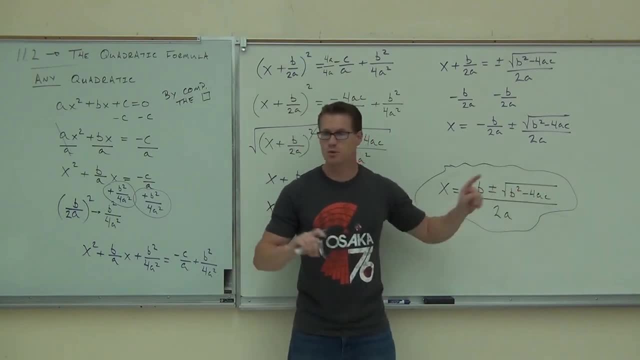 This means if you look here and you find your numbers and you plug them in, you automatically get your answer, x equals. That's your answer. 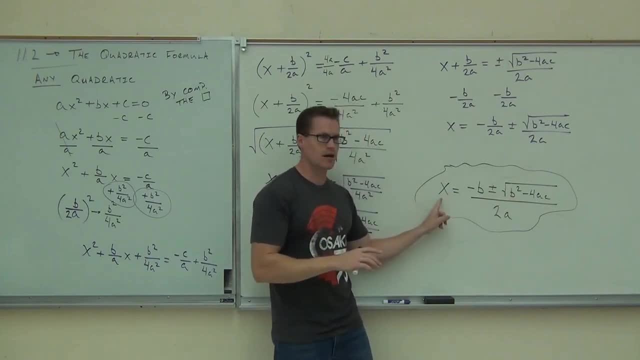 Is that awesome? Yes. No work. No work. Just plug in numbers. Now, I can tell you, even though this is right here, this is the formula. It's there. Oh, yeah. 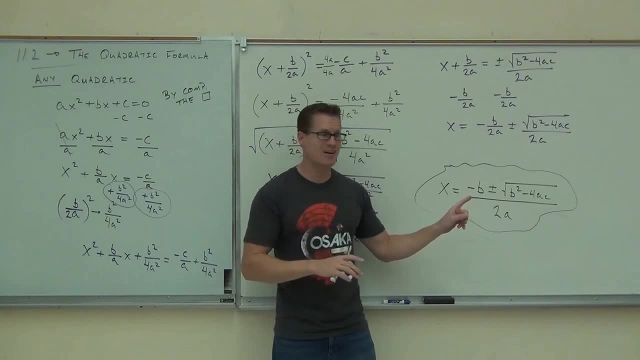 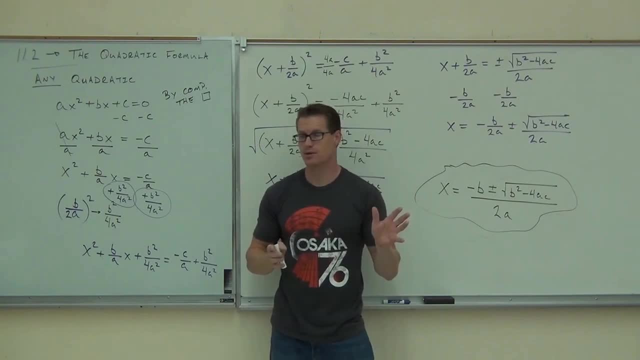 Alok, yeah, do. Alok, screw this thing up. You know why? You've got to memorize it. You do. You have to memorize it. I'm going to teach you how to do that in just a second. 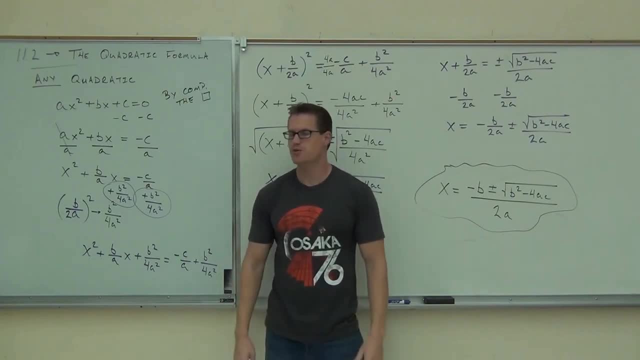 But also, the signs, positive and negative, your positive and negative signs kill you guys. They murder your problems. I see it all the time. 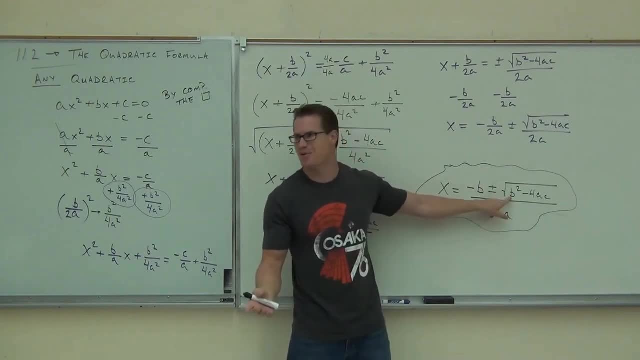 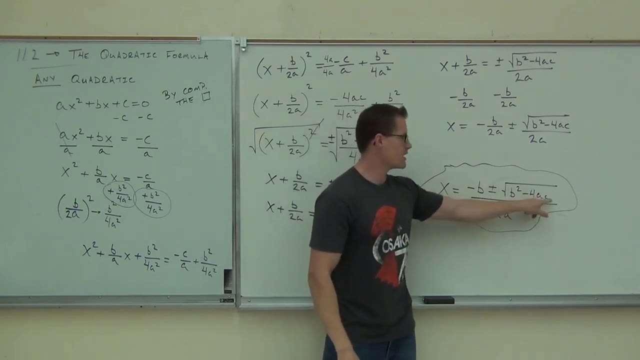 You've got to know that when you square something, you're not going to have a negative anymore, right? Even if the negative's in there, you square it, you're not going to have a negative anymore. This is b squared, in parentheses, minus 4ac. You're going to have negatives over here. You've got to know. 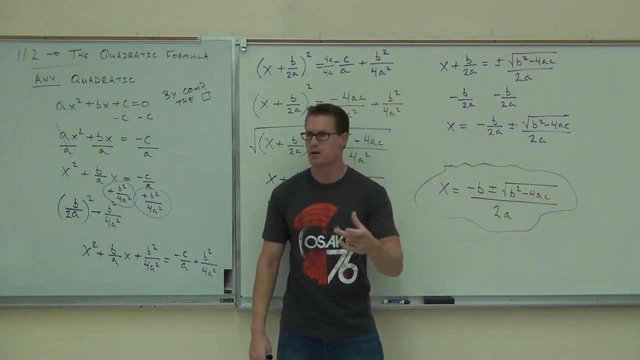 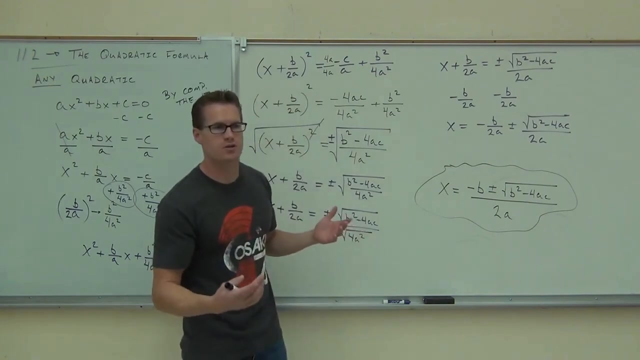 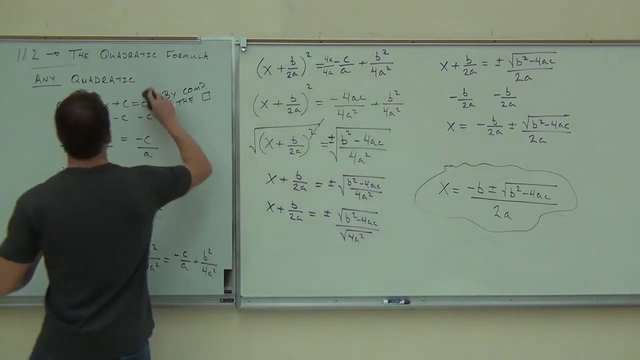 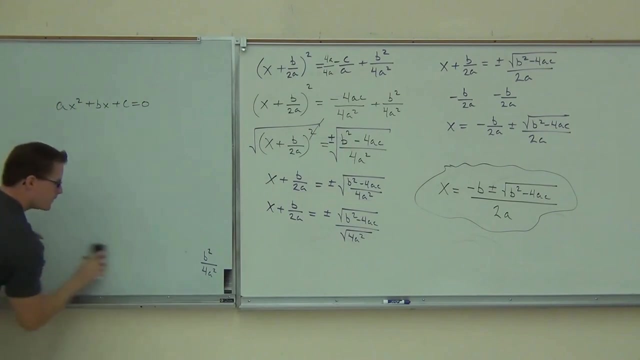 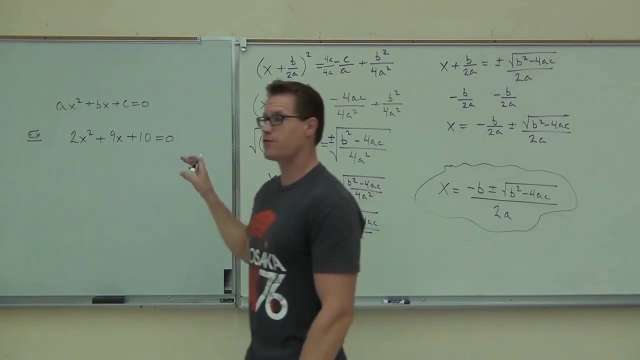 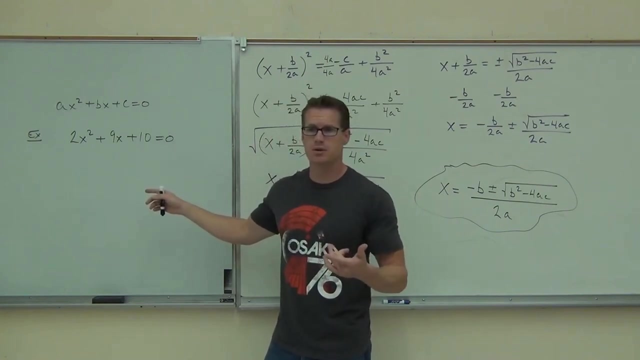 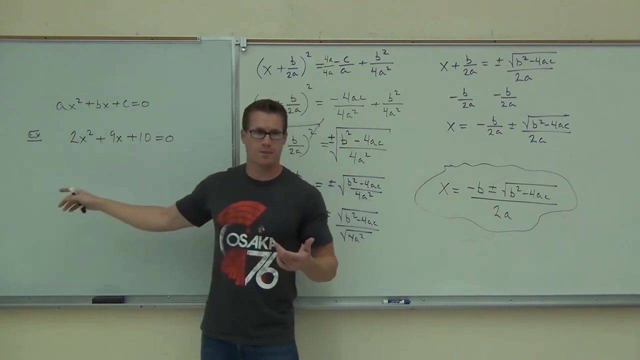 negative and you're subtracting it becomes a plus right when you have a negative and there's no negative over there or two negatives you're actually subtracting that you know that the a here is a number you have to multiply that thing negative negative that could change it into a positive right there so you have to watch your signs very carefully that's the only thing that can really happen let's do one example I'll give you a way to memorize this formula so I'm going to leave the quadratic formula on the board over there we're going to identify that any of these problems can be solved with that for example 2x squared plus 9x plus 10 equals 0 all you need to be able to do is use the quadratic formula find your a B and C now first thing could you do this with factoring I don't know maybe maybe you could but it has an extra step on it right that's not going to be that fun could you do this with completing the square absolutely every problem can be done by completing the square that works all the time however I'm going to tell you something if you can't factor it in less than 10 seconds and it has the number up front you're definitely not going to be completing the square if you can't factor it in 10 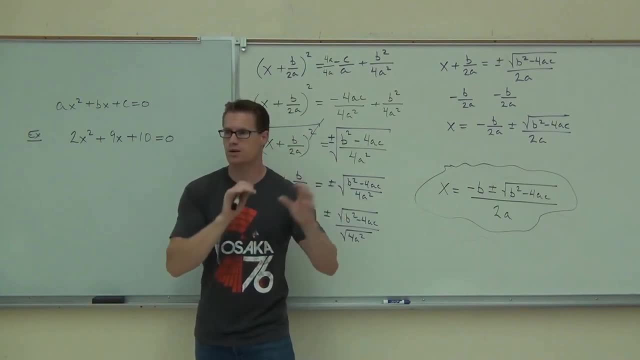 seconds you should have two options here factoring or quadratic formula if you can't factor it in 10 seconds can you factor it in 10 seconds 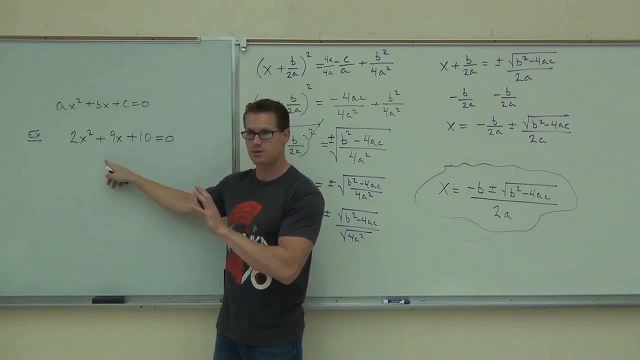 ready go 1 2 3 4 seriously think about it 5 6 7 8 9 10 have you factored it okay then skip it then go to quadratic formula I'm serious I'm serious if you cannot factor a problem in 10 seconds you're wasting too much time on it factoring should be 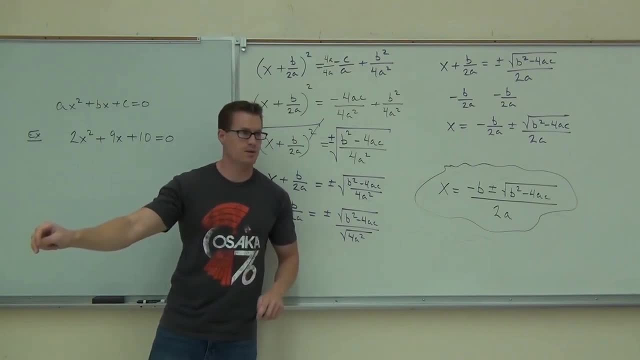 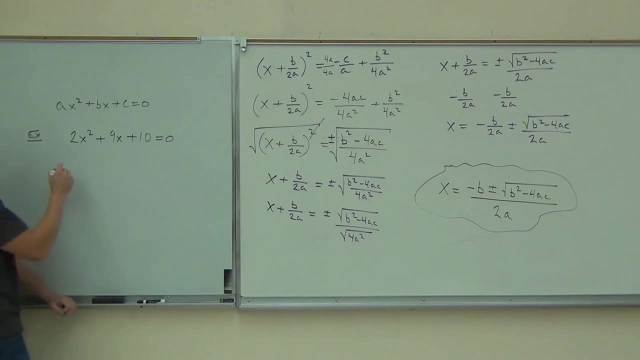 quick or you skip to something else that works faster you with me that's the idea don't use completing the square that way it takes way too long all I need to do to do is find your A, your B, your C, everybody, what's your A? Two. 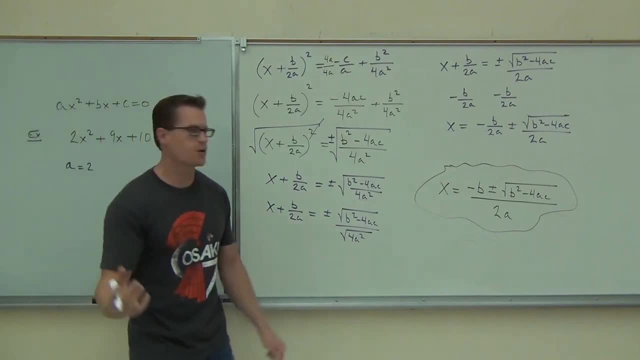 Two. Just the coefficient. This has no variables in it, folks. Are there any X's? No. Are there any X's? No. 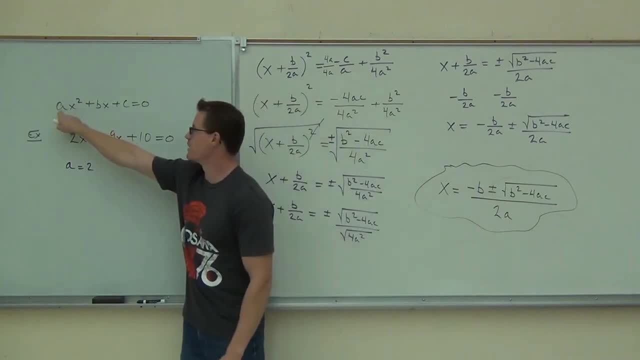 No. A, B, and C are the coefficients of your problem. A is the number, B is the number, and C is the number. What is your B? Nine. What is your C? Ten. 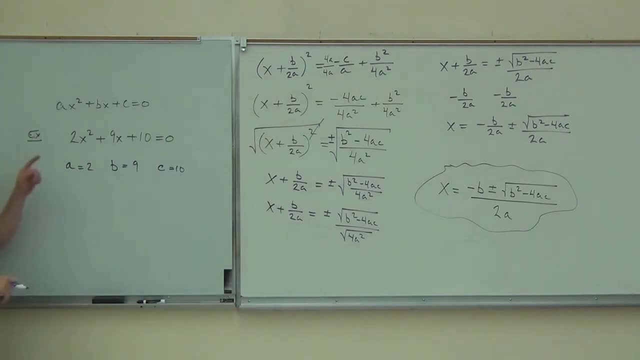 Make sure you got that one right, yep. We're going to take these numbers, plug them in there. Do you see your A, B's, and C's? 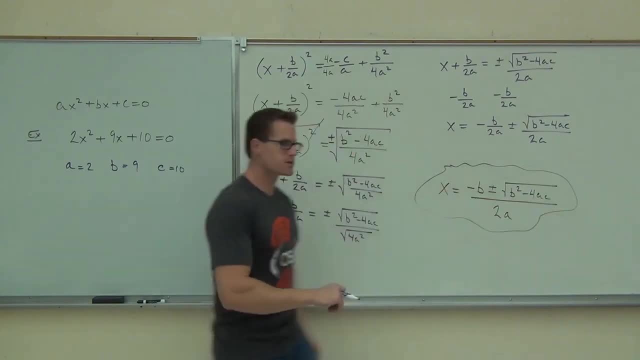 We know our A, B, C. We're going to take these numbers, plug them in for these letters. Let's see if we can do it. 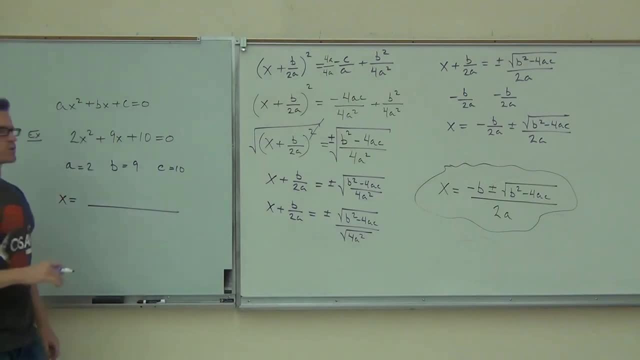 X equals negative B. What's negative B in this case? Nine. Then I have to have what, folks? A sinusoidal membrane. It is a formula. It does not change. 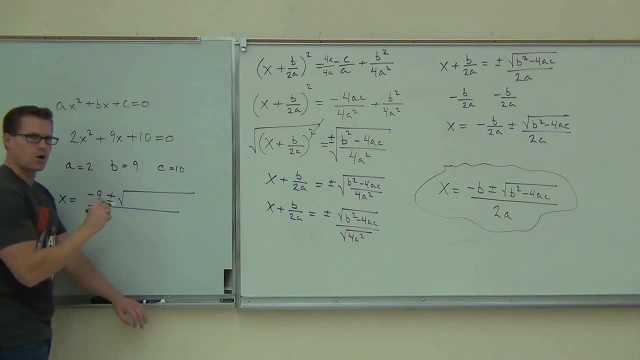 And then a square root. In the square root, you're going to put, and I want you all to do this just to make a habit of it, parentheses squared. That's going to be in parentheses. It means whatever you have, you're going to square it positive or negative. What goes inside the parentheses? Nine. Nine. B squared. B squared. 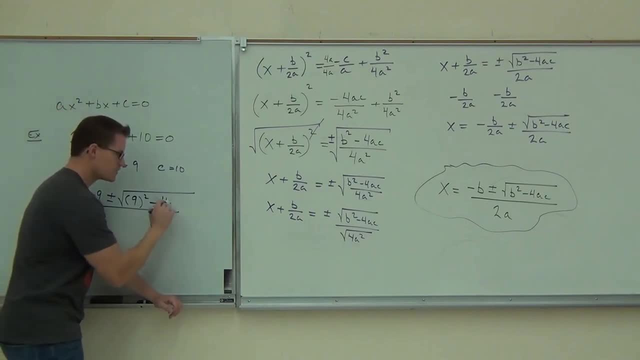 Minus four. Four doesn't change. Four AC means four times A times C. How much is your A here, ladies and gentlemen? Two A. Times C. What's C? Ten. All over two times what? Two. Two. Two times two. 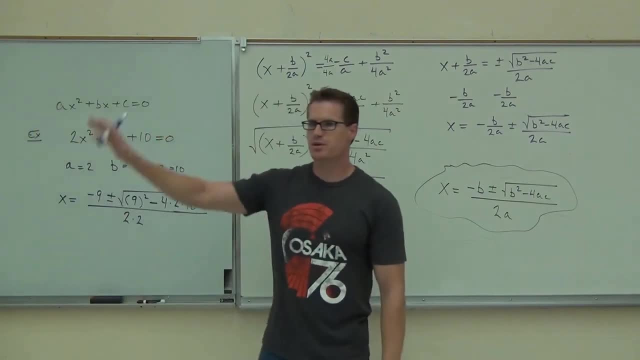 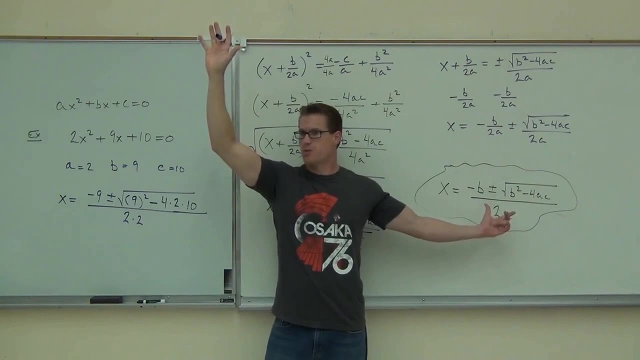 Raise your hand if you see where those problems come from. Keep your hand up if you understood where this formula is coming from. That's kind of important too, right? You know where it's coming from. It's in the square. So we know our A, B, and C. We can plug those things in. We'll work this thing out later. We'll work that thing out tomorrow. 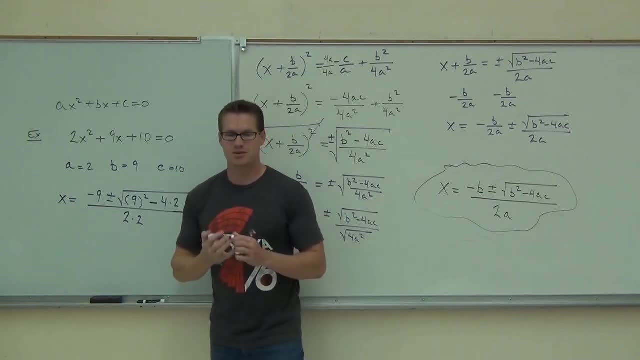 We'll do maybe three or four examples and we'll be done. Now, would you like to learn a song on how to complete this thing? Yeah. I'll do it, but you're going to do it. I'll do it, but you're going to do it. 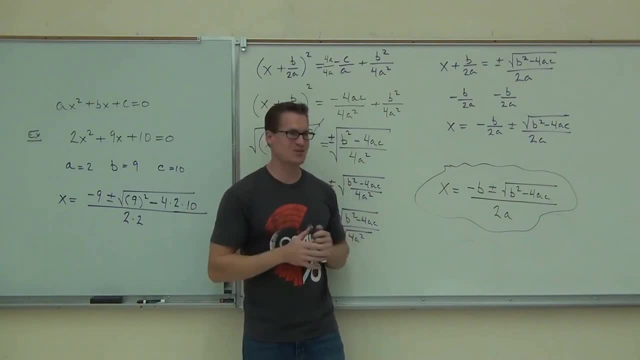 You're going to do it too. And if you don't, I'm going to turn the video and watch you as you do it. Here it is. Now, don't say you don't know lyrics because the lyrics are on the board. All right? This is it. 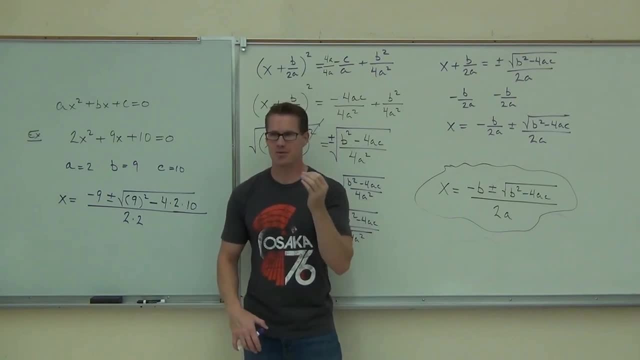 Here's how it goes. And you're going to hate me. You're going to hate me around Christmas time. 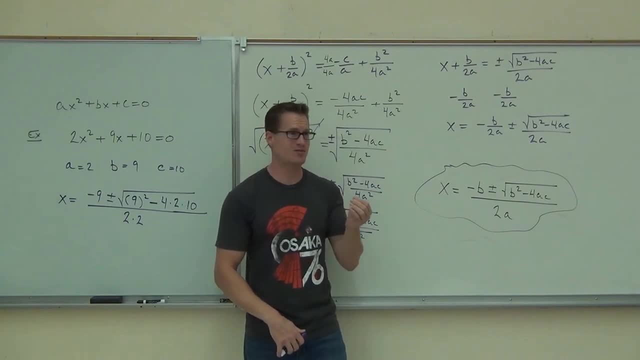 I promise you will because here's what. You never forget this. It's going to be in your head forever. Here's your lyrics. This is your pass out of class. If we do it good, we'll get to leave. If not, we'll be here all day. Ready? Here we go. It goes, I don't have the best voice, so don't laugh. You like that? I'll do it one more time and then you guys will come in. Ready? 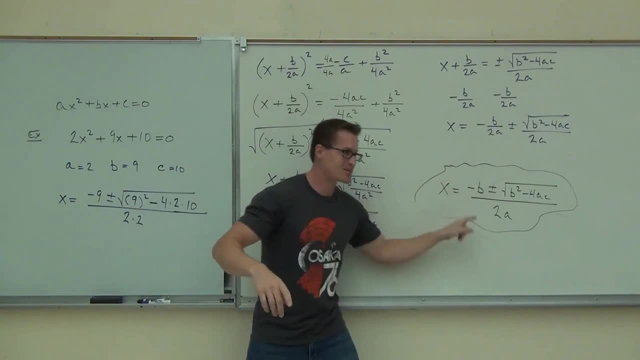 X equals minus B plus or minus radical B squared minus 4AC all divided by 2A. You like it? Now we'll do it together. Ready? One, two. Are you ready? Are you ready? The words are here. Let's try. One, two, three. 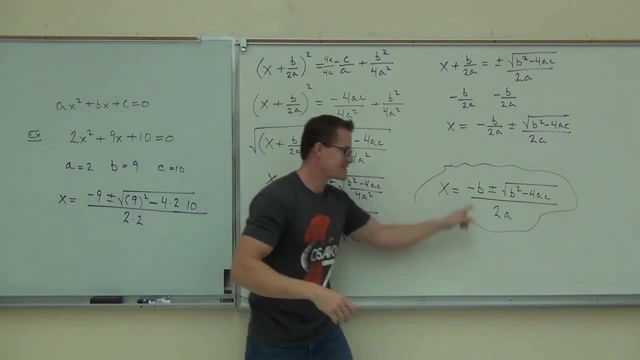 X equals minus B plus or minus radical B squared minus 4AC all divided by 2A. One more time on your own. I'll start you off. One more time. Ready? One, two. 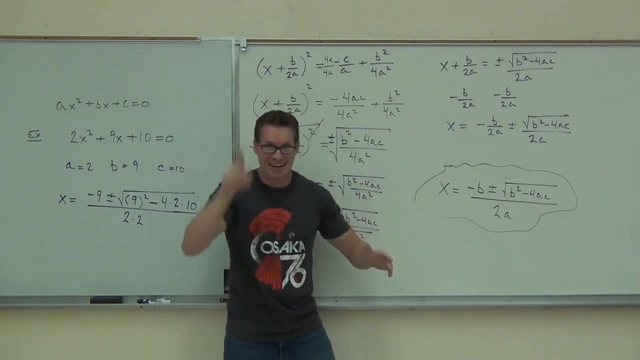 X equals minus B plus or minus radical B squared minus 4AC all divided by 2A. It's not 2A. 2A. 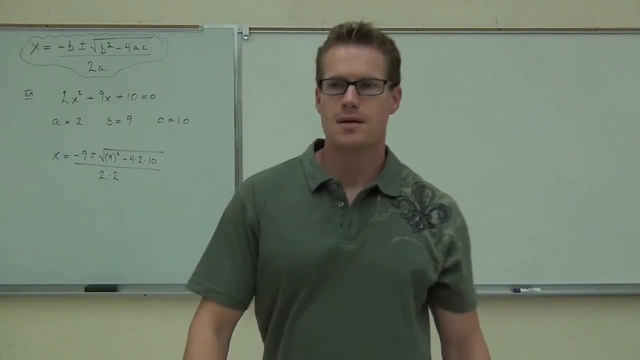 It's just OK. OK. All right. So, if you remember from last time, working with the quadratic formula. 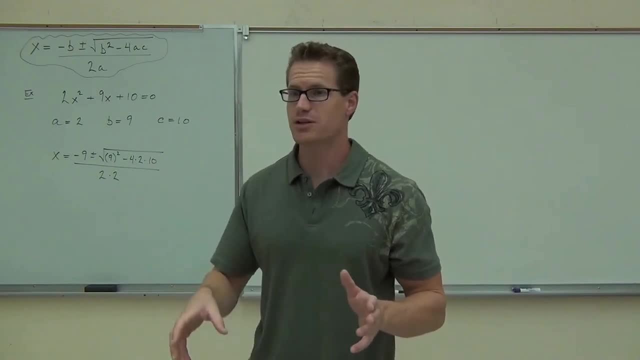 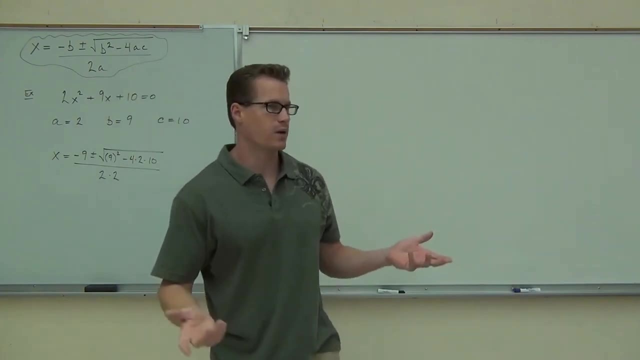 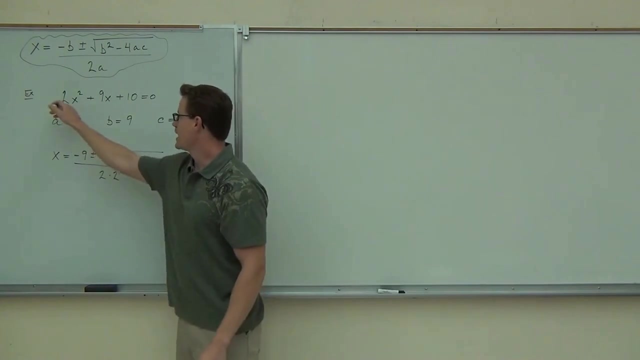 Last time we kind of invented this formula together. Hopefully, you remember how to do that. You don't need to do it yourself, but remember where this formula came from. This is basically, we completed the square once and for all on a general equation and that gave us this nice formula that has no Xs in it, just A, B, and C, which are the numbers that correspond with coefficients in any quadratic equation. So, when we do our problem, of course, the only thing you need to be able to do to get this right is to be able to do the first and last. is be able to identify A, B, and C when you are in standard form. 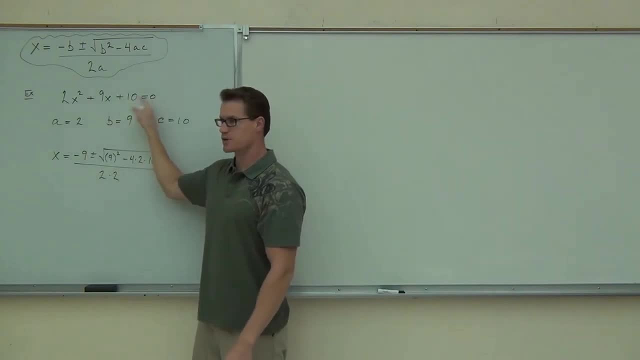 So notice, do you have to have zero on one side for this to work? Yes. Yes, you do. 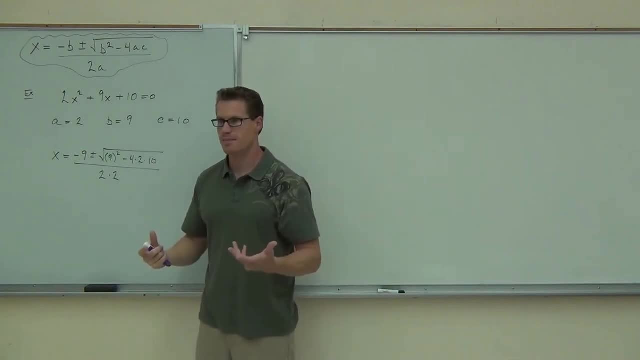 Otherwise, the signs for your A, B, and C will change. Do you see that? It's going to be negative over here. We don't want that. We want the correct signs for each of these. It has to be in the correct order, x squared, x number. The zero's got to be on one side. That's how you find your A, B, and C. Now, do you think you're okay with that? You sure? 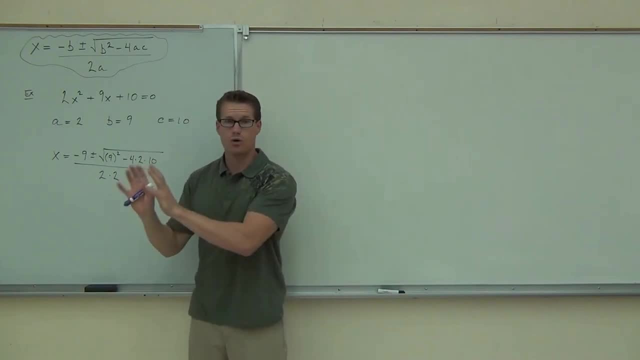 So just like most of the quadratics, we are going to get zero on one side and everything else on the other side. The only time we did not do that was with completing the square. That was a special case. Okay, you need to be focused up here, folks. All right, that's it. 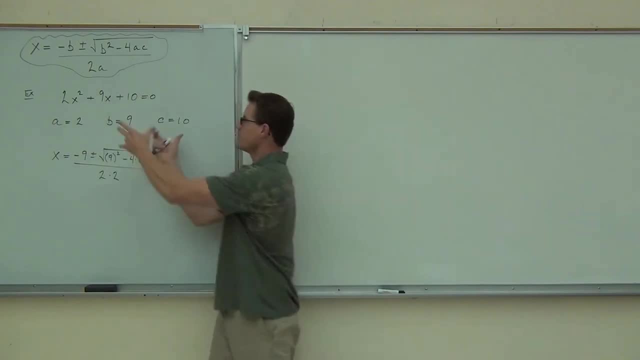 So we found our A is 2, our B is 9, our C is 10. If we take those numbers, we substitute them in that formula, and we get down to this far. I think that's where we stopped last time. Is that where we stopped last time? Let's continue because I told you, as long as everyone's going to be able to find A, B, and C, everybody. 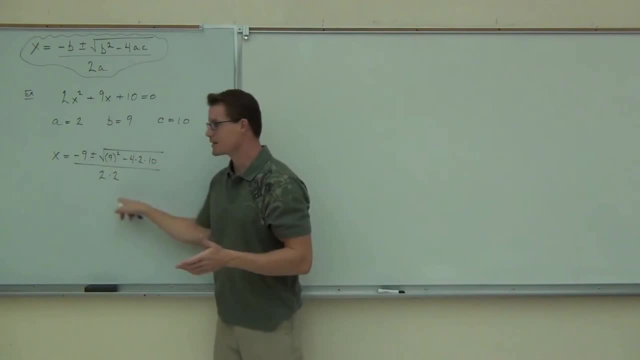 Everybody's going to be able to do that. Almost everybody's going to be able to plug them in here correctly unless you just completely forget the song I taught you or completely forget how to substitute numbers. 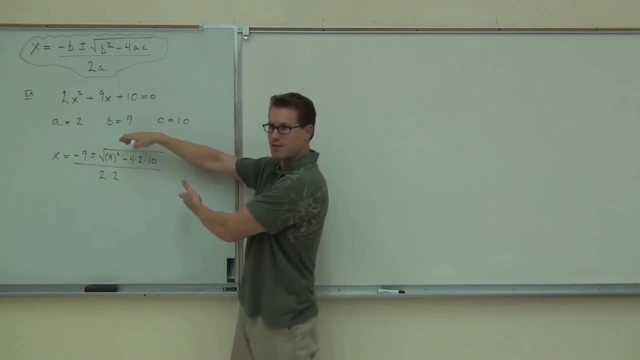 This is going to be right for 95% of you. For 95% of you, you're going to be just fine on this. 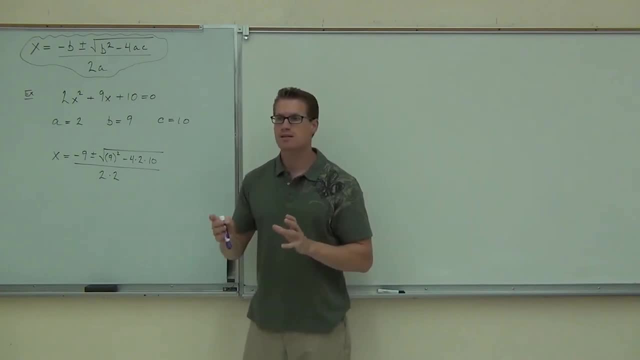 The problem happens when you start doing the actual mathematics. Science happens. Simple math errors happen. 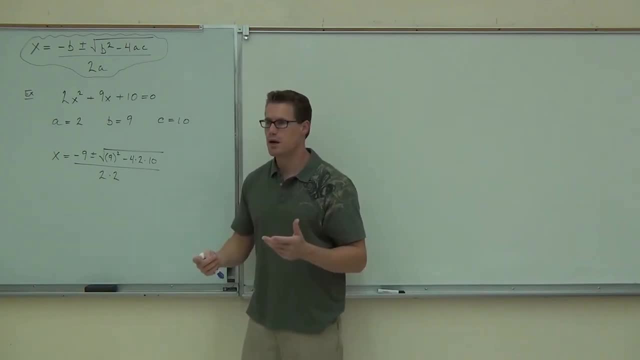 That's how this thing gets messed up. So we're going to go nice and slowly. You're not going to rush through this stuff. You're going to have plenty of time on your test. Don't rush it. Don't rush it. Go slowly. Use your calculator if you want to. I don't care what you use. 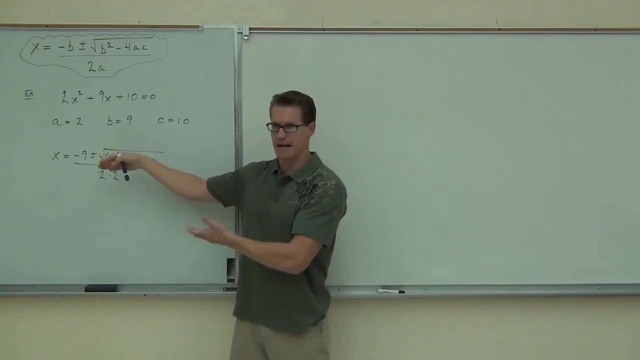 Just make sure your simple mathematics here is accurate. So we're going to go through. We know the negative 9. You're going to leave that. 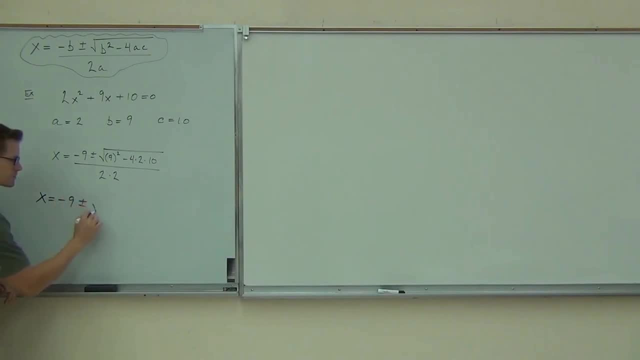 So we go x equals negative 9 plus or minus radical 9 squared. 18 or 81, which one? 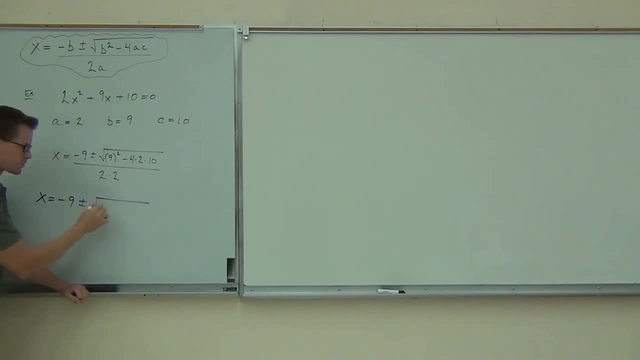 Notice that you're squaring this number. It will always be positive for this portion. If you get a negative number here, well, chances are you've probably done something. Actually, you've definitely done something wrong. If you get a negative after you square something, Now, this, yeah, that can't be negative. We're not squaring anything over here. This is minus how much is that? Eighty. 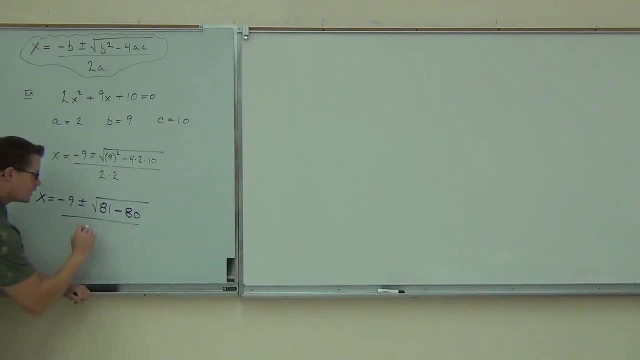 All over the square root of 2 times 2. I'm sorry, all over 2 times 2, which is 4. 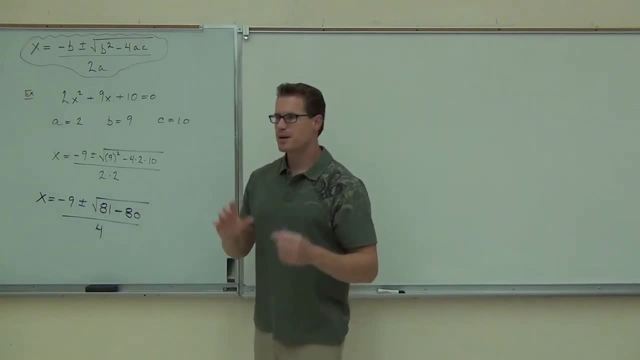 Still okay so far? So we're going step by step. 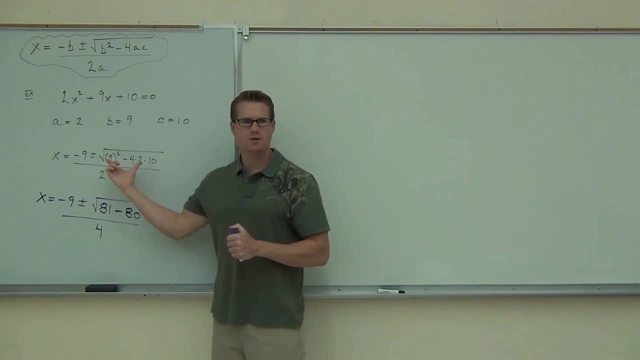 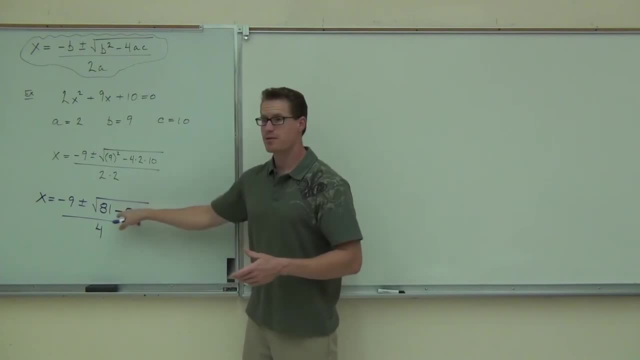 Sample five because I didn't say anything. Yeah, we could probably do that math, right? Those are going to be two numbers. 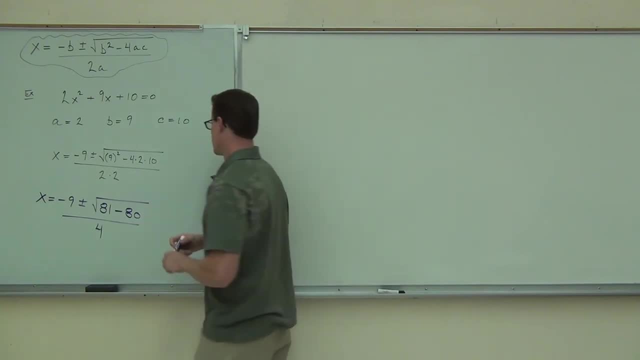 Eighty one minus 80 gives you one. Negative nine plus or minus radical. Don't skip out on these steps. It's important to get all these steps down. 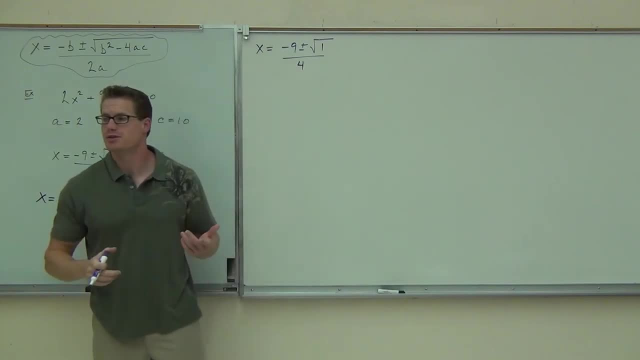 Over 4. We're going slowly. That way we don't make any math errors. 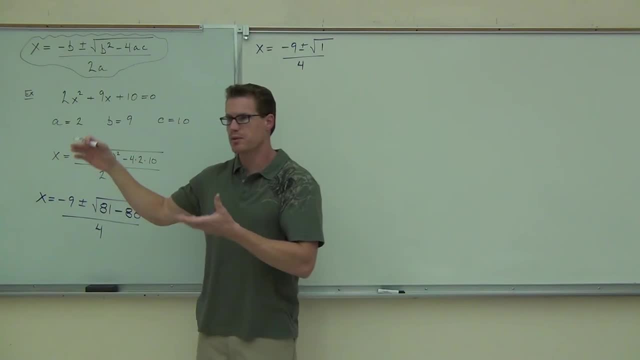 It's not a hard problem. It's simple math. I mean, you know how to square numbers, multiply, subtract, and divide. You know how to do that. Just make sure that you do it accurately. How much is the square root of 1? One. So don't leave it as the square root of 1. Oh my gosh. No, no, no. 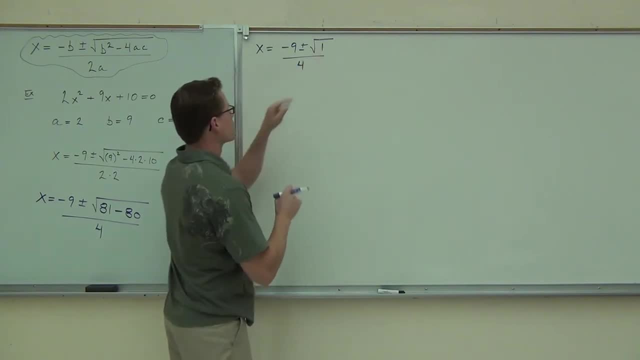 We're actually going to get two real nice numbers out of this. So the square root of 1 gives us x equals negative 9 plus or minus 1 over 4. 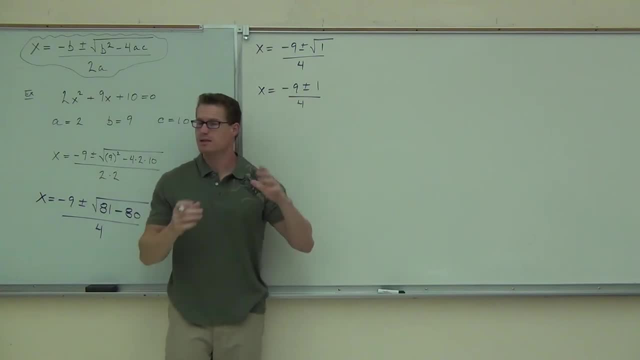 I'm not just doing this for your benefit, showing you all the steps. This is how I want to see it. I want to see each and every one of these steps. That's going to make you more accurate. 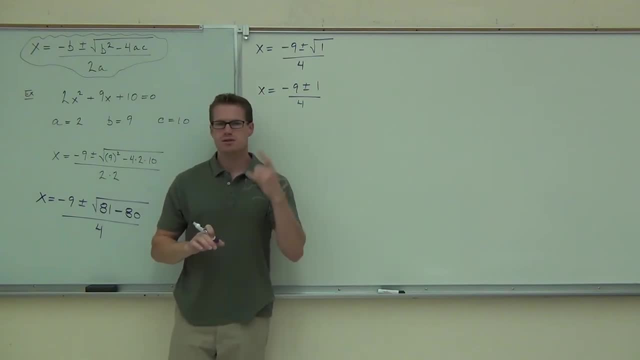 Hey, do I get two solutions? Yes. That plus and minus gives us two solutions. So we're going to get, follow the stream, upstream, downstream. 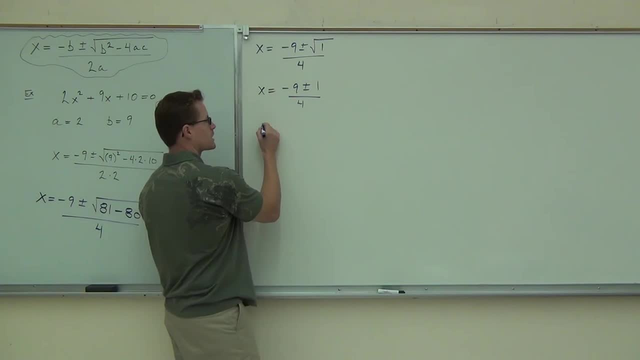 You're going to write out both of these before you do your math. So check it out. 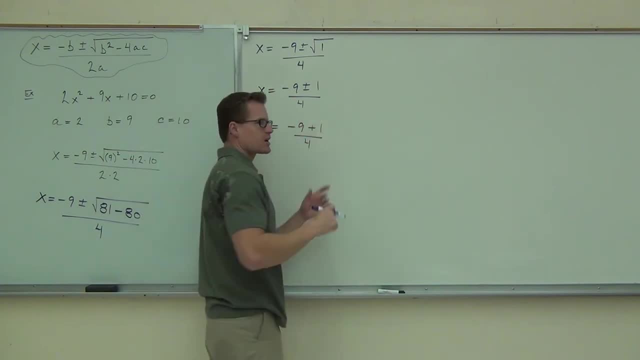 You get negative 9 plus 1 over 4, just like we did before, right? Plus 1. And we're going to get negative 9 minus 1 over 4. 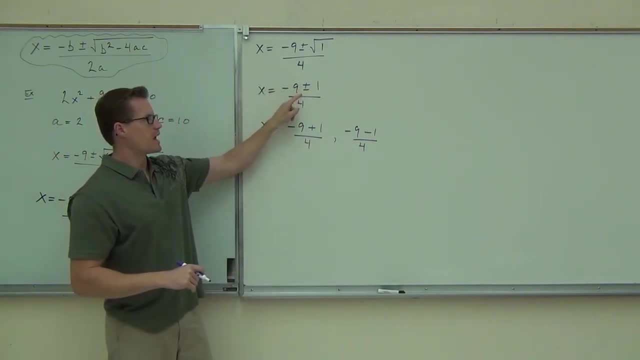 The negative 9, that one doesn't change. But we get the plus and we get the minus. Upstream, downstream. You guys are up to so far? 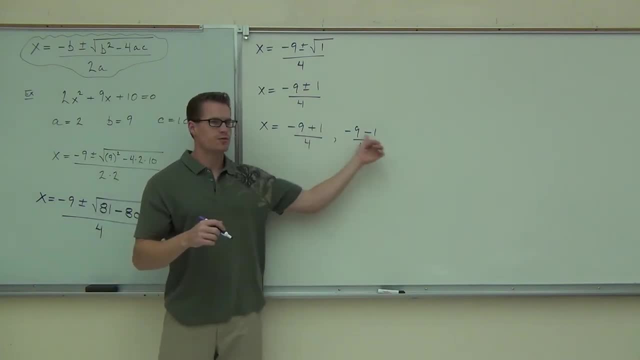 Hey, can you subtract and add this 1 from the negative 9? No. Can you do that problem? Yes. What's negative 9 plus 1? It's going to be an e. So don't hold back on that. You can do that. The only time you can't do that is if you have an i over here. 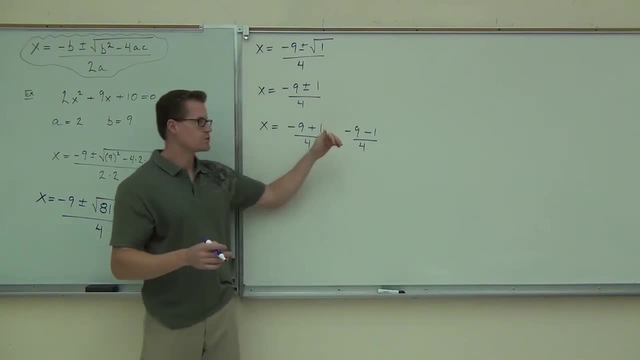 Or a square root, which is the same thing. So don't forget you know how to do this type of problem. 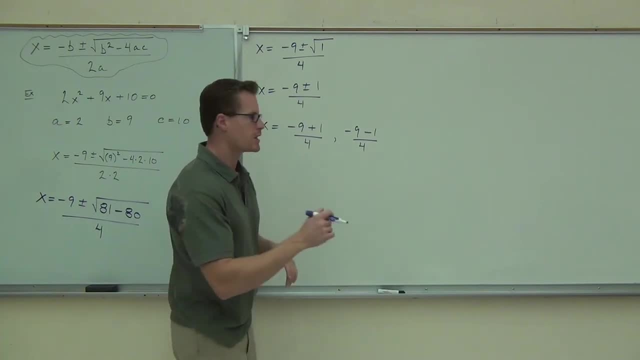 You guys need to be up on the board with me, not looking at other things, okay? 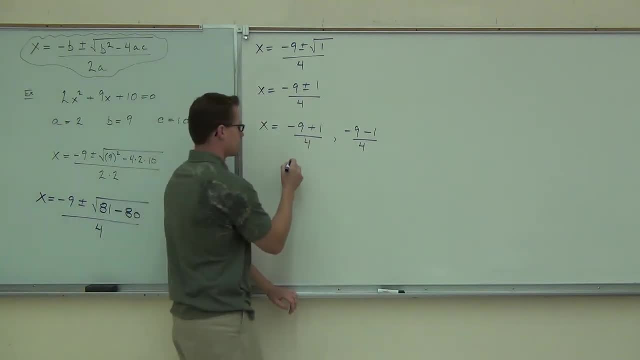 So negative 9 plus 1, how much is negative 9 plus 1? How much is negative 9 minus 1? 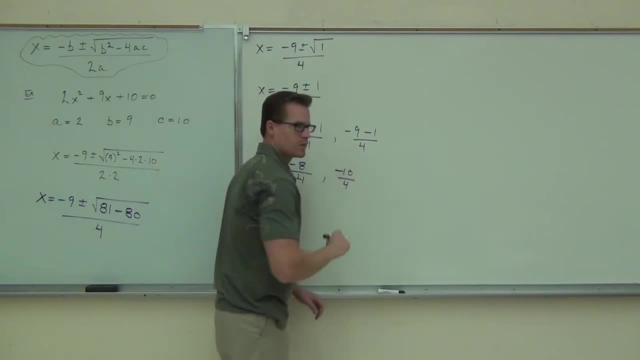 So don't make this harder than it is. This is not a hard thing. You're just doing simple mathematics here. 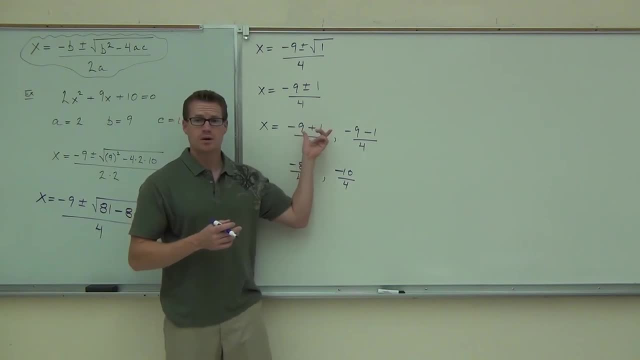 Just because this is a quadratic formula, it doesn't mean you can't add a number. It doesn't mean you can't subtract a number, okay? Don't stop there. Don't stop here. 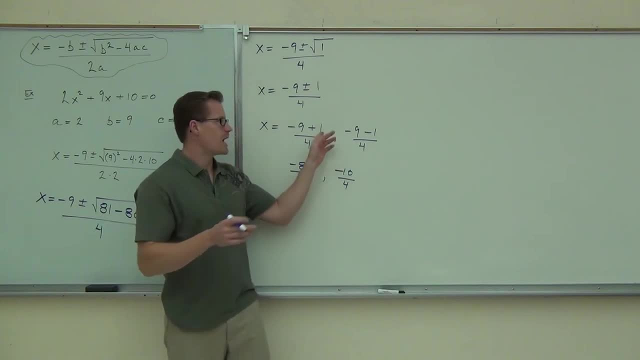 If you can put those together, then do it. If you can't, well, okay. If this happened to still be a square root, well, okay. 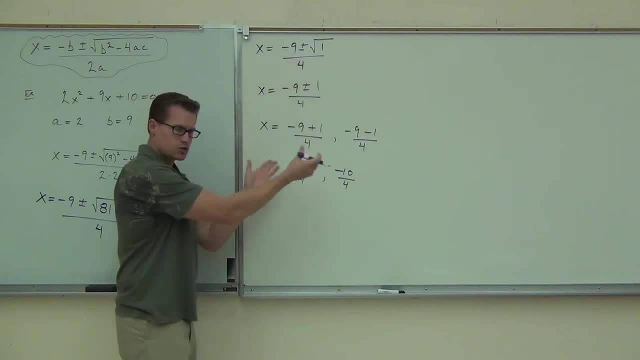 You can't do that. But if it's a whole number like we have, well, shoot, we can put those things together. We can get some real nice answers out of this. What's negative 8 over 4? Negative 2. 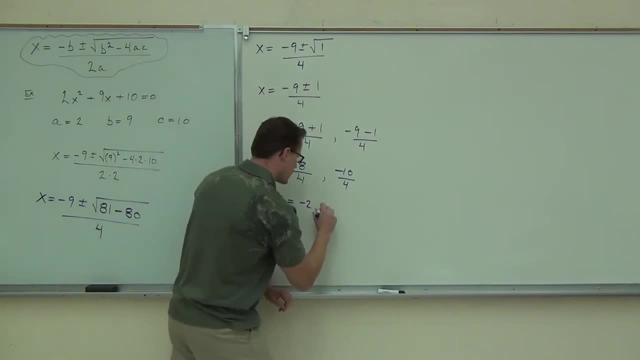 Can you reduce that? Yeah, negative 5 times 4. Negative 5 times, all right. Negative 5 times, all right. Would you raise your hand if you feel okay with this? 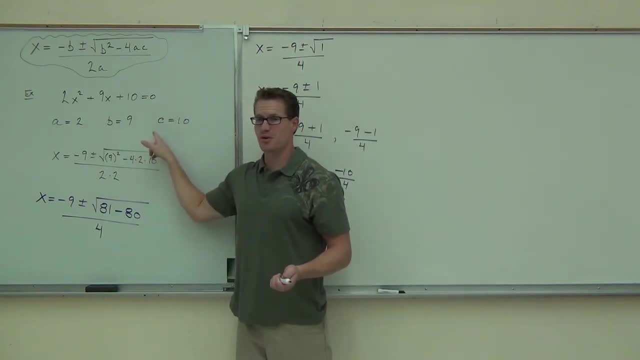 So what's the hardest part of it? Well, this is not the hardest part. That's probably the easiest part. Paying attention? Yeah. Plugging this in is probably an easy part. It's not hard. 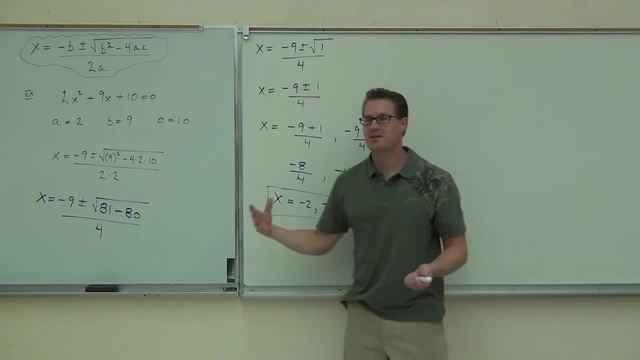 Doing the mathematics and getting all the way down to here, ironically, that's the hardest part. 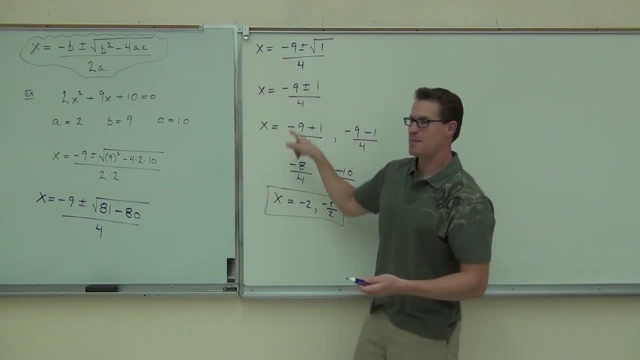 And to be honest with you, doing this stuff happens in Math 80. Happens in pre-algebra class. You do this stuff. You do the addition and subtraction. You do the multiplication and division. 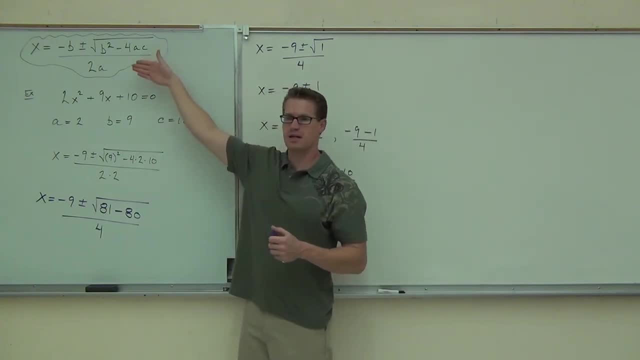 So basically, once we've done this, man, we've made this stuff a whole lot easier. This is easier than factory. It's easier than completing the square. It's looking at numbers and plugging in the formula. Are you guys all right with this? 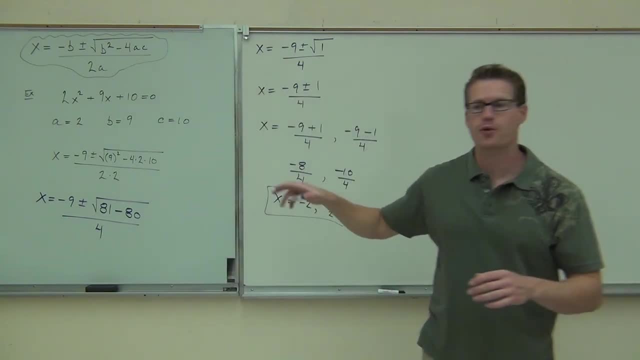 Now, what we're going to do today is try a couple more examples. I'll give you some different forms, different ways this can look, but we can still use our quadratic formula, okay? 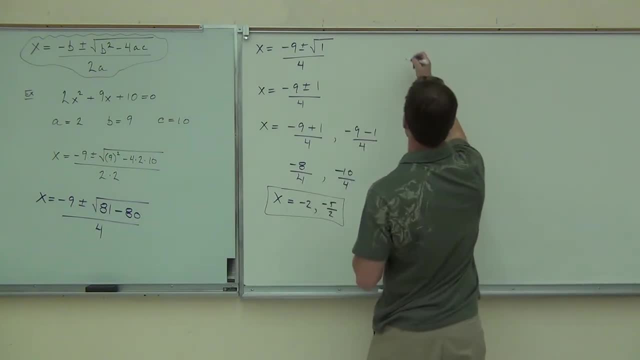 So next example, still kind of basic, basic here. 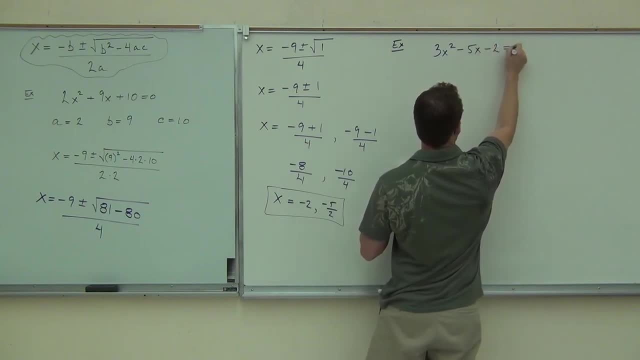 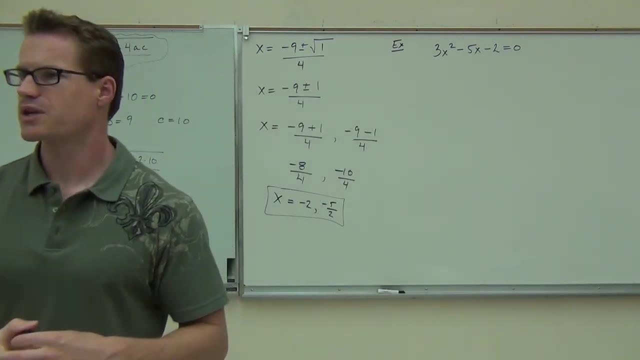 Okay, ladies and gentlemen, look at the board. The first thing I need you to realize is, well, first question I have for you, is this in the appropriate form? Is that how I want it? Yes. No. 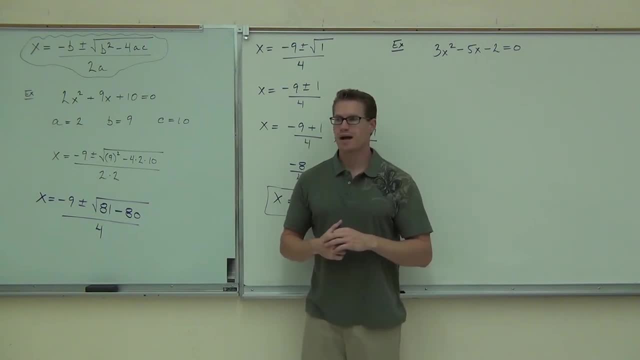 Why or why not? Do I have zero on one side? Yes. 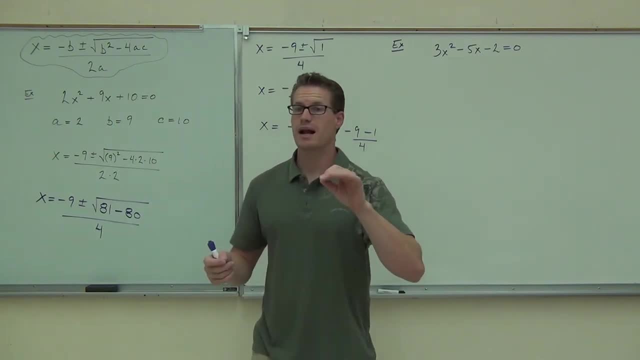 What I want you to do right now is find A, B, and C, and write it out explicitly, A equals blank, B equals blank. Write that out. Remember that when you find A, B, and C, it goes with the sign in front of that number. So with that in mind, how much is A, everybody? Three. How much is B? Is it five or negative five? Negative five. And C? Negative two. Do I have any X's when I do A, B, and C? No. You see, A, B, and C are numbers. They're coefficients. So you should never, ever have a negative five. You should never have an X in this formula. 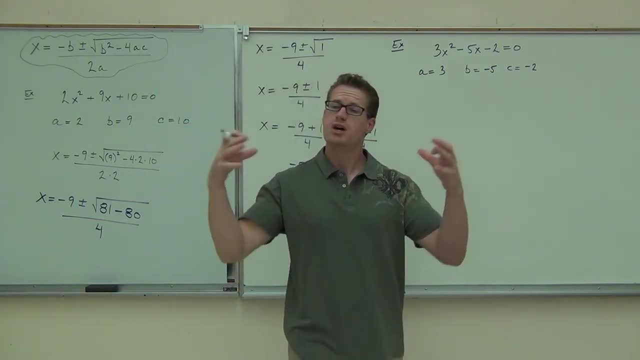 What this is doing is taking the values of A, B, and C, the coefficients, using them in such a way that you get your solutions, completing the square. That did that for us. Okay, what are you supposed to do now? Okay, I want to show you how to do this because this is the first time we have some negative numbers. 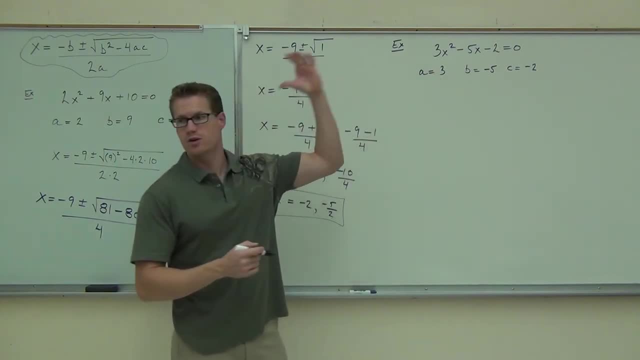 So when I'm taking this and plugging it into my, or substituting it into my quadratic formula, 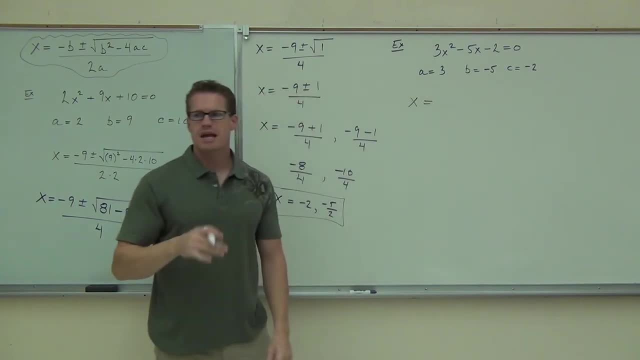 I'm going to have X equals, X equals negative B. We are going to write everything out explicitly without doing any math in our head. When we do math in our head, that's typically where the sign errors come in. 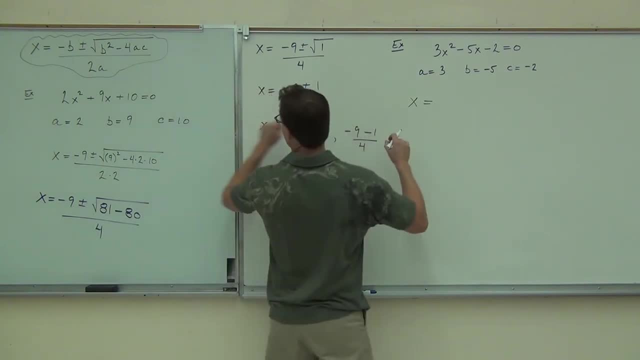 So when we do this, what's what I want you to write up here? We're going to write negative B. That negative is going to be there regardless of what B is. True? 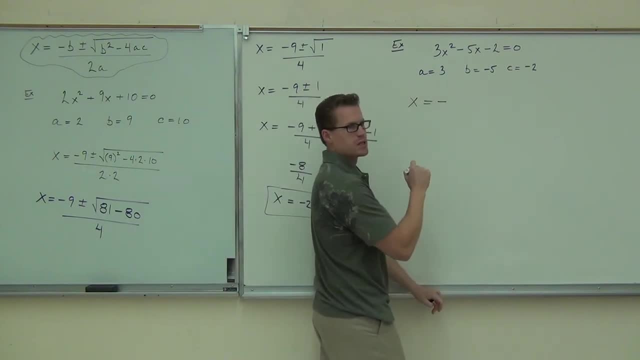 So when I write the negative, then I write how much B is. How much is B? Negative five. So should I have negative five or negative negative five? Negative five. Wait, like that? No. No. 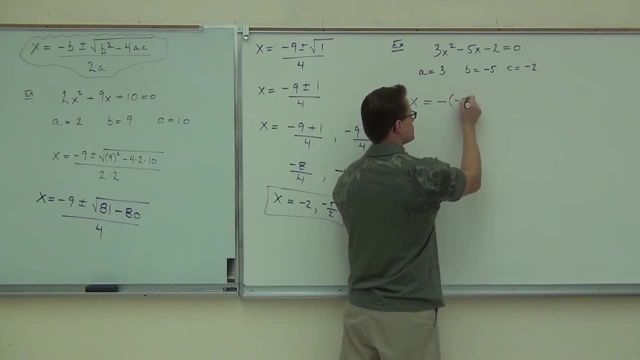 Good. Parenthesis says negative whatever that number is. Negative negative five. 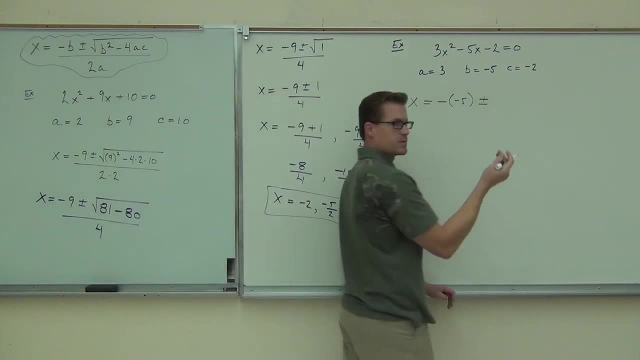 Then what do I write? Good. That's got to be there. It's a formula. Then the square root, that's a big square root covering everything there. Inside of that I have B squared. How much is B again? 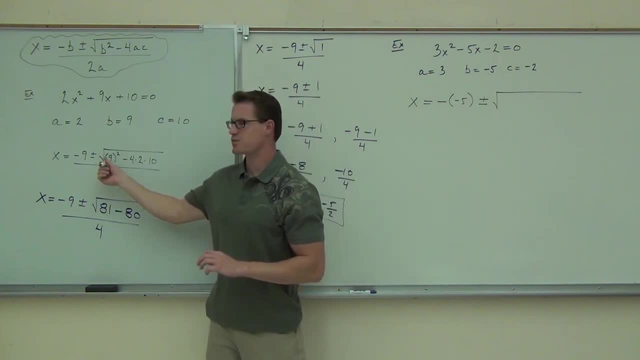 Notice this is why I wanted you, you were probably wondering why do I have parenthesis around that. I told you that last time. I want you to practice that because when you get to something like this. 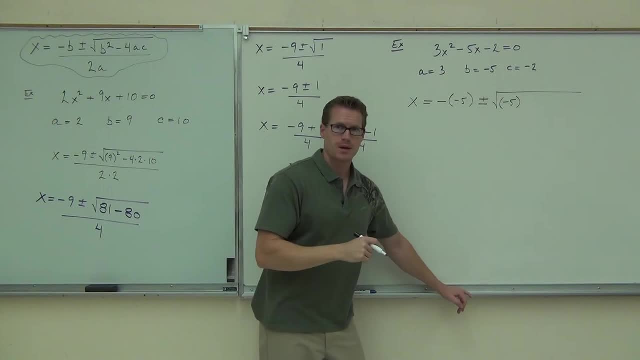 Look at the board, please. This right here, that right there is different than that right there. Those are different things. We've covered that a couple times. This right here would be negative 25. Do you see it? That would be negative 25. You'd square the five and then you'd apply the multiplication of negative one. You'd get negative 25. I've covered that just a couple times in here. 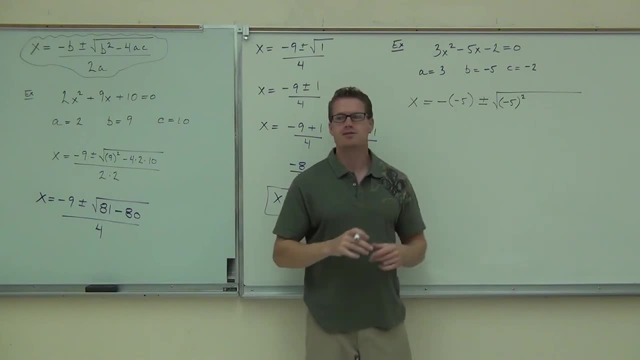 This right here is different. That says negative five squared. That's what you want to show. You want to show that number squared. Whatever it is, you're squaring it. So in this case, are we going to get negative 25? No. What are you going to get? Minus. Minus. Put it in parenthesis. 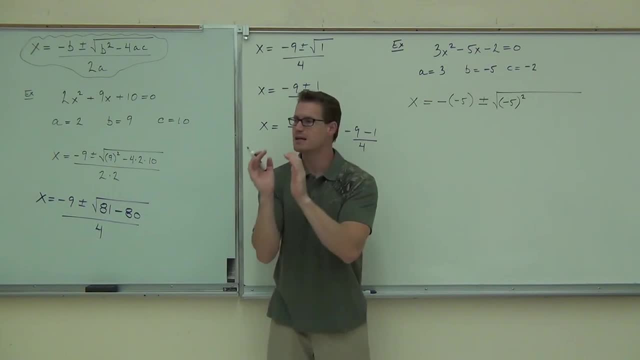 Practice that and make sure you have it in parenthesis, all right? Because that negative, that also gets squared. Then what do I have, ladies and gentlemen? Let's keep playing along. Minus four. 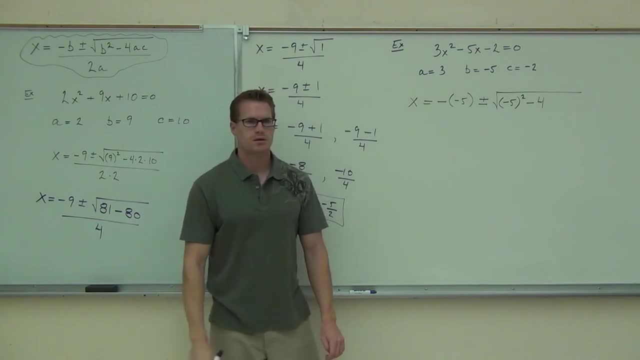 Minus, just like that, minus four? Times, times what? Times three, because A is three. 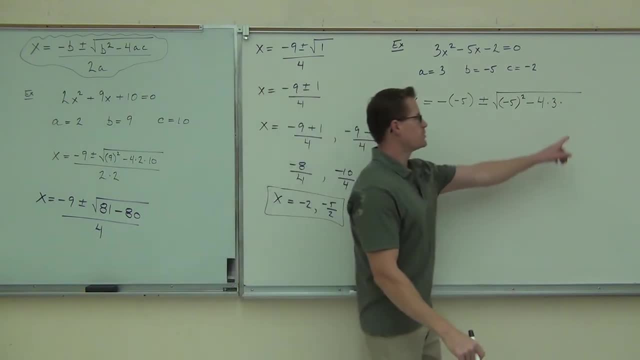 And then times C. How much was C? Two. This is the only place you put your C. You put B two places. You put A two places. You put your C only one place. 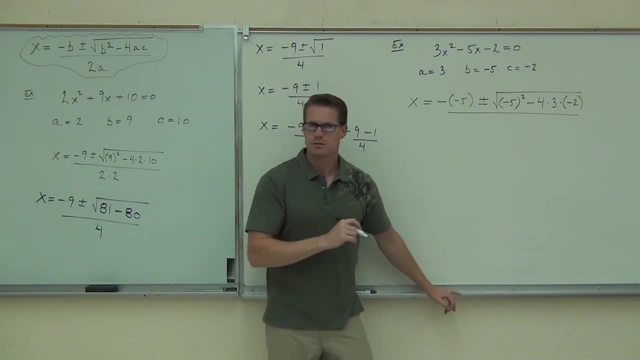 All over, all over what? Two times negative two. Oh, good. One over. Times what? Three. Three. 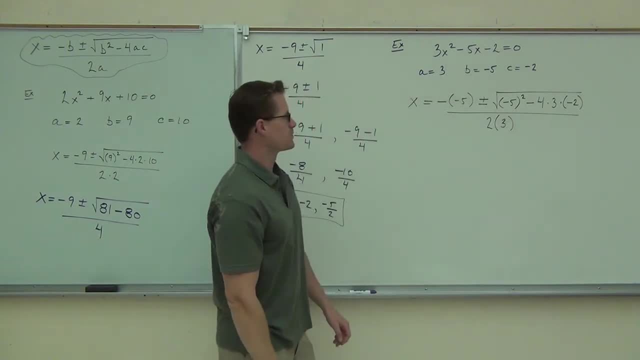 You put your A two places. C only goes one place. So we're going to double check before we do anything else. This is a good thing to do. Trust me. Don't just assume that you did this right the first time. Make sure you did it right. 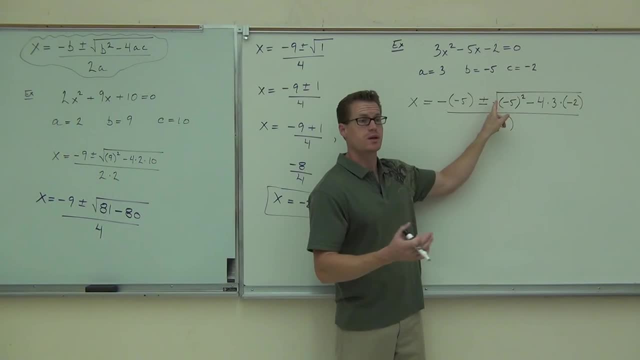 We have negative B, check. Plus or minus, okay. Square root, got it. 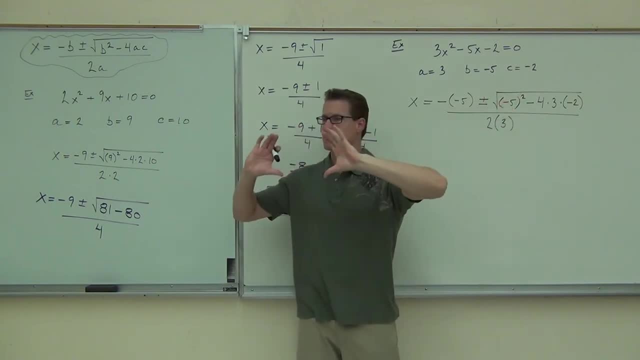 We have B squared, that's negative five squared. I've had that in parenthesis, making sure all of V is being squared. 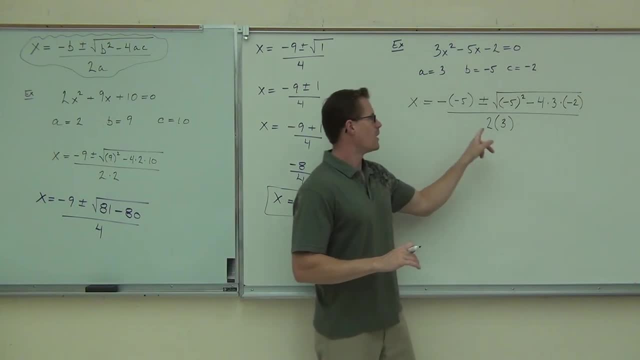 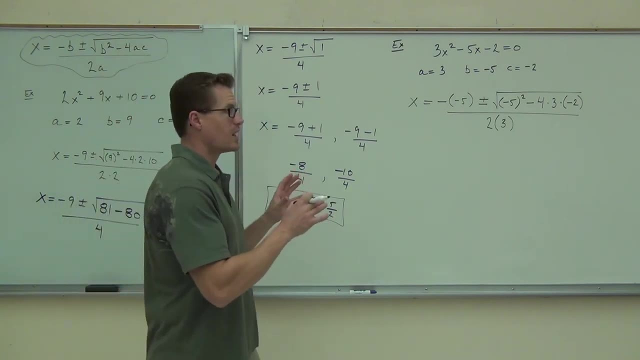 Minus four times A times C, got it. All over two times A, that's appropriate. That's exactly what we want. Now we work slowly, going through this thing, doing step by step, realizing that we need to go slowly in order to get these signs correct. So, let's start. 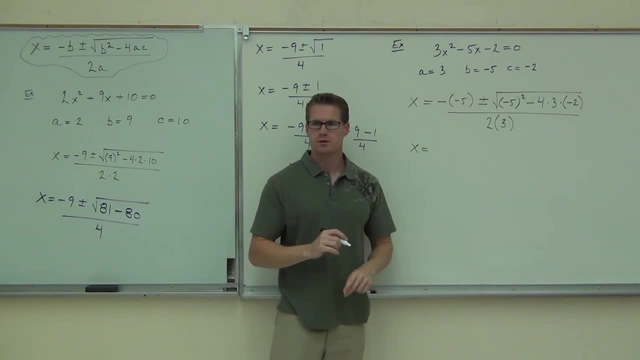 How much is negative negative five, folks? So I'm going to write positive five. The plus and minus, I don't deal with that until like the last step. Some of you guys are zoning out. I need your attention up here. All right. You need to be following along. And participating. 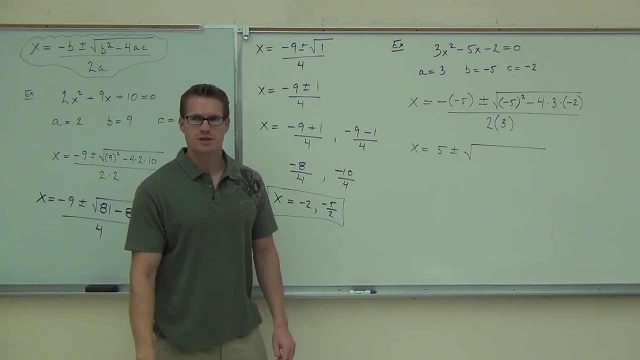 How much is negative five squared? Positive or negative? Positive or negative? Positive. Then watch what happens. I do have a minus. 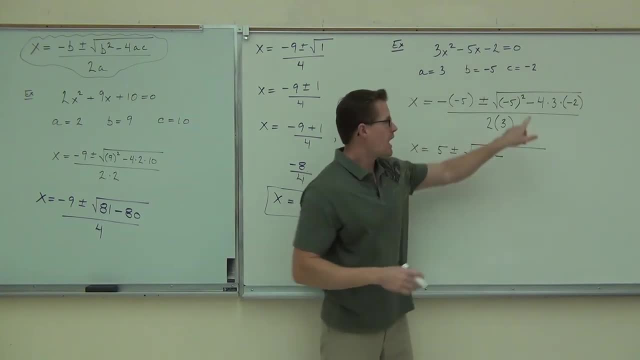 I'm going to write this out so you can see it so that we're not doing this in our head. I do have a minus, but how much is four times three times negative two? How much? Negative 24. Negative 24. Negative 24. Is that like that? Is that like that? Well, like this. Yeah. Is that like that? Yeah. 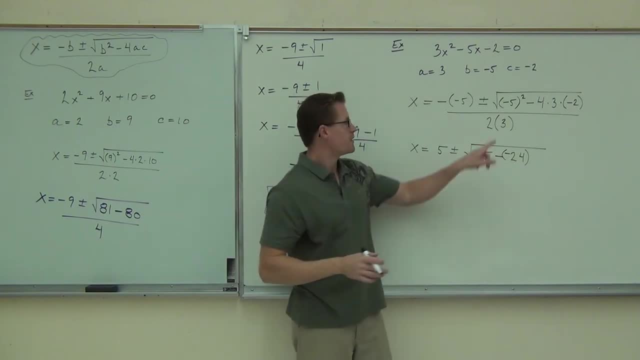 Don't lose those negatives or those minuses. This minus is this minus. That negative is that negative. What's that going to do to my problem? Am I going to subtract or am I going to add? Okay. You know what happens? I'm going to give you a problem like this on the test. 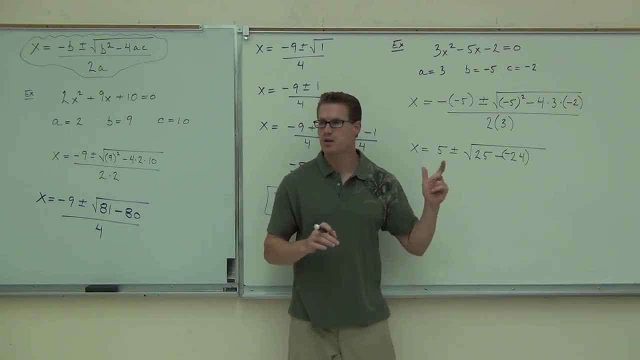 What happens here is people give me one of two things. They give me 49 or they give me one. Is that going to make your problem different? Yes. Can you see how people would get one? It happens all the time. People do that. 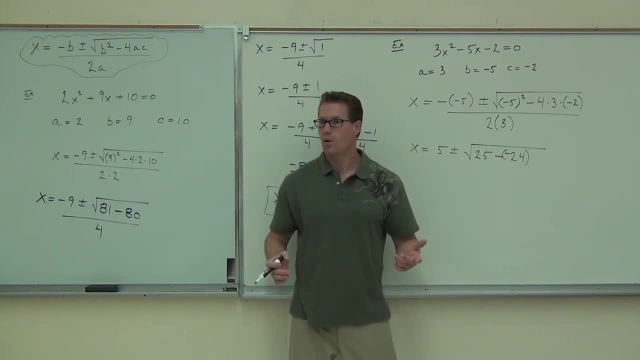 They get 25 minus 24 and they give me one. Or they do it correctly and realize, oh, I'm subtracting a negative number. 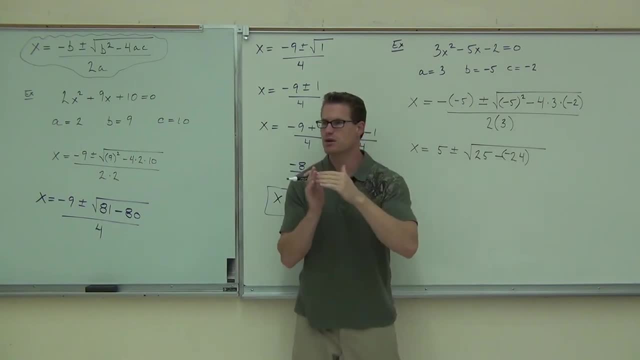 I'm subtracting negative. I've written that out. I see the minuses right next to each other. 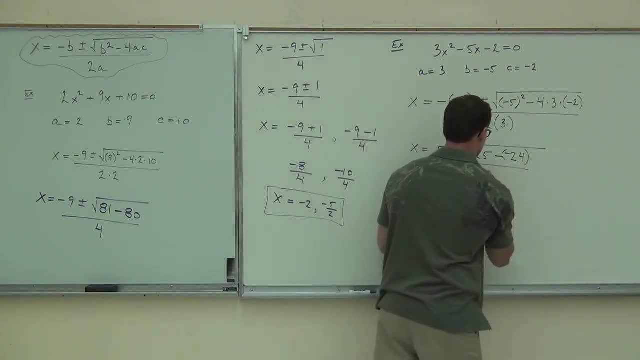 That's going to make it plus. Of course, we have all over six. 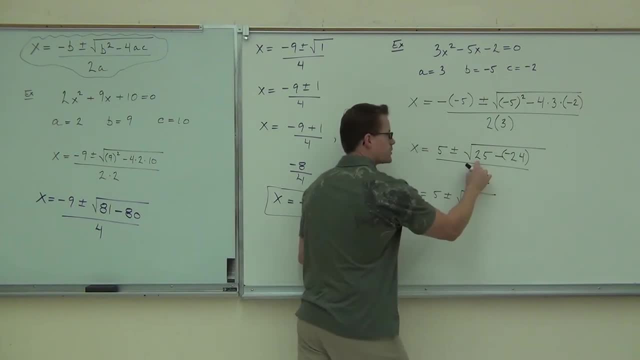 So this gives you five plus or minus the square root of 25 minus negative 24. 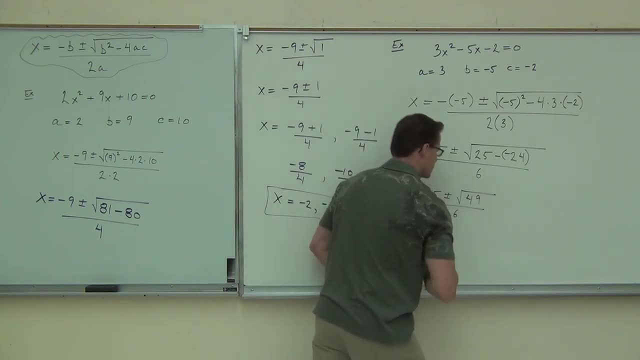 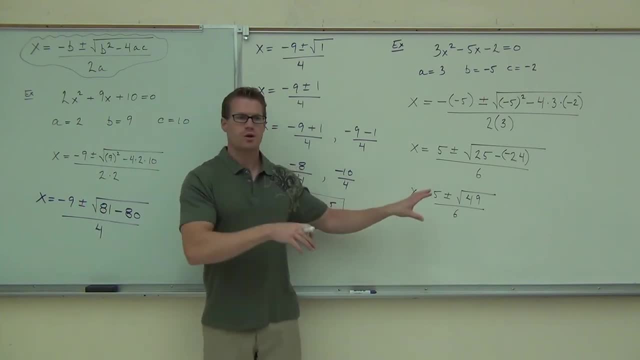 Square root of 49. Yeah, we can simplify that, right? Don't leave the square root if you can simplify it. Square root of 49, well, that's seven. 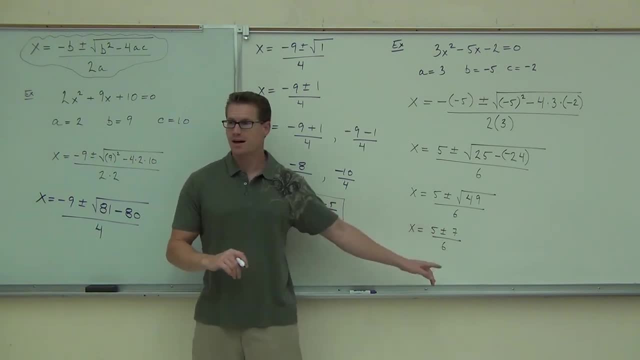 Okay, am I going to leave it like that? No. No, definitely not. How many solutions do we get? Two. Write out your solutions. 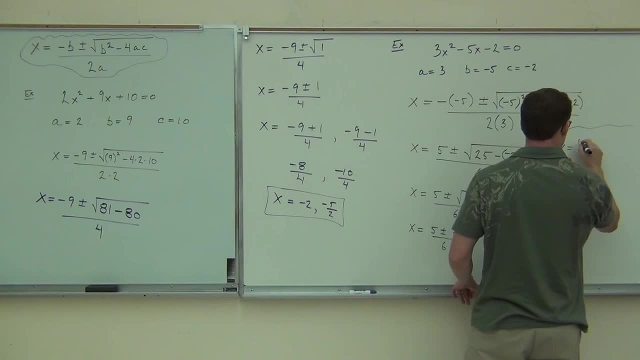 Five plus seven over six, five minus seven over six. The five doesn't change. Do we have a plus and we have a minus? Are we going to leave them like this? Is this as far as we can go? No, heck no. Shoot, do it. 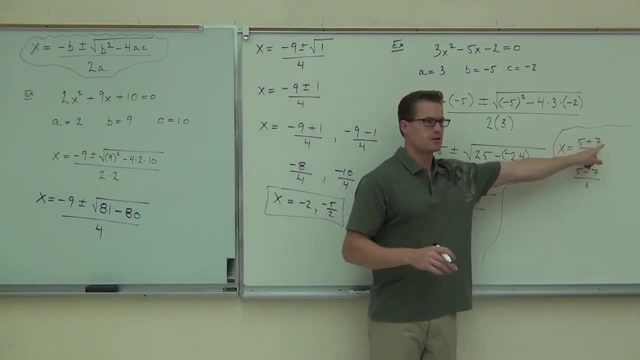 I mean, actually do the mathematics. You can do five plus seven, right? You can do five minus seven. Do those two things, you're going to get your two solutions in much better terms than this and way better terms than this. 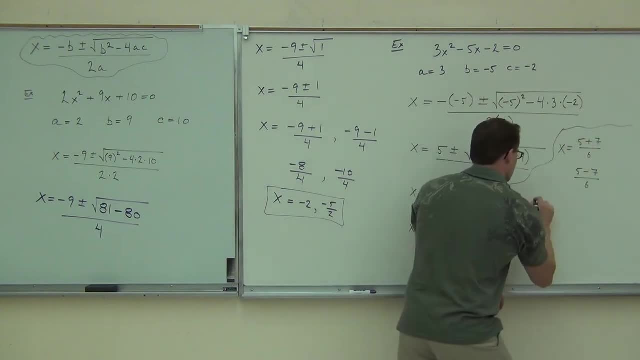 This is something you can actually work with. So we have x equals 12 over six and x equals negative two over six. You see where those numbers are coming from, folks? We have 12 over six, negative two over six, and we're going to do what now? x equals two and x equals negative one-third. Good, so we're going to simplify those fractions. 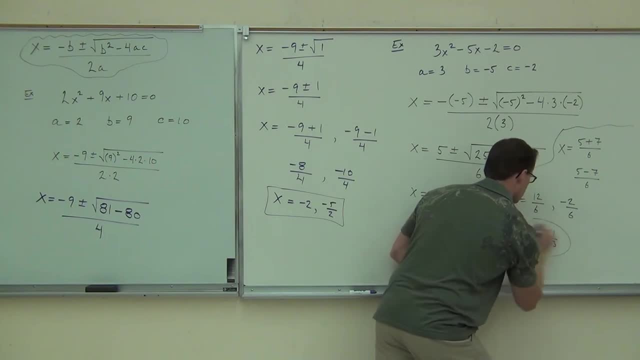 Two, sure, negative one-third, got it. Would you raise your hand if you feel okay with this? Are you okay with this so far? Pretty good about it? Oh, I missed it. 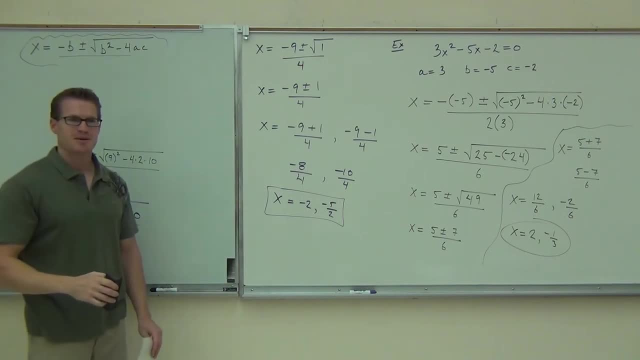 I erased lyrics to a song. Oh, that's heaven forbid. Did you watch this song again on the internet? 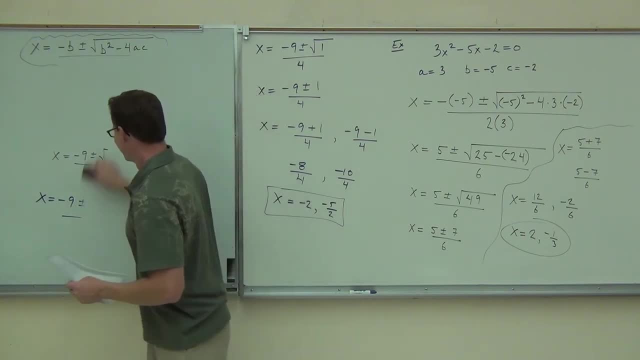 I put it up there so you can watch it. Mr. Knight, can we have some of the lines of that little x thingy that song? Do you have some of the lines? Wait, wait, wait, wait, hang on. Repeat that, please. Do you have some of the lines? Hang on a second. Occasion. Do you have to memorize it? Sorry. That thingy up there, that x thing. Do you have to memorize it? What's that thingy called? I got it. Okay, it's called what? Discriminant thing. I'm discriminating you against you by making you memorize the thing that you're discriminating? Do we have to know that or are you going to give it to us? Do we have to know it? I taught you a song for it. Did you post it already? Yeah, I emailed it. Why didn't you email it back? But did your daughter not believe you? 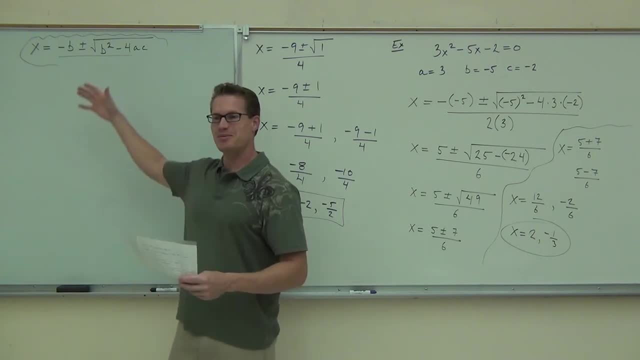 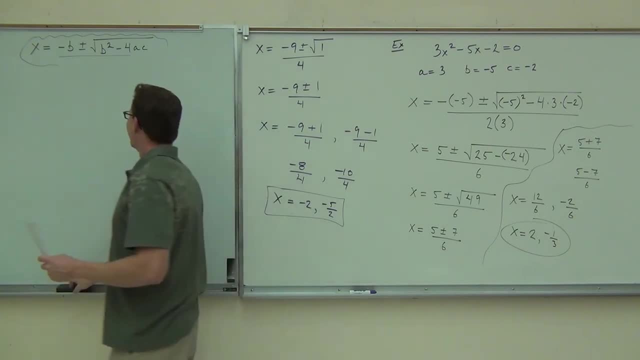 She said, that's something only kindergartners do. She said, well, I teach college. There you go. 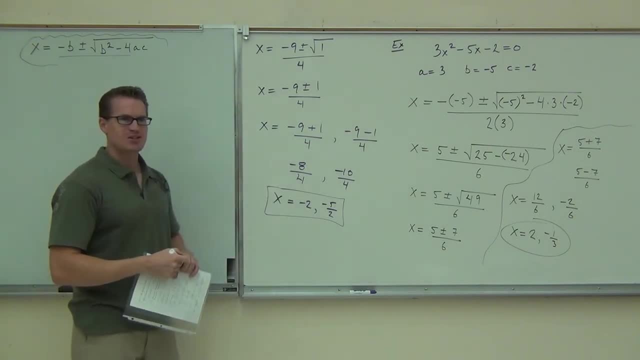 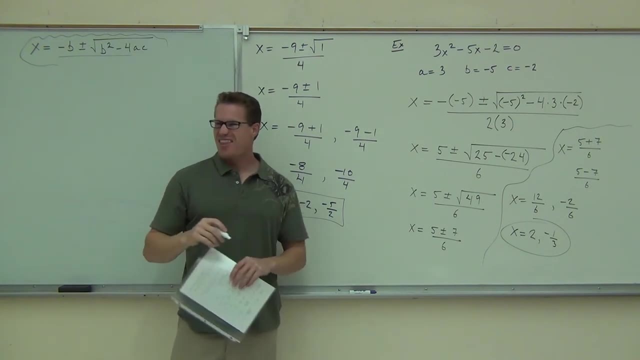 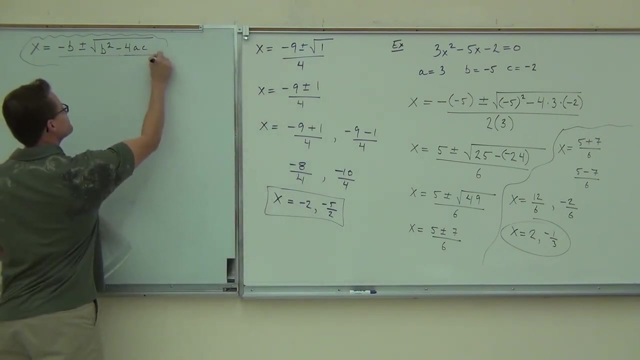 But the mind, the wood, and the approaching end. 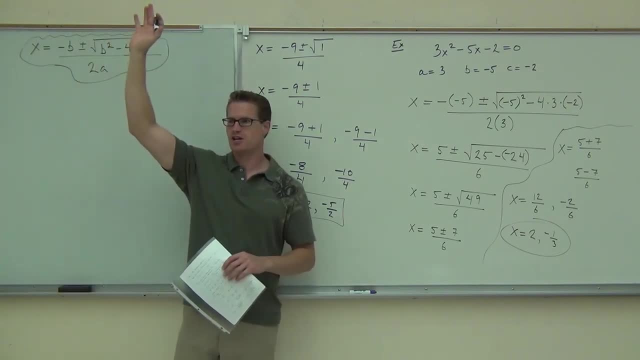 who is not here for the song shame on you shame on you no I'm not using you know one time you have video you can watch it forever you're gonna sing it 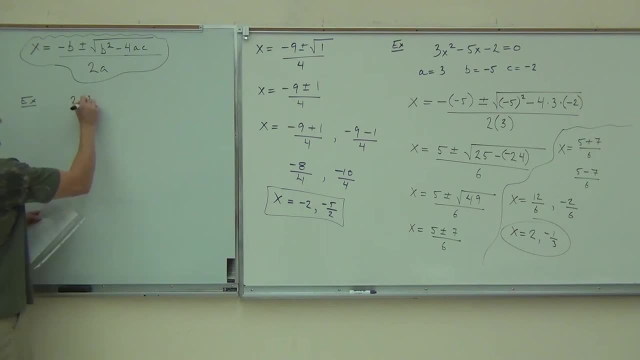 again I guarantee you actually I should make the people who weren't here come up here and sing the song I don't think I'm going to because they'd have a mutiny 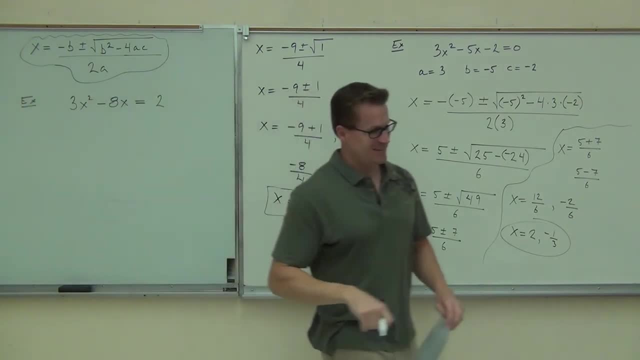 but anyway okay we're going to do two more problems together I'll give you a couple to your own but honestly it's the same thing over and over you just need to know how to manipulate these equations to get them in the right form 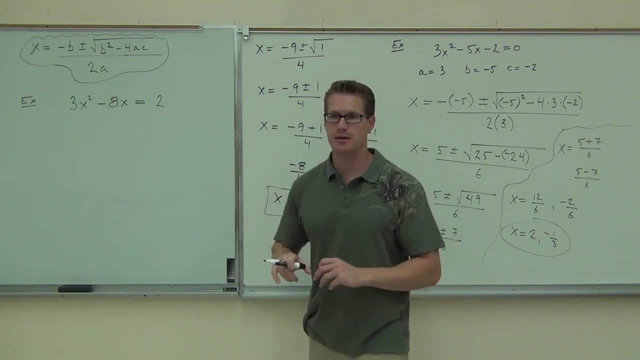 so first question is is this the same as the first two exams we've done what's wrong with this okay so if you try to look at the board here looks like I know papers are going around but you still need to pay attention here if you try to do this right now you get a is B 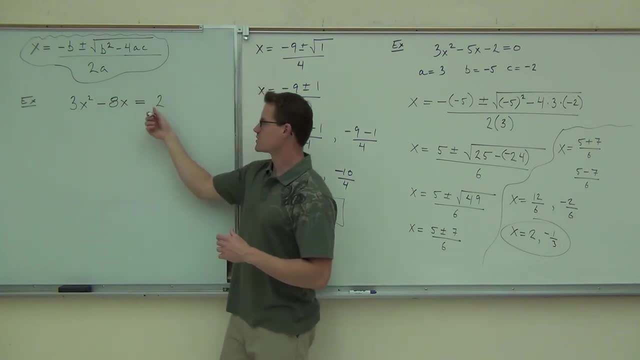 I'm not sorry a is three B is negative eight and if you think your C is two do you have it right that's wrong you know people get confused on that they look real quick they go oh it's almost right hey no problem but there's no zero there's no zero you cannot use the quadratic formula so do the first step right now get that in the correct form 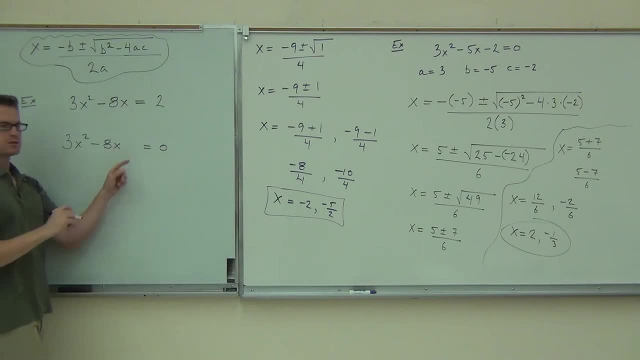 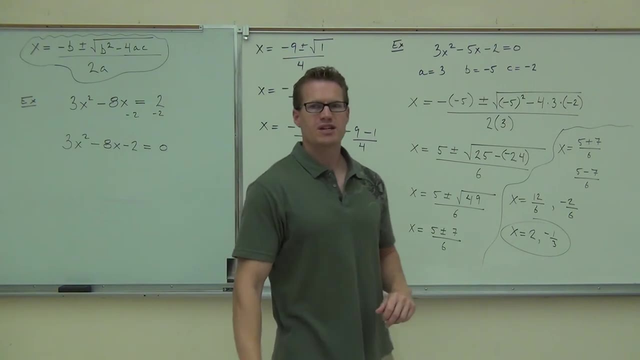 what goes right here plus two or minus two because you subtracted two from both sides okay what's the next thing good you could use if you're going to use a quadratic formula A B and C look at the board here real quick with me please would you do a completing the square on this problem okay there's two different questions could you you could would it be easy what would make this hard to do the completing the square 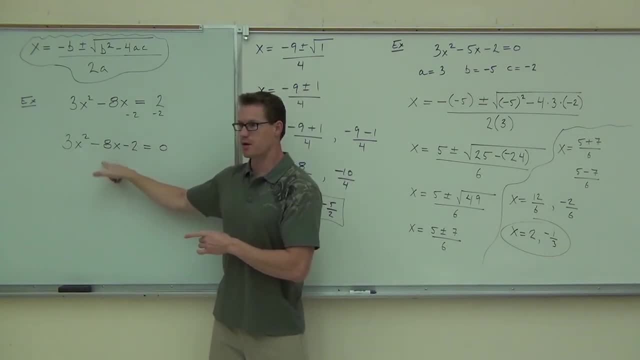 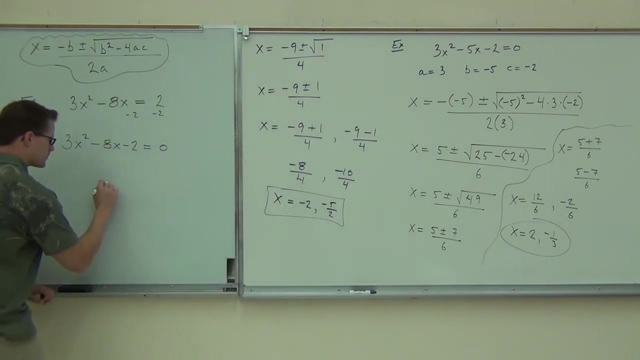 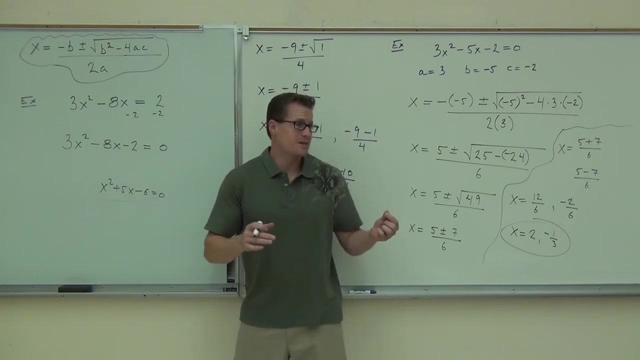 that makes it hard and when you divide it that makes it really hard okay are you going to want to do this completing the square you're not going to want to do that could you factor it you could try I don't know if you can or not but you could try you'd have negative eight you'd have negative six right that's not factorable so you'd spend ten seconds trying to do that don't forget the stuff that you know already you do know how to factor things diamond problem extra step right you do know how to do that in the next section if you try to do quadratic formula all the time it's going to work every time listen listen here the quadratic formula works every time no matter what without fail it will work for you but sometimes factor is easier if I give you something like this could you use quadratic formula absolutely it's factoring easier definitely yeah positive six negative one so the X plus six X minus one that's way quicker than the quadratic formula so don't forget that you can factor stuff you should try that first if that works spend ten seconds doing it if you can't do it in ten 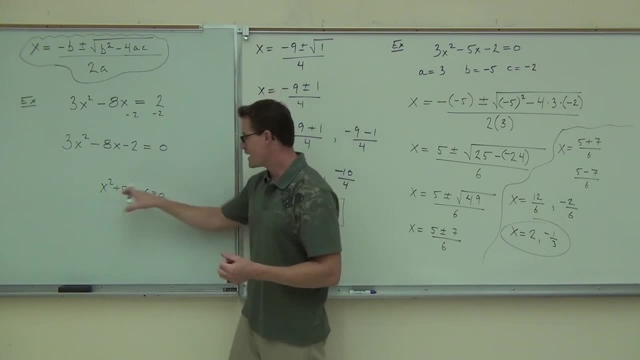 seconds then the quadratic formula is quicker but if you can factor it in ten seconds shoot do that does that make sense to you so do not lose the stuff 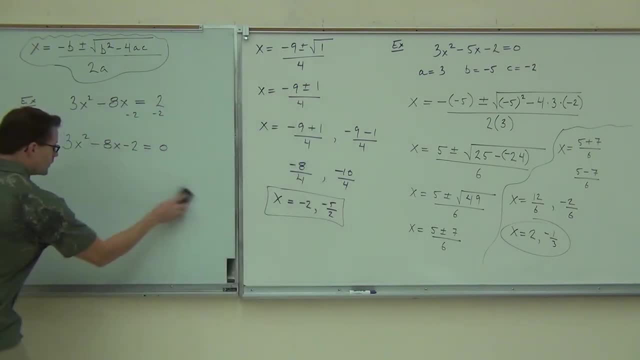 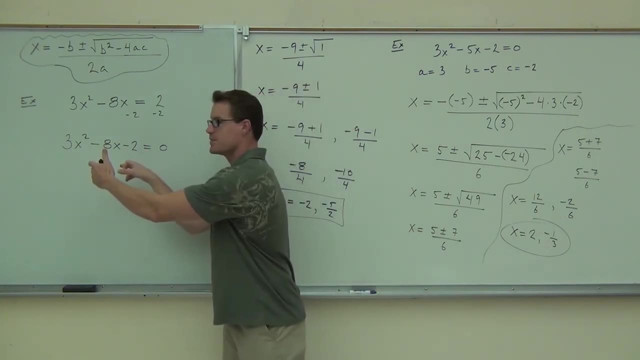 you've already learned in this class okay now you said a B and C sure because I can't factor that in ten seconds it's an a factorable so we're gonna go ahead and we're gonna find our a B and C do that now right at the bottom so we're going to go ahead and we're going to do that now right at the bottom 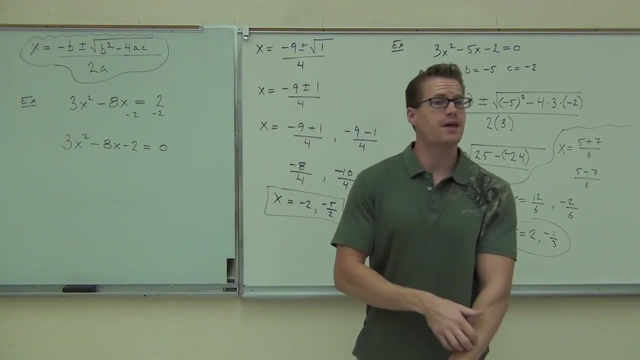 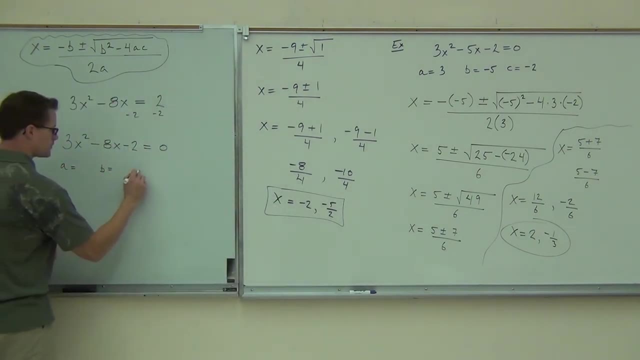 Write it out explicitly for me. If you've already done that, try plugging that in the quadratic formula. Okay, how much is your A, ladies and gentlemen? One person knows my A? Three. How much is my B? Negative. And my C? Negative. Perfect. 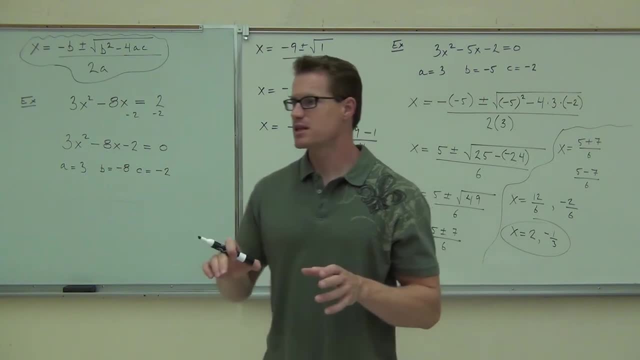 Now, after that, once we find our A, B, and C, we should be pretty good. I mean, that's it, right? It's in the right form. 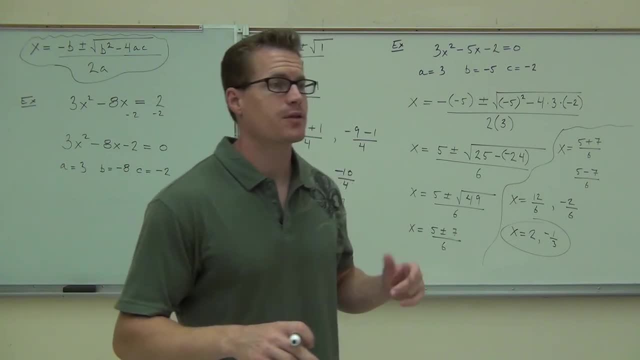 We're going to take those numbers and plug them into the quadratic formula without doing any math. 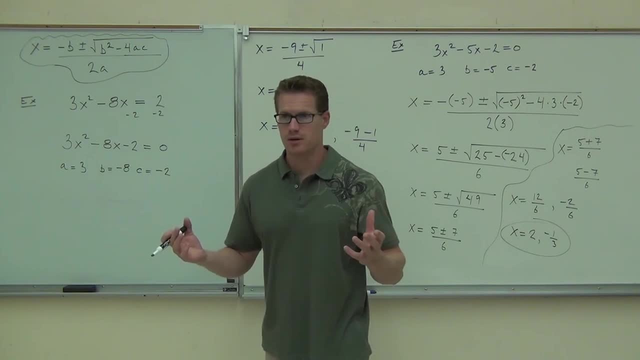 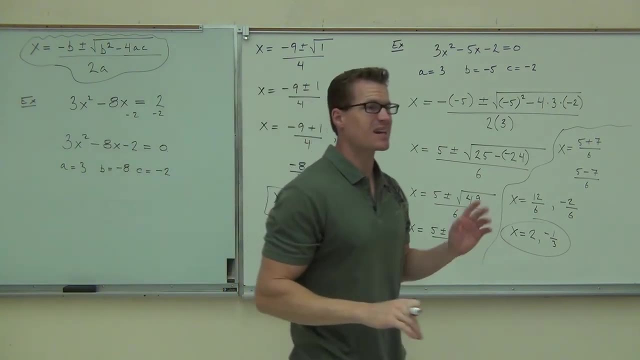 That's what I want you to practice right now. You should have several parentheses up here. I want you to plug them in here without doing anything except plugging in those numbers. So go ahead and take about 10 seconds and do that now. Notice that once you get the hang of this, this actually does go pretty quick. I mean, this is just a formula. You're just substituting. That's nice. Okay. 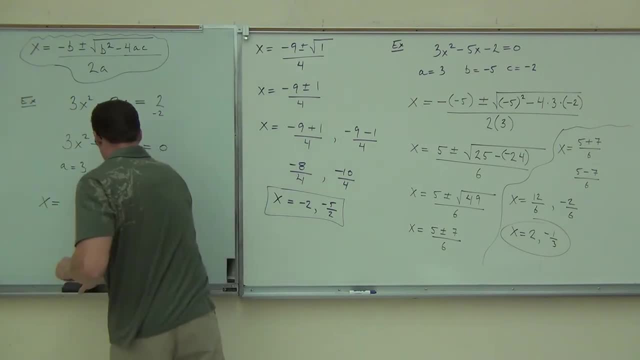 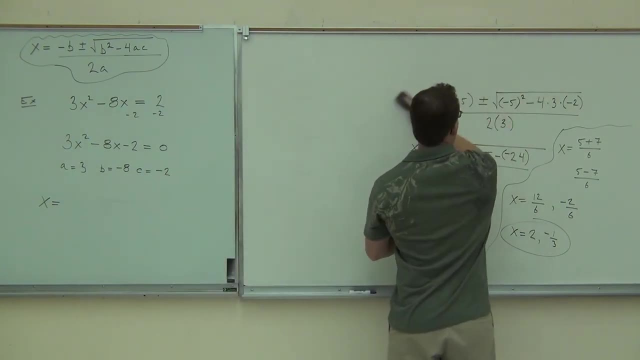 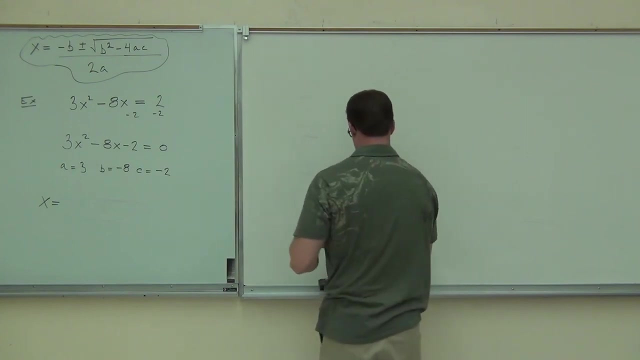 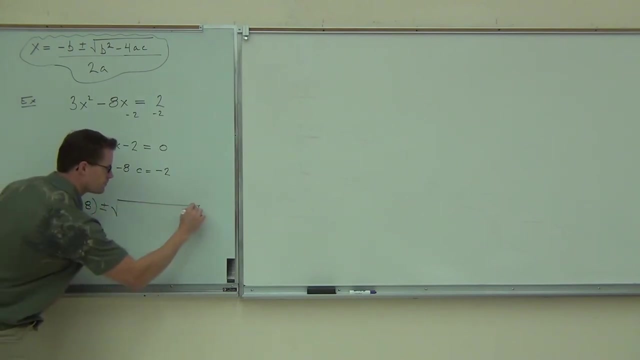 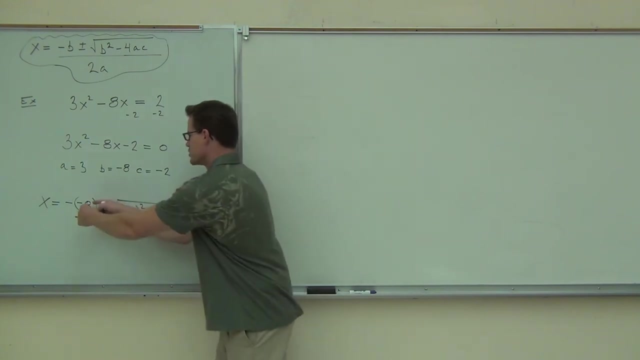 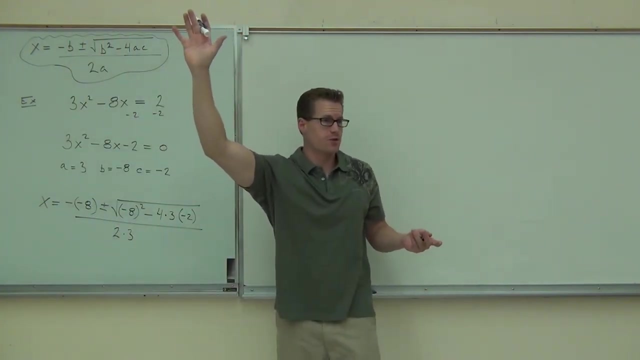 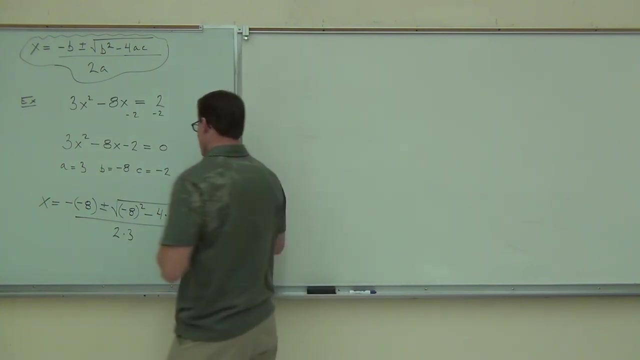 Let me see if I can get it. Okay, x equals, well, we're going to have negative B. In our case, negative B is negative negative A. You should have parentheses. Then we have a plus and a minus. minus and we have a radical because that radical is going to be an inequality that you ever do then we have b squared if b is negative 8 like it is in this case we've got negative 8 squared then we have a minus and then we have 4 times a times c that's 4 times 3 times c which is negative 2 and then don't forget to divide you know what some people are going so fast sometimes they just give me this and they forget that there's anything down here or they just put a 2 it's not just a 2 all the time it's 2 times a 3 raise your hand if you have exactly that on your paper that's what i want to see that's worth partial credit that's worth at least a few points because you understand how to use a quadratic formula now if we can get this right this is worth like maybe three or four points out of ten maybe three or four at least that's something but i do need to get correct answers right because this is useless unless you can manipulate to get it right but from here there's 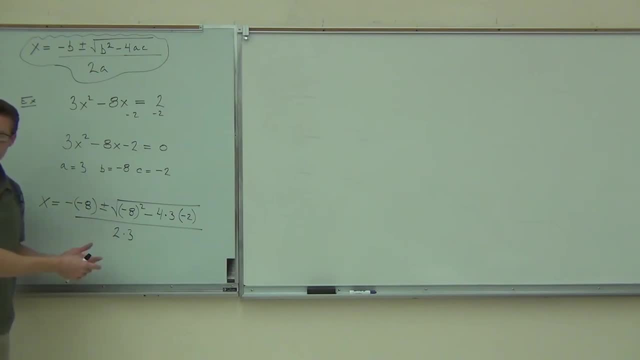 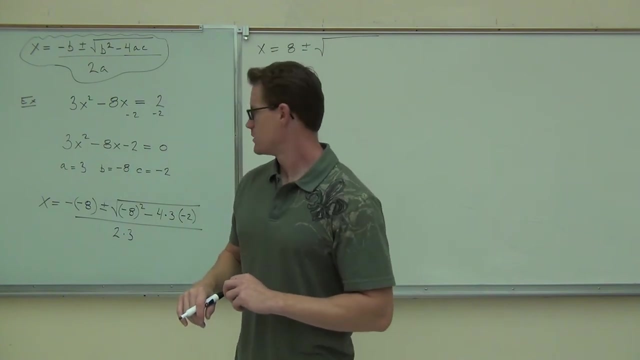 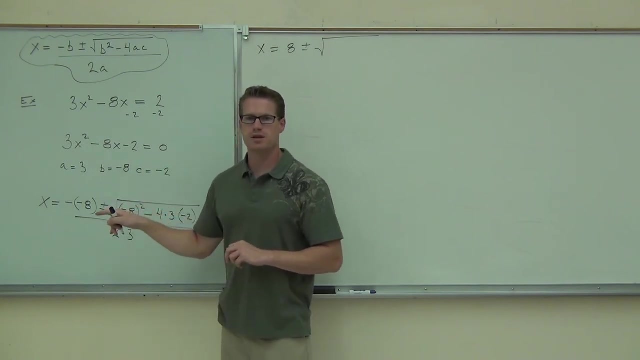 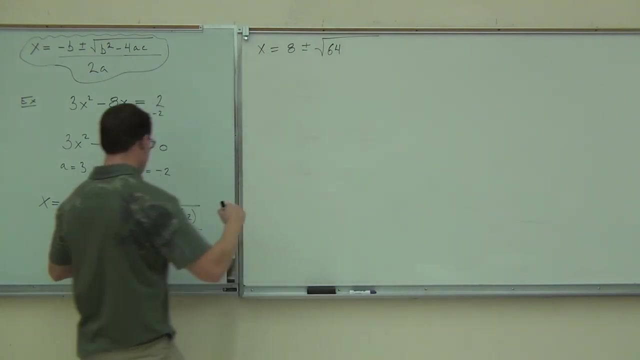 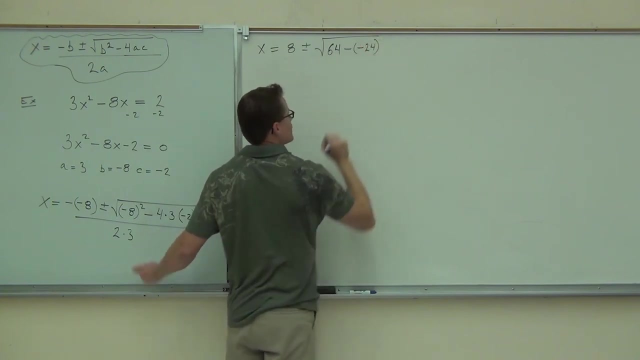 a actually no math c going on there's only pre-algebra going on there's just changing signs there's just squaring numbers multiplying subtracting maybe figuring out a square root but you do that in pre-algebra too so let's go ahead and go real slowly through this we're going to do negative negative 8 how much is that so positive 8 plus or minus square root what's the first thing in our square root folks it's 4 this the first thing in our square root is going to be positive or negative do you ever get a negative no not from this part now can you get a negative within your square root yes sure if you've done all this math you might get a negative but this first part will always be positive because you're squaring a number okay then we have a minus sign what are we subtracting negative 2 okay good so So you should have a minus and then a negative. Do you have a minus and then a negative? Yes. Good. 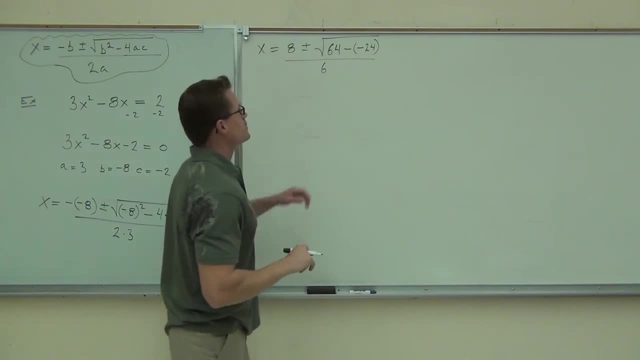 And then all divided, don't forget about that. Let's continue going. 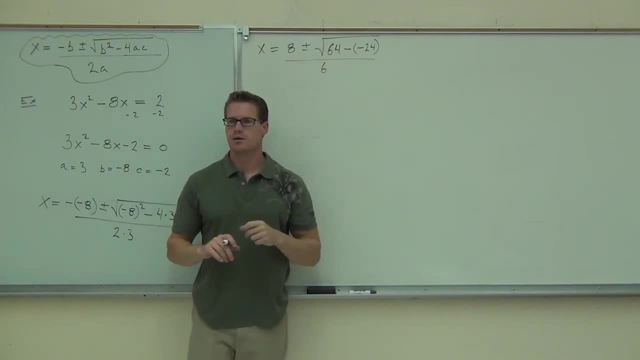 How much is 64 minus negative 24? 88. We're not gonna get 40? No. Oh, what? Are we subtracting or actually adding? We're adding. Plus or minus, you said 88? Yeah. Over six. Over six. Done? No. No, simplify the radical. Go ahead. Can you simplify the radical like we did in every other step? Yep. 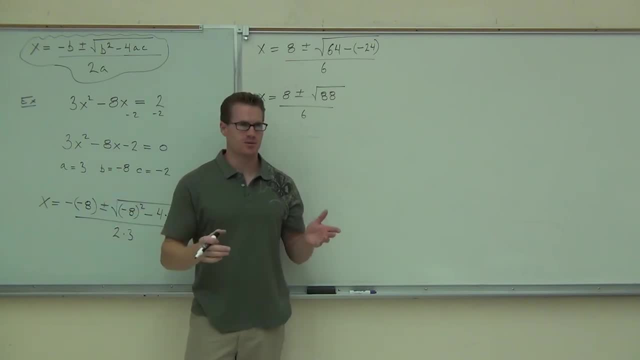 Now, I can't say, what's the square root of 88? And you go, oh, it's seven. Well, that's not gonna work, right? But we can find out what that is. What number goes into 88? Four. You okay with that? You sure? 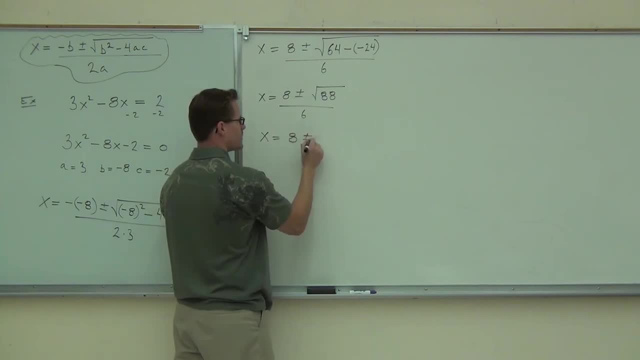 So this is eight plus or minus, notice that this is four times 22. That's gonna give you two root 22. Do you see where the two root 22 is coming from, ladies and gentlemen? Yeah. All over six. Are you done now? No, you need to simplify. We can. 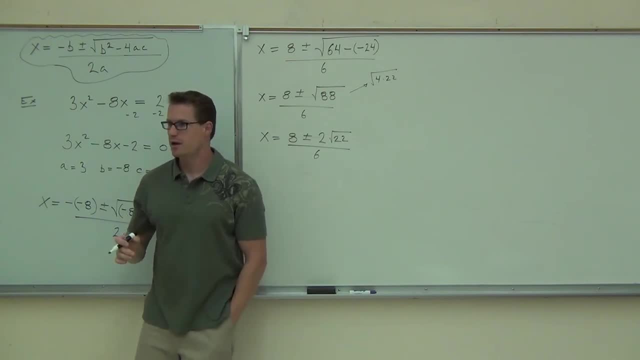 You could write this as two solutions now, but that's not good enough. 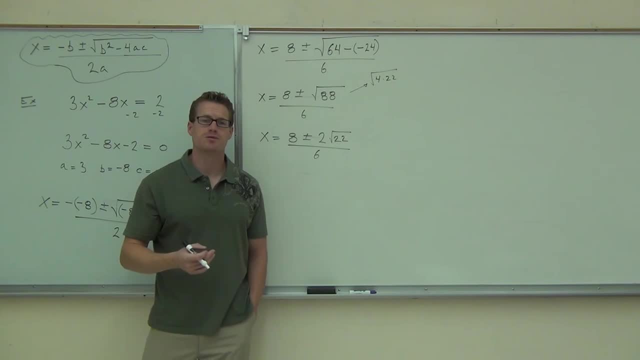 Okay, this answer will never be in the back of the book. This answer's not simplified. 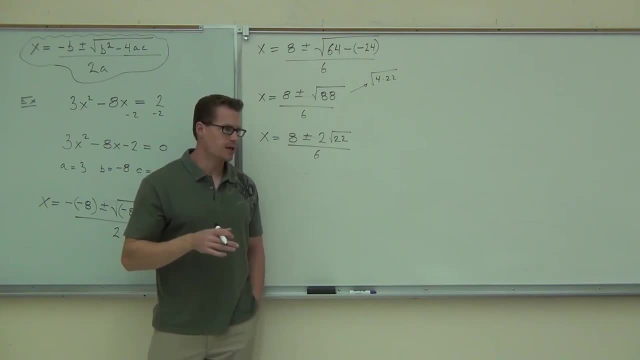 What you need to do on these problems, you actually need to factor if you can. I want you to notice that if I go with the six here for a second, notice how two can be divided out of that. Do you see that? You with me? This is, really, this is like eight plus two root 22 and eight minus root two root 22, right? Two is a common factor here. 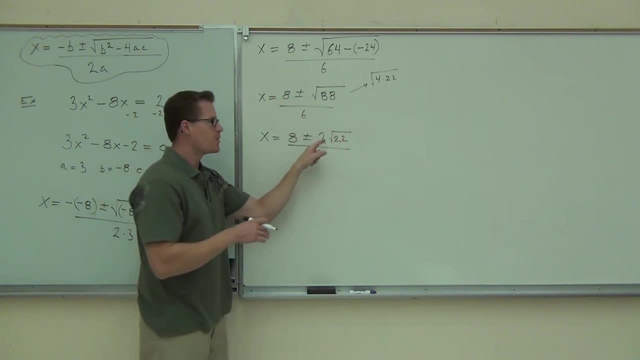 Not the, leave the 22 alone. You've already, you've finished that part. 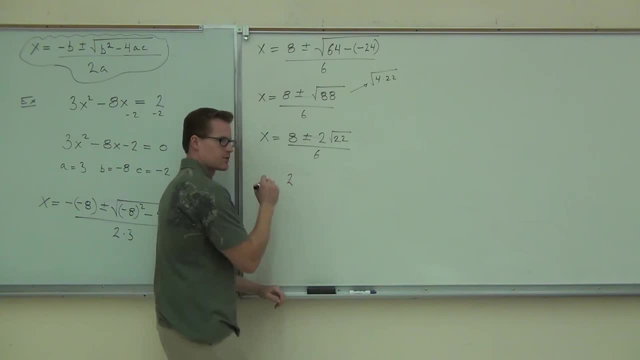 But this can be factored as two, watch carefully, four plus or minus square root of 22. Hey, wait a minute. How did I get the four? 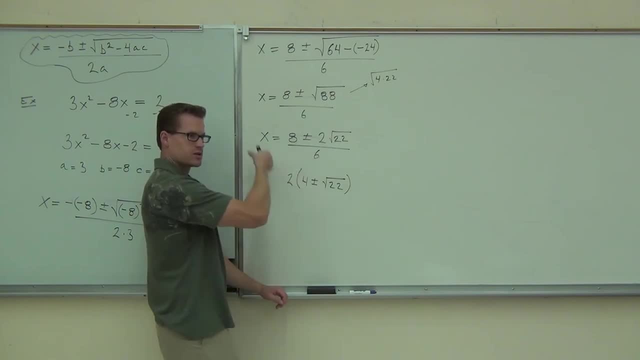 I factored it, divided by two. Factoring means divided by two. Where'd this two go? I factored it, I divided it, threw it away. 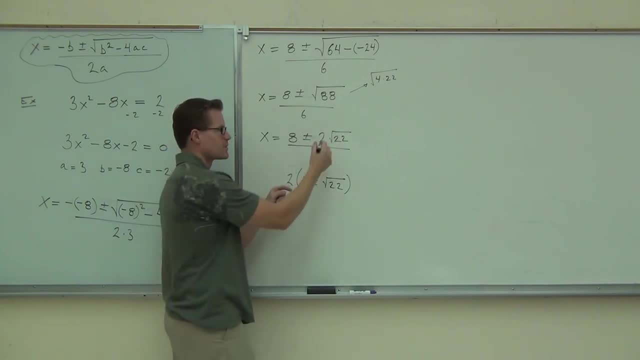 Why didn't I do that there? Well, that's got a square root. I've already taken away the two. Remember, this is two times. So if I divide this whole thing by two, I factor out the two. The two's gone, the 22 stays the same. If I factor this by two, I divide that by two, I get four. All over how much? Face. 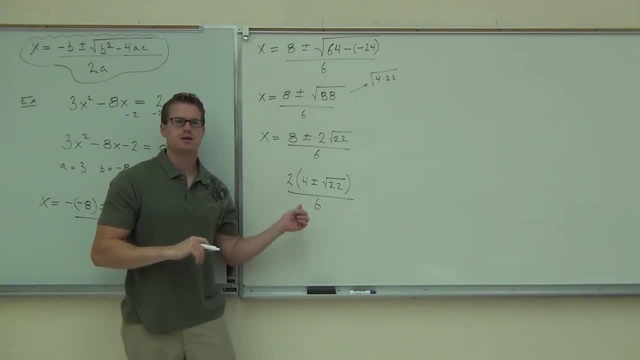 Hey, hey, look it. Can you simplify this now? Yes. Yes, absolutely, absolutely you can. So when I simplify this, this is two times, this whole expression, I can simplify two times something. That becomes a one, this becomes a how much? Three. So x equals, the one doesn't do much. 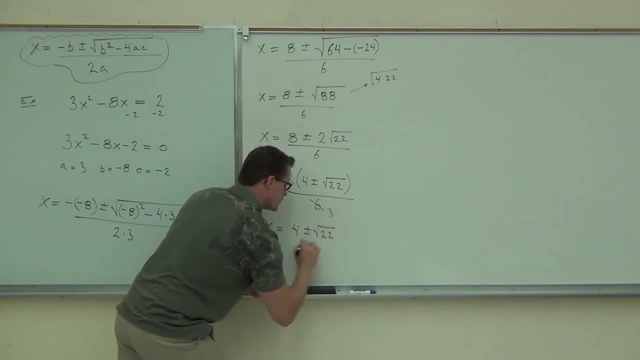 I have four plus or minus the square root of 22 over three. I am almost done, almost done. Do I have two solutions? No. Well, I don't. 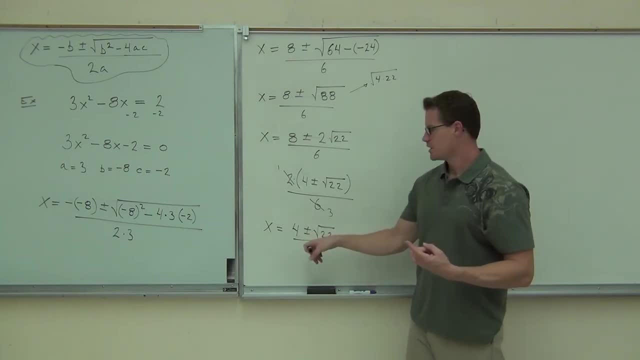 Sure, that plus and minus gives me two solutions. Write it out now. 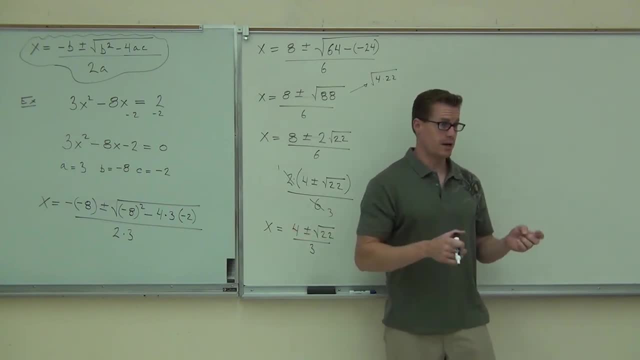 It's all simplified as much as I can. I just want you to write it out now. 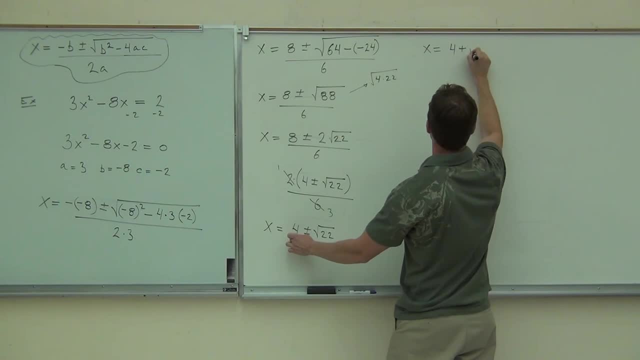 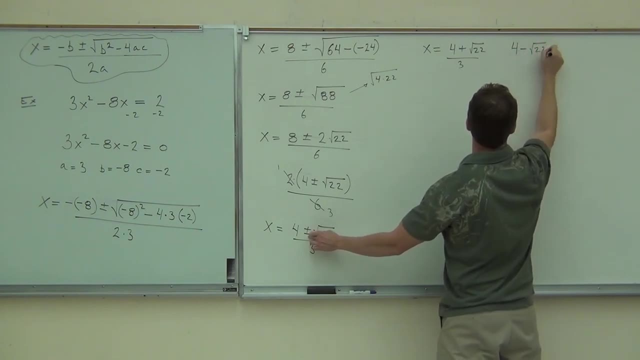 So x equals, we'll follow the stream, four upstream, plus root 22 over three, and four downstream, four minus square root of 22 over three. 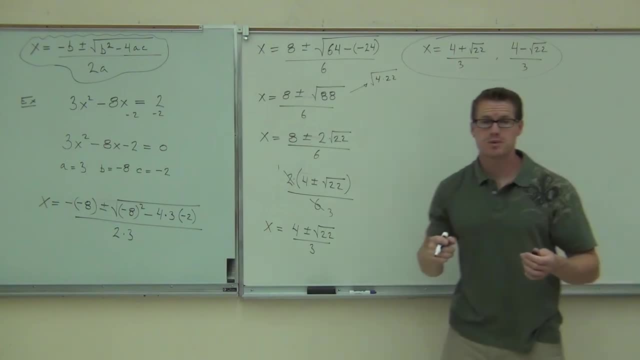 Those are the two solutions that you should get. That's as simple as possible. That is what would be in the back of your book. Okay? 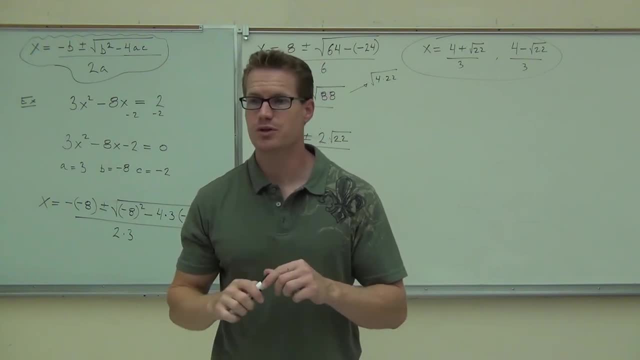 So if you're doing this problem, listen, this happens a lot when you're doing completing the square and quadratic formula. 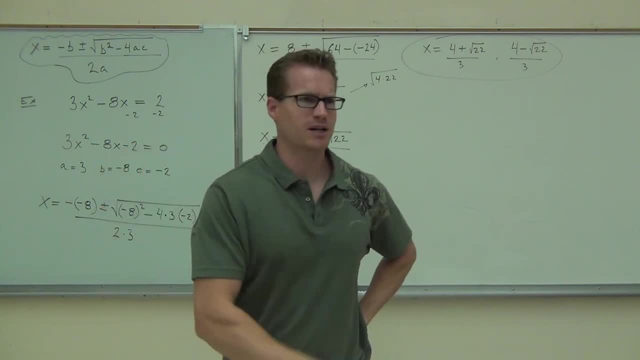 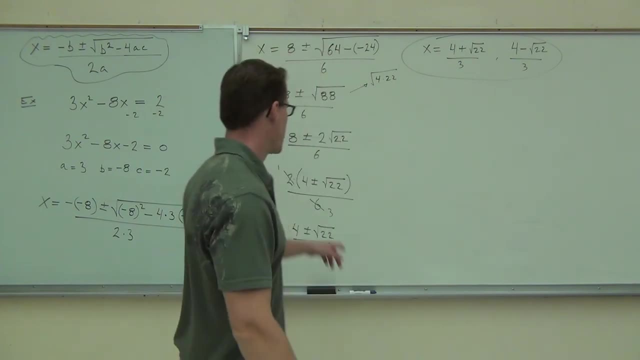 If you're doing the problem, you get all the way down, you go, crap, it's not in the back of the book. You're checking your answer's in the back of the book, by the way, right? I hope you are. And you go, dang it, what am I doing wrong? Maybe nothing. Maybe you just haven't gone far enough. If you write this, this doesn't look anything like that. 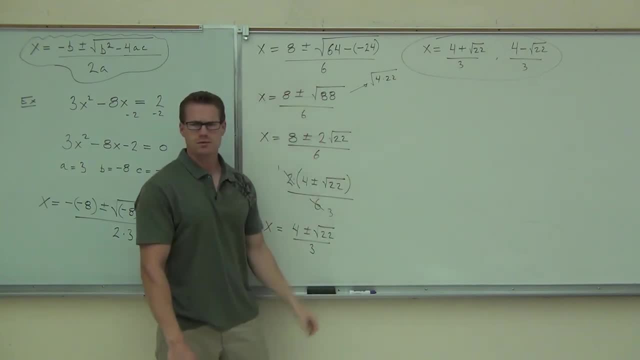 Every number is different except the 22. So if you get this and go, whoa, I thought I was doing it right. What happened? Well, either you messed up a sign, you plugged in the A, B, and C wrong, or you haven't simplified enough. 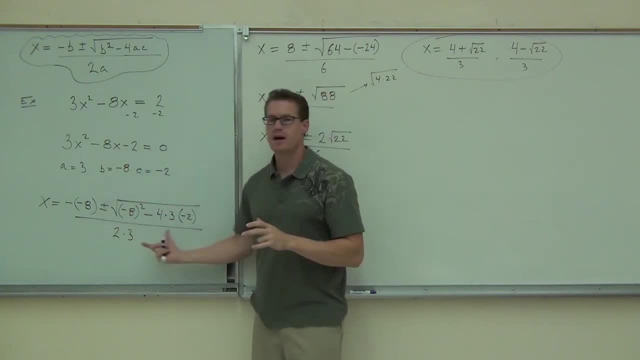 So check whether your A, B, and C are correct. Check whether you did your math correctly. 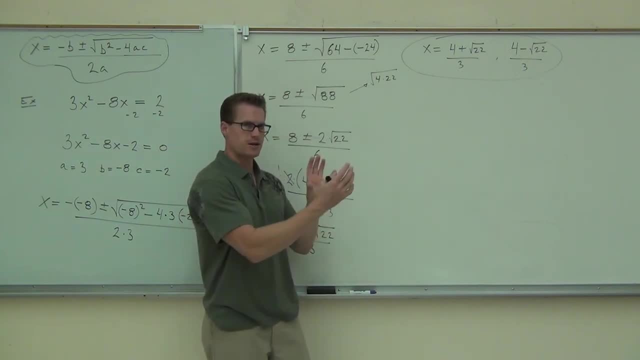 But then, if you did, well, try simplifying. Factor out the number and simplify it. You guys all right with that? Okay, so make sure you are factoring. 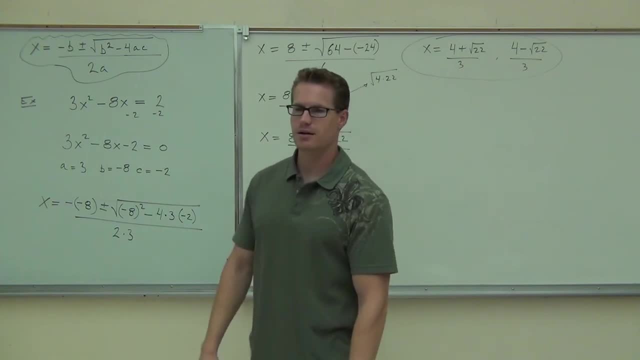 I did put up your answers for the test review last night, like eight o'clock, you're welcome. You're welcome. 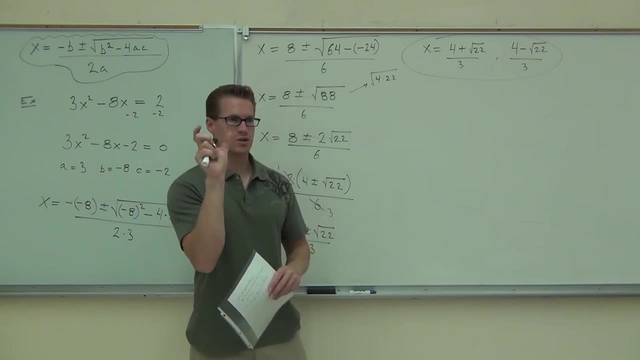 And you'll notice sometimes I give you two answers. The first one is what you should have initially, and then there's a little arrow, and the arrow says, that's what I want. Okay, the arrow is go further. Give me that. How many people feel okay with what we talked about so far? 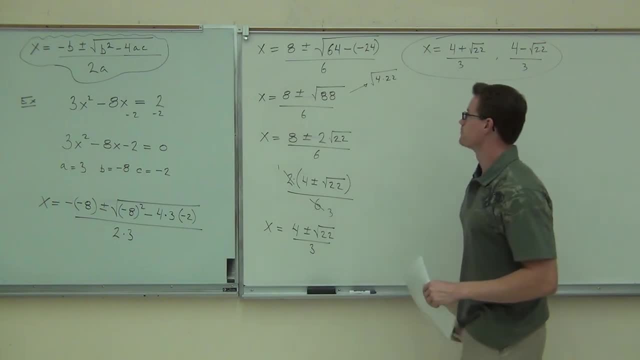 So you're putting things in the correct form first, and then you're just working it out. Are there any questions on this? Because I have to erase this to go on. It's pretty straightforward though, isn't it? Pretty straightforward. Nice. 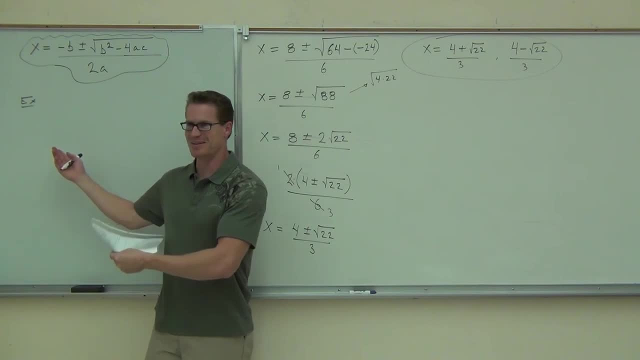 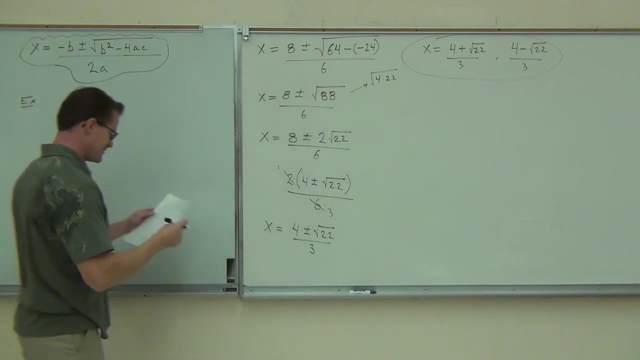 Now, you knew I was going to do something to you right here that's not fun. You knew that, right? You knew that, because I'm building these up. I mean, of course, I'm making them more difficult. It's Friday. It's Friday after all, so why ruin your good Friday with rain and with fractures? Right now, I have one. 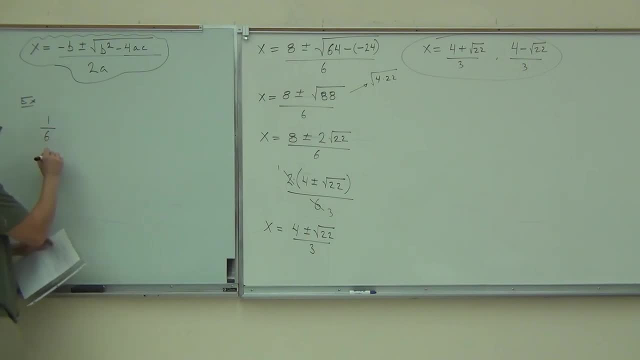 Right, right, right. Yeah. 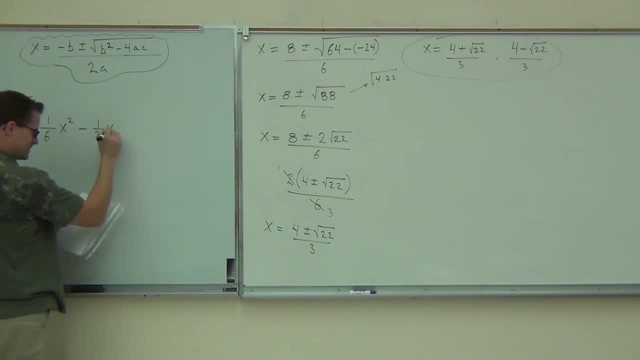 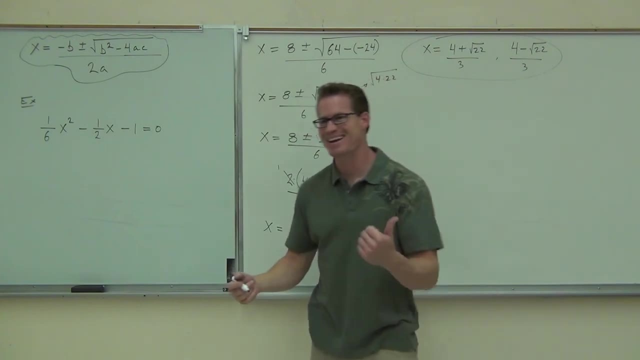 So, I'm going to go ahead and do this. I'm going to go ahead and do this. I'm going to go ahead and do this. Yeah. You get a triple whammy today. You get rain, you get fractions, and you get homework. What a Friday. Fraction Friday. You can't miss Fraction Friday. 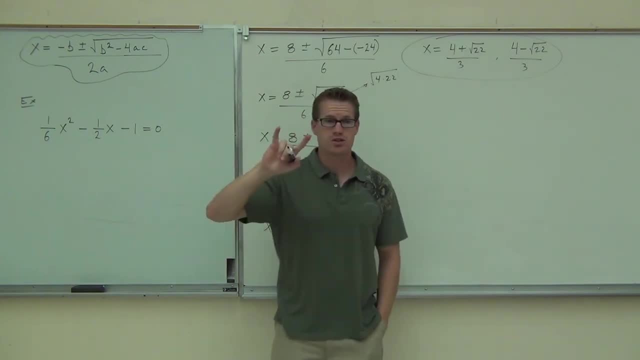 Oh my gosh. Hey, firstly, let's check a couple things. There's two things you can check. First thing is, is this all to one side and zero on the other side like I want it? Yes. OK. Yeah, that's true. Is it in the correct order, which means x squared x number? 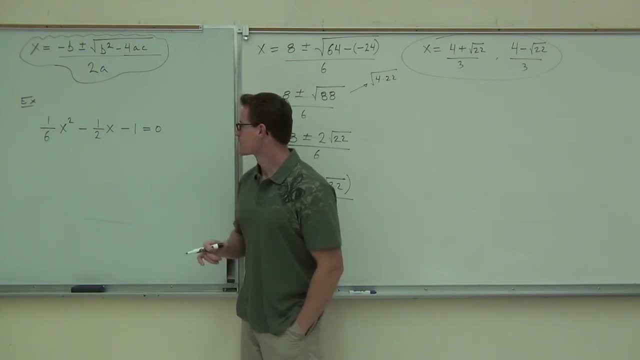 Yes. That's how you need to have it to find a, b, and c. How much is your a? 8. 8. 8. How much is your b? 1 6. How much is your b? 2 and a half. How much is your c? 2 and a half. 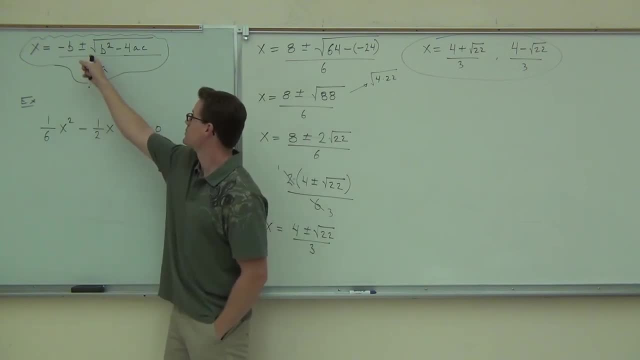 So, could I take these numbers, what's important, could I take these numbers and plug them into this? Yes. 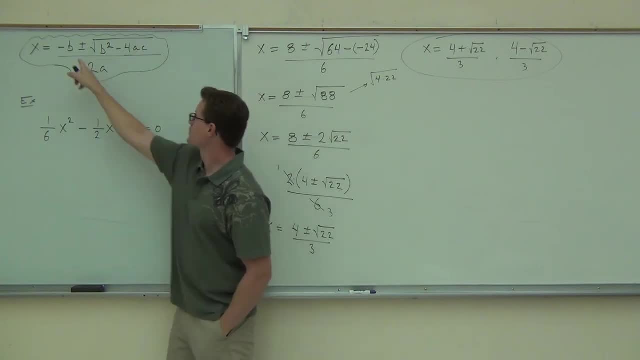 1 6 would go there and there. One, negative 1 half would go here and here. 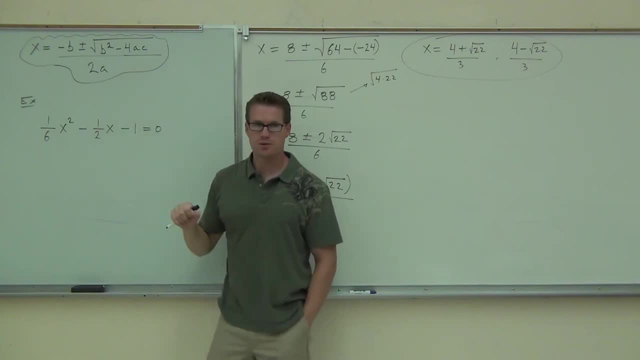 I would be getting 1 fourth out of that. And then, negative 1 would be going there, true? Mm-hmm. Do you want to do that? No. Shake your head. No. Do you ever want to work with fractions? No. No. Is this an equation? Yes. Oh, yeah. What can you do with equations? Chapter 7. Chapter 7. What can you do with equations? 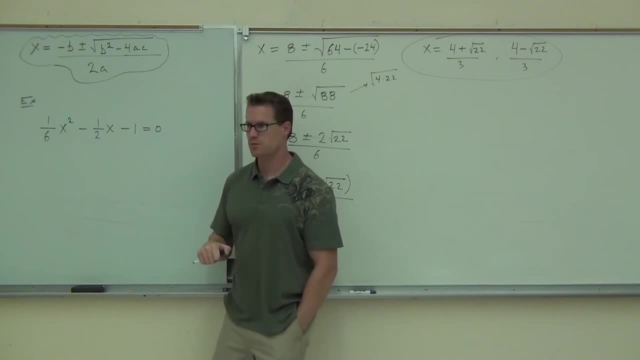 Can you always get rid of a fraction with equations? Yes. Oh, my gosh, then do that. Listen, listen carefully. 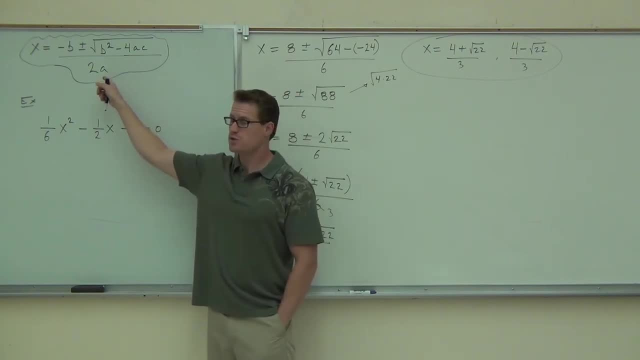 If you plug fractions into this thing, two things are going to happen. You're going to get it wrong or you're going to spend a tremendous amount of time doing this to get the right answer. Okay, a tremendous amount of time. Because you're dealing with fractions, folks. You'd have 1 half here on the top of it. You'd have a complex fraction. You'd have to work with that. Do you want to work with that? No, no, you don't want to do that. 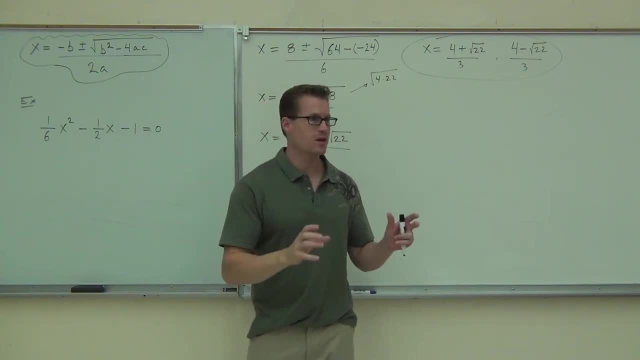 You'd be finding common denominators all day long and manipulating this to get the correct thing. 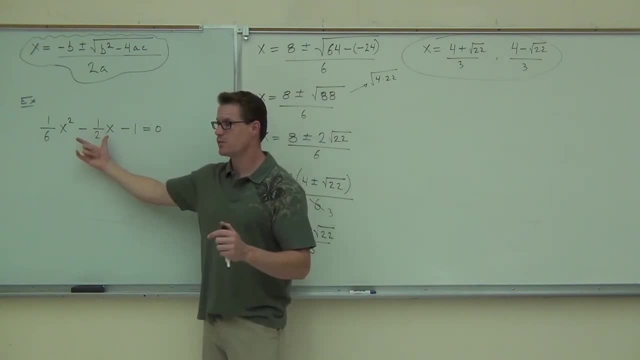 When we're going to be able to solve this first, well, not solve it, but we're going to be able to get rid of those fractions first and then have something very simple to deal with. 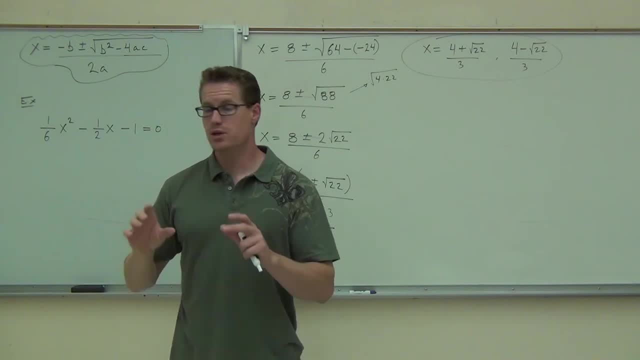 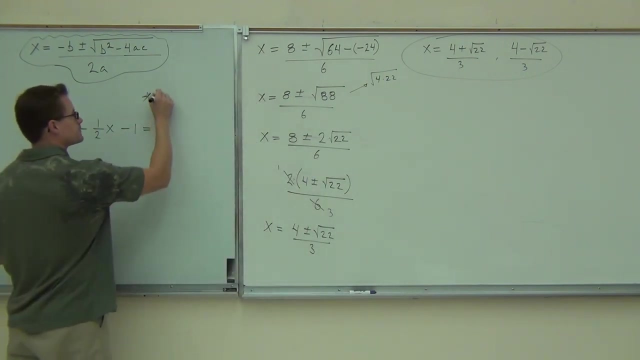 You with me on that? So the first thing I need you to do when you get a problem like this on your test, which you will have, it can be either very easy or very hard. If you don't clear the fractions, it's very hard. If you clear the fractions first, it's very easy. So first thing. Eliminate fractions. 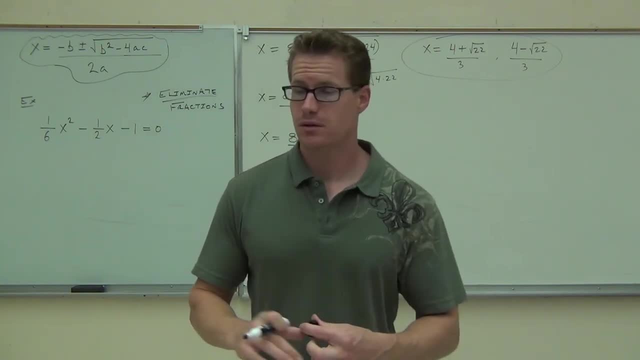 Okay, how do I eliminate fractions? LCD. So I need that. Can you find the LCD? It includes all my denominators. 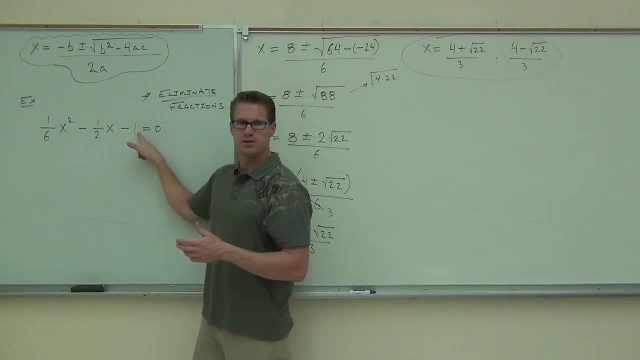 How much is it? Is that a denominator? 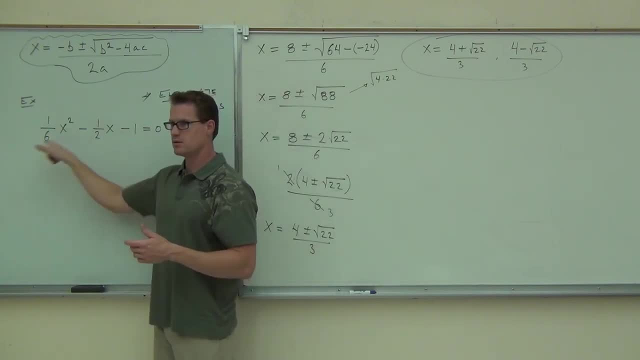 So even were this a 4, would it pay, would it be, would it be part of this? No. 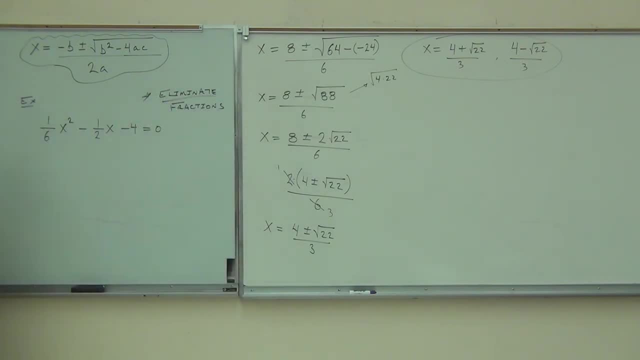 If this was like a, a 4, or if this, how about this, how about this, if this was a 5, would it change my LCD? No. 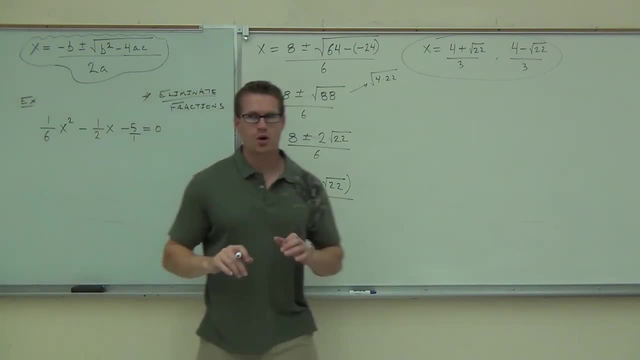 No, because this is like 5 over 1. Right? So don't let that confuse you. 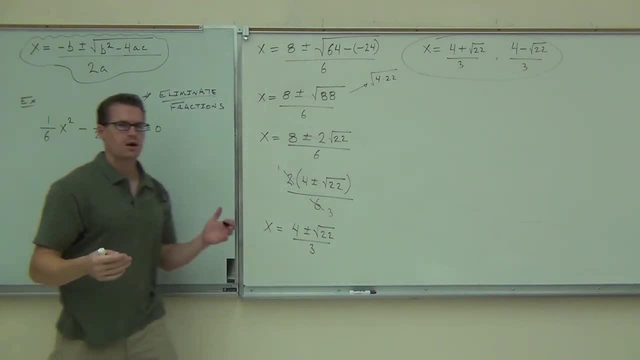 If this is a whole number, no problem. It's like a whole number over 1. That plays no part in your LCD. You're just looking at the denominators here. 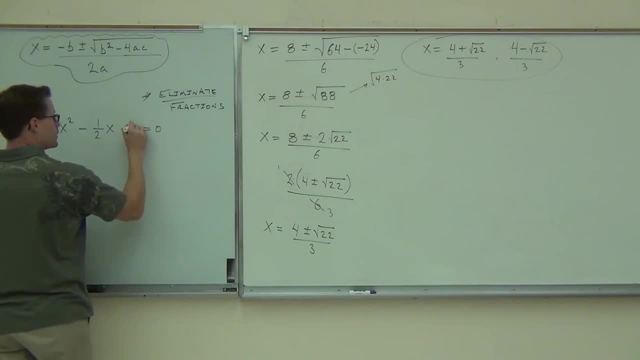 Just add denominators. Now, this was, if this was 1 over 5, would that be a part of your LCD? Yes. 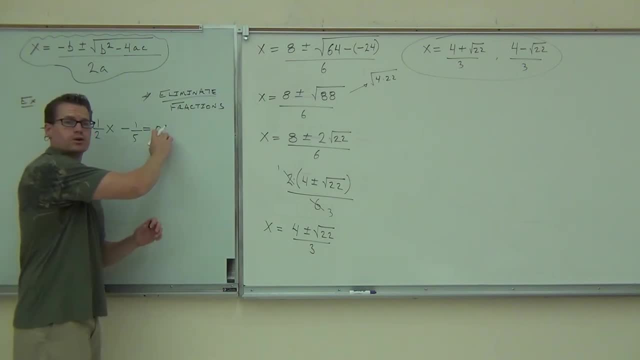 Absolutely. If you had a number over here, well, you won't, because you're going to put it in the proper form first, aren't you? 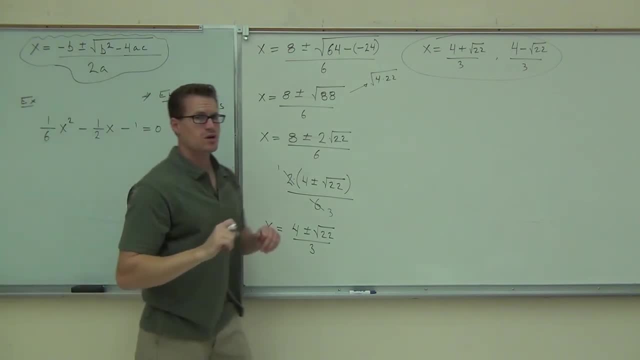 Okay, good. So, with that in mind, how much is your LCD, please? Six. Good, six. 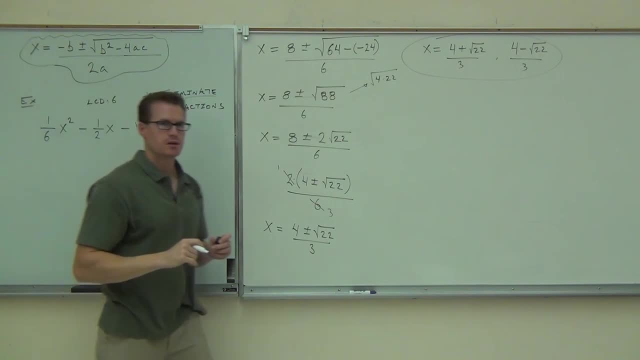 Yeah, we don't need 12, do we? We just need 6. Don't make it worse than it is. 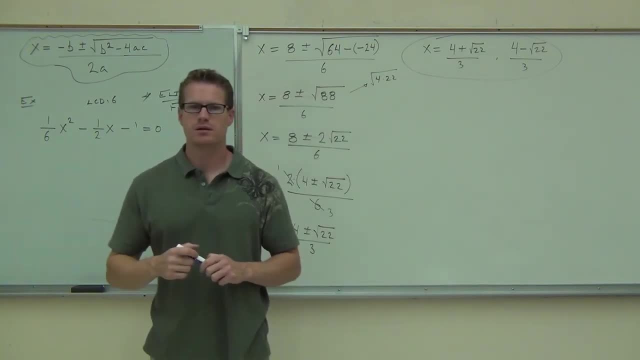 So take that, what do you do with that 6? Multiply it by how many things? One thing, two things? One thing, three thing, four thing? Two. Just two? Three. Three. 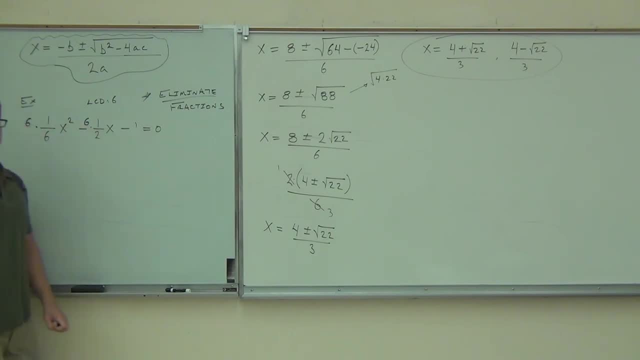 If I multiply, look at the board. If I multiply it here and here, does that work? 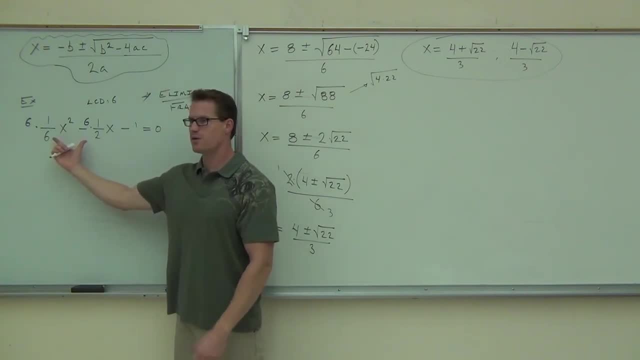 No. Notice how I've multiplied two terms, I've left out the rest of my equation. What else do I need to multiply it by? By my little one. 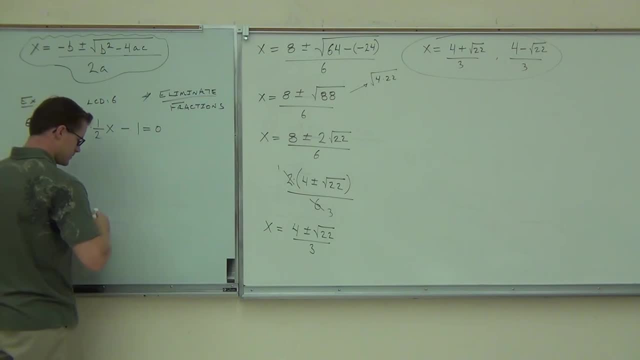 By my little one. Okay. I don't like 666. 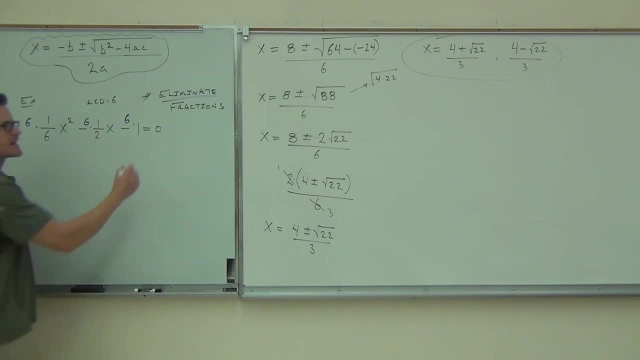 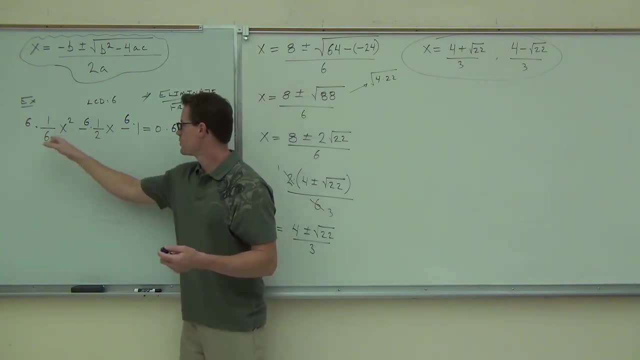 Because this is an equation, and when you multiply one side you have to multiply the other side. Now, fortunately for us, how much is this going to be? Zero. Zero. Don't make the mistake and put six. Please don't do that. Zero times anything is zero, all right? 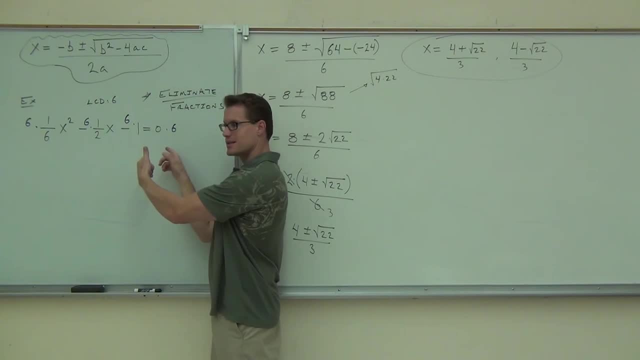 So, yes, you are multiplying this. But if you do this correctly, everything's on one side anyway, this is still going to be zero. Yes, no Everybody yeah So that's gonna be zero how much is this going to be? 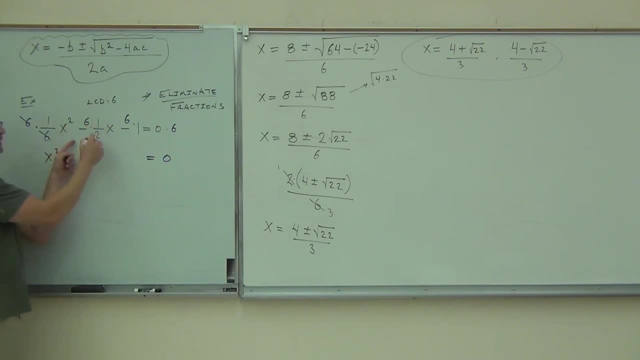 Perfect x squared is this going to simplify yeah, it has two years in the LCD that's going to be minus what? 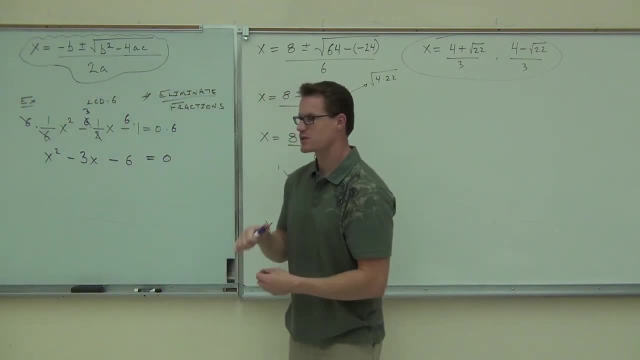 Hey, does that look a lot better? Oh my gosh, that's so much better That's way way better 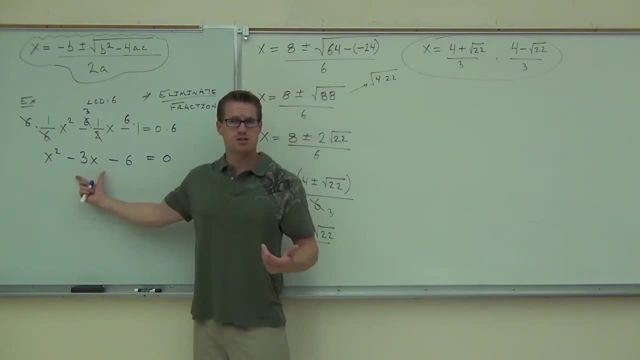 You can even try it that you can't factor this you'd spend 10 seconds doing it you have negative 3 negative 6 you try to Factor 1 2 3 5 7 8 10 you can't do it then use quadratic formula So that's the idea here. You don't want to do completing the square. That's an odd number 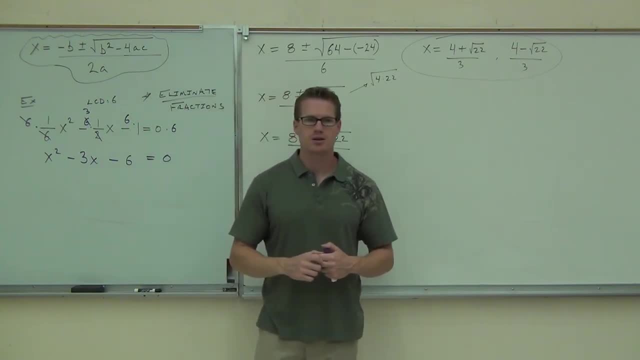 So do the quadratic formula find your a your B and your C formula real quick? This is lesson. We'll actually do all the way together 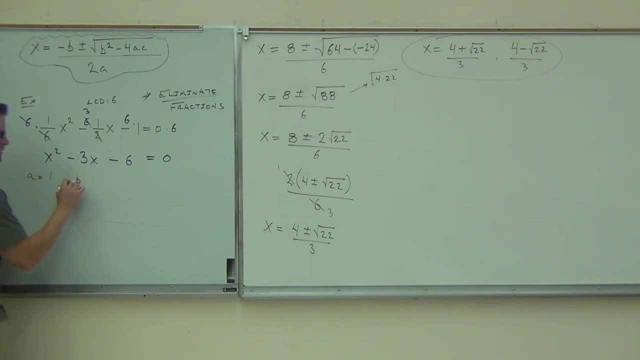 How much is your a how much is your B? I'm glad you got the a the a is not 0 the a is 1 and C is So we're going to plug this in we'll get x equals negative 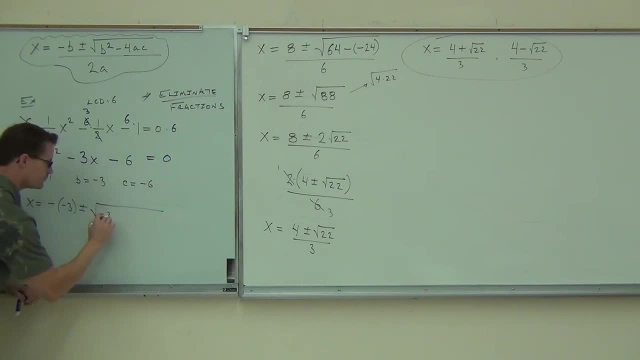 B plus or minus the square root of B square minus 4 times a Times C all over 2 times a 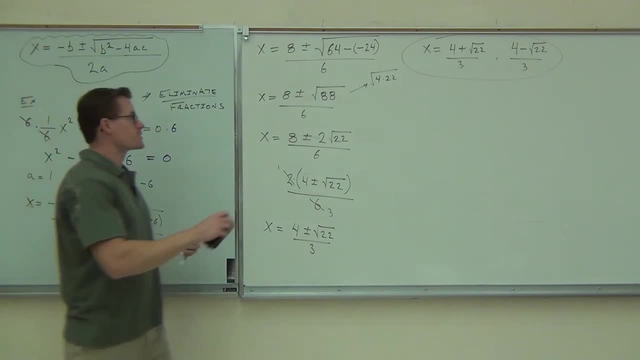 So negative negative 3 plus or minus negative 3 squared minus 4 times 1 times negative 6 all over 2 times 1 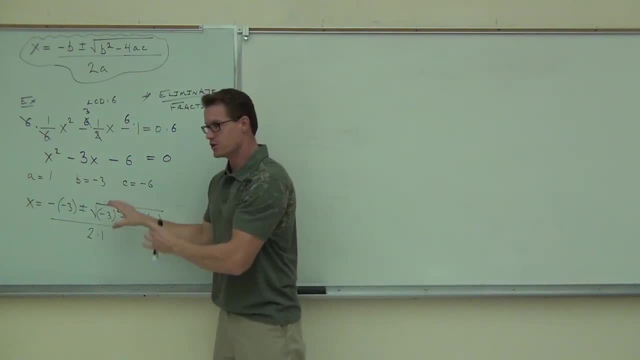 If you show me that at least I know you know what you're doing right if you get that far you do know what you're Doing after that would be a math error 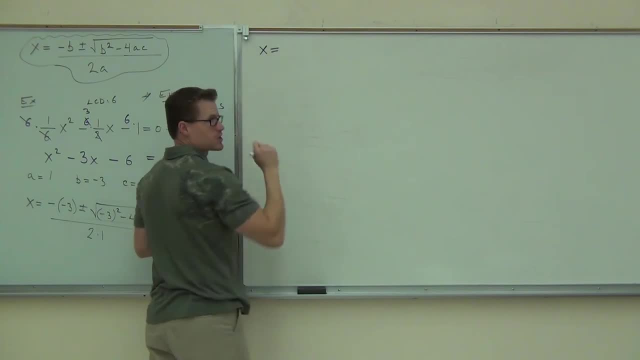 But basically back there, so we're going to do this. What's the first thing? I'm gonna write ladies and gentlemen Let's go quickly. We should have no ideas at this point how much 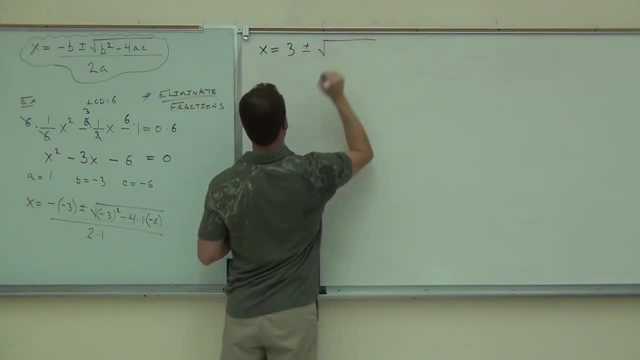 and then Sure inside my radical the first thing gives me nine minus What? Minus negative 24 very good All over 2 times 1 gives you 2 You still okay so far 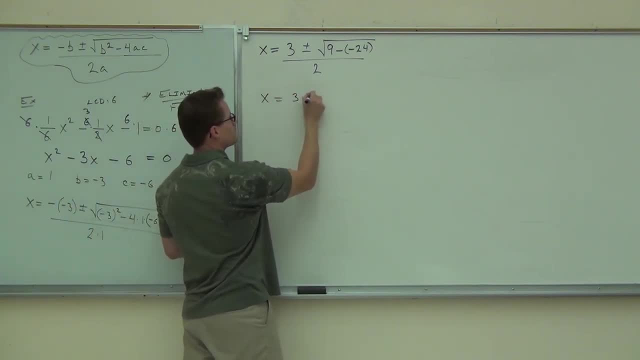 Okay, so we're going to have x equals 3 plus or minus the square root. What's inside my square root at this point? 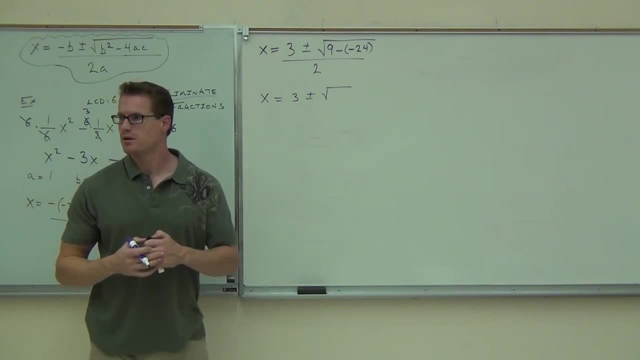 Am I subtracting should have a negative or should have a positive how much over 2 Now at this point 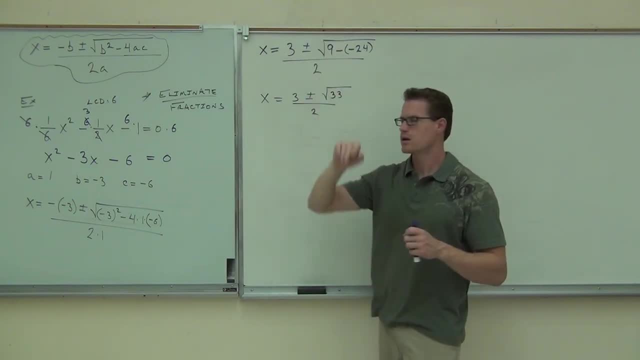 Firstly how many people feel okay getting down to that far? Good for you at this point you try to simplify that can you simplify that now it's 3 times 11. That's 2 primes. I can't do that 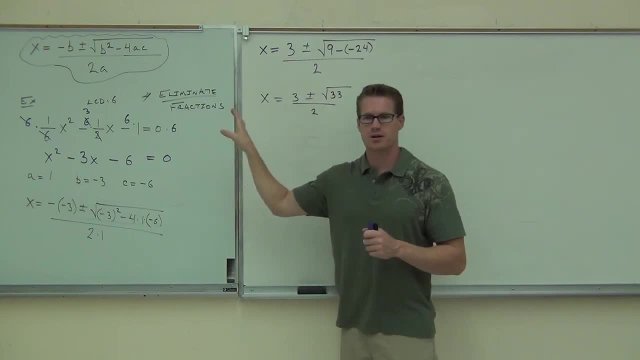 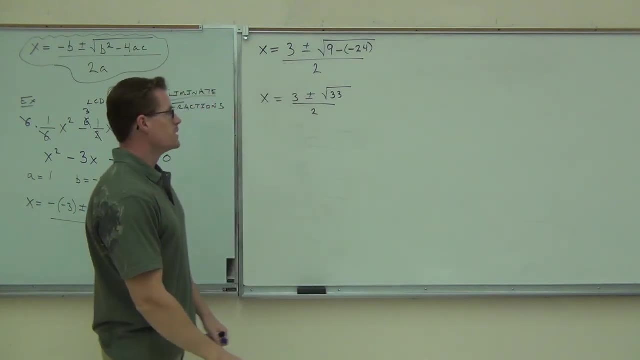 Can't simplify this can't factor anything out. You can't factor anything here. You cannot factor 3 this 3 is okay This one's inside the radical you can't do that. It's gonna be outside the radical to factor so in this point 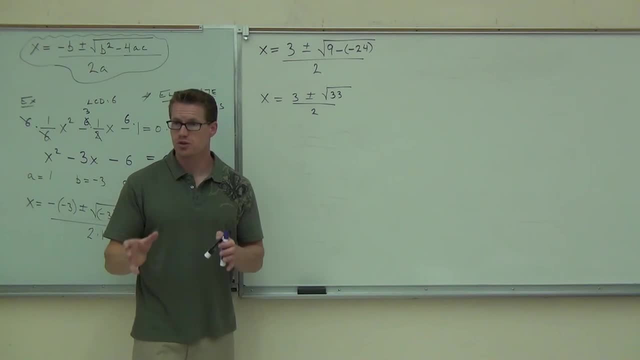 Well, well, this is kind of nice You're actually? Pretty much done. You just write your two solutions. Do you see your two solutions write them out your death? 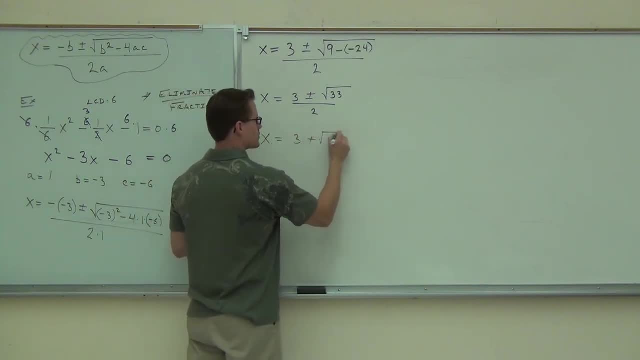 You've got x equals 3 plus square root 33 over 2 You get 3 minus square root of 33 over 2 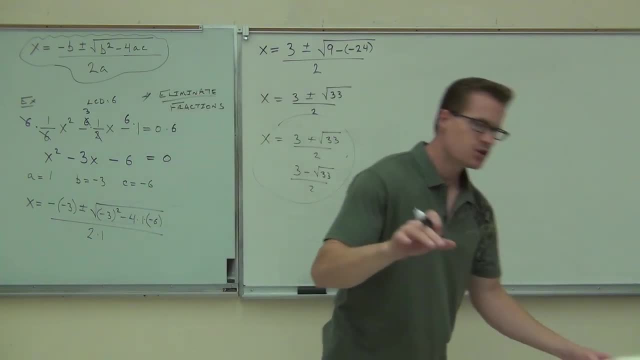 That's it I'd like you to do one of your own before you go any further Again you're going to have one very much like this on your test 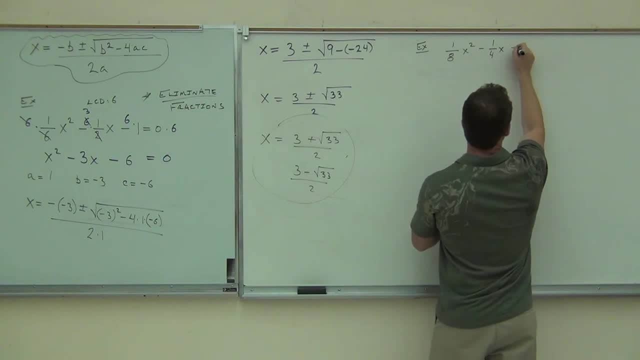 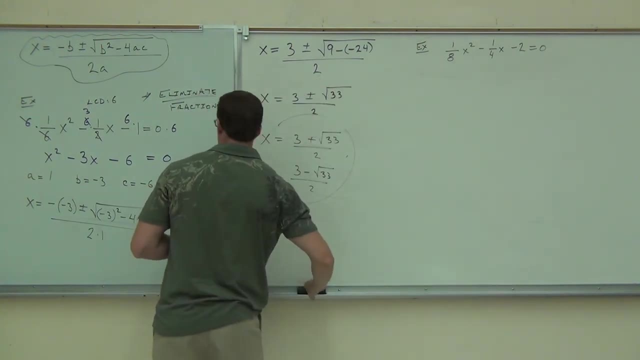 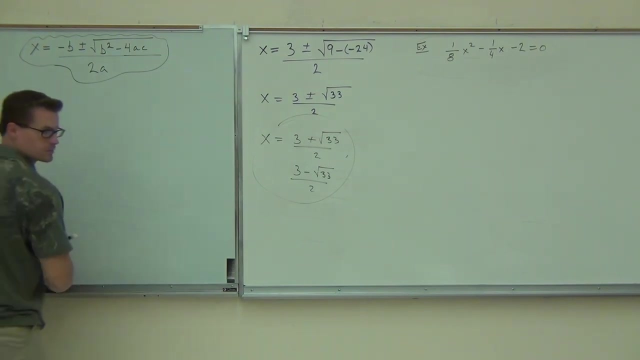 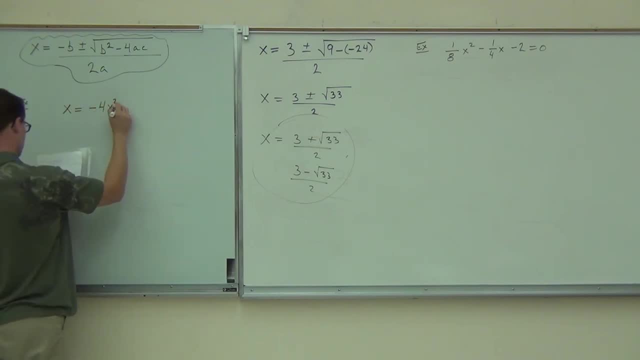 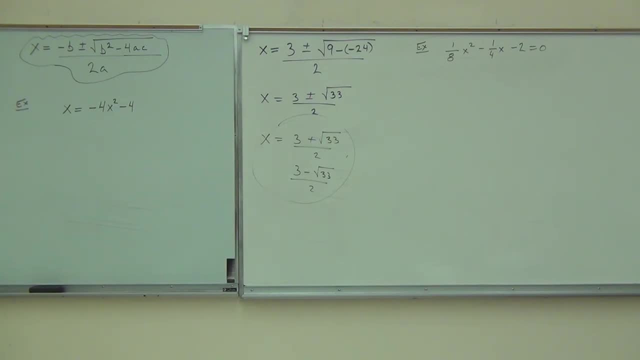 So we're making sure we have the correct form. That means that it goes x squared, x number. You're making sure that everything's on one side. 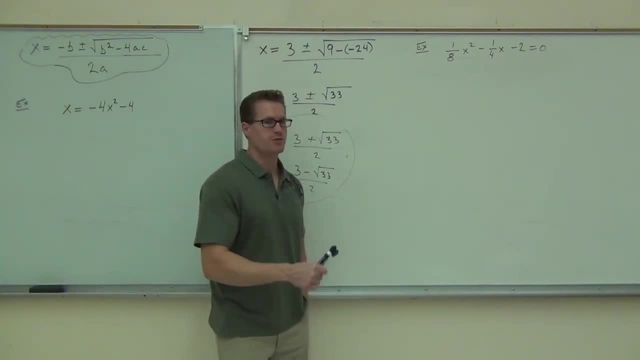 You need to have a zero somewhere on one side of the equation if you're going to use a quadratic formula. You have to have a zero. If not, it's not going to work. 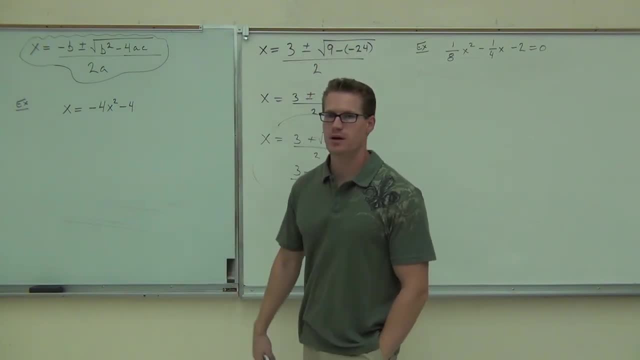 Next thing, should you ever plug in fractions to your quadratic formula? Never. Oh, never. Never. That'd be ridiculous. You have an equation here. 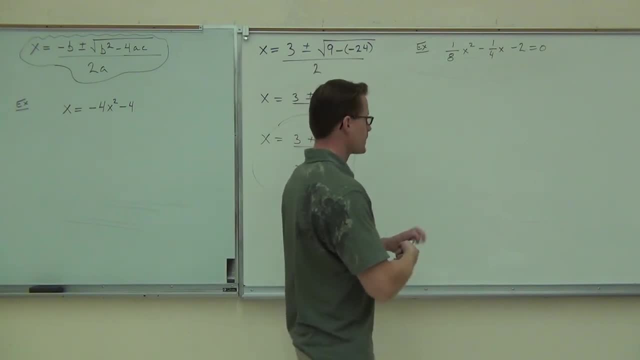 Get rid of your fractions first. Otherwise, it makes it way too hard. So in our case, we are trying to get rid of fractions. This is chapter seven stuff. What are you going to multiply by to get rid of your fractions? 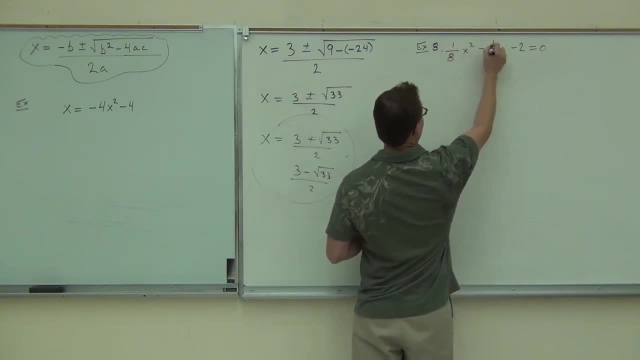 Eight. Good. So here, multiply by eight. And here by eight. How about the two? Yes, two. And here? Yes. 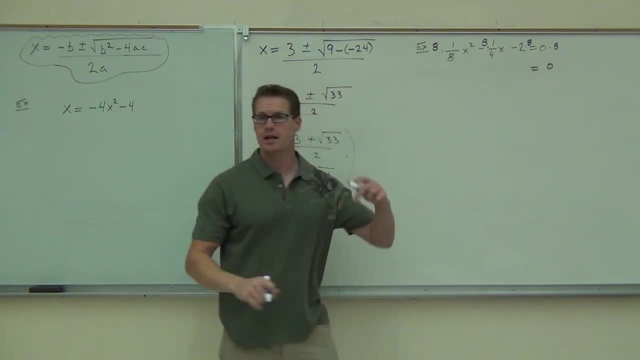 Yeah, technically, yes. Now, fortunately for us, that's a zero. Zero times anything is zero, not eight. So we have zero on one side of our equation. Here, you get, nicely. 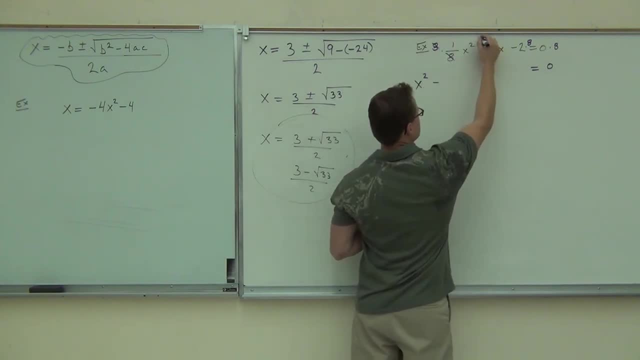 X squared minus 2x minus 16 gives you zero. 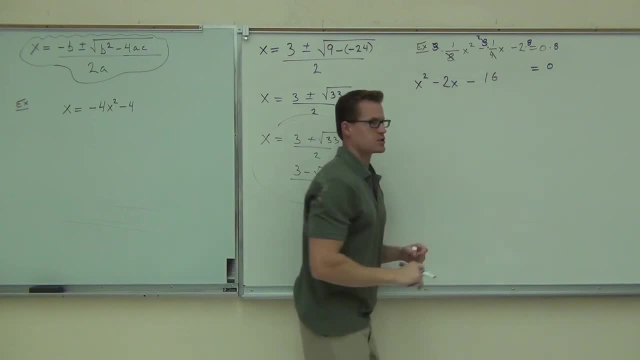 How many of you were able to make it that far? Good for you. Now, in normal situations, well, this is, of course, a quadratic formula section. So you're probably going to be using that. But most of the time, you're going to check to see if you can factor that. You would check that. You'd have negative two on the top, negative 16 on the bottom. 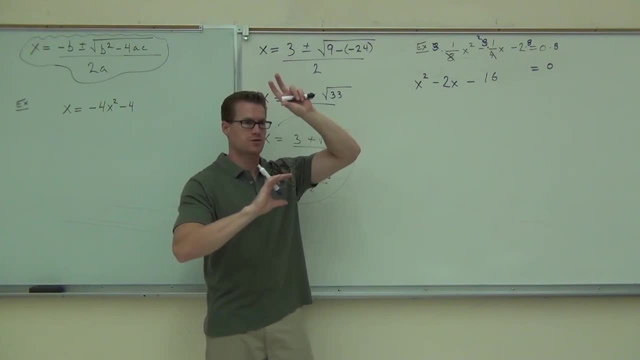 I'm not seeing anything that I can factor out of that to use for adding to negative two and multiplying to negative 16. I don't see it. 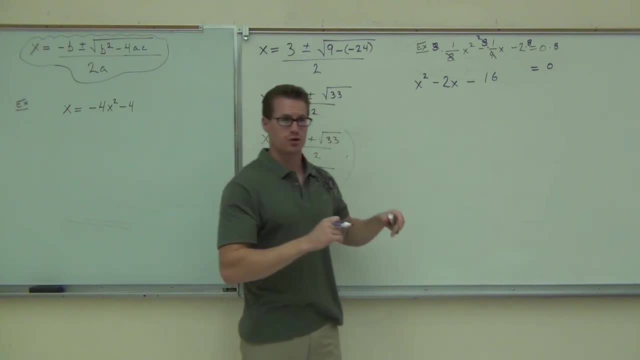 But I'd try for 10 seconds. If you can't do it, then you move on to quadratic formula. 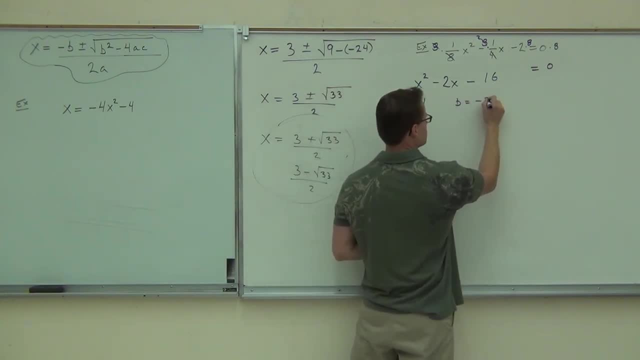 A is? One. B is negative two. And C is negative 16. Did you make it that far, folks? Yes. Good deal. 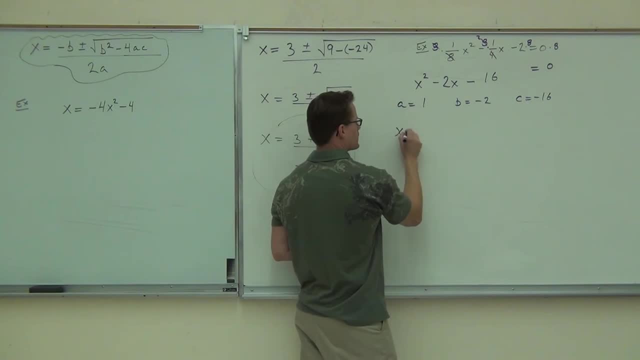 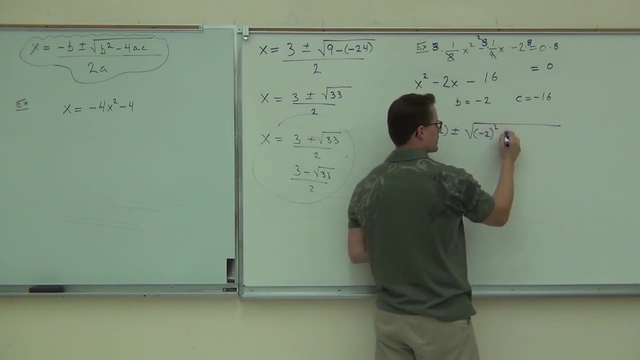 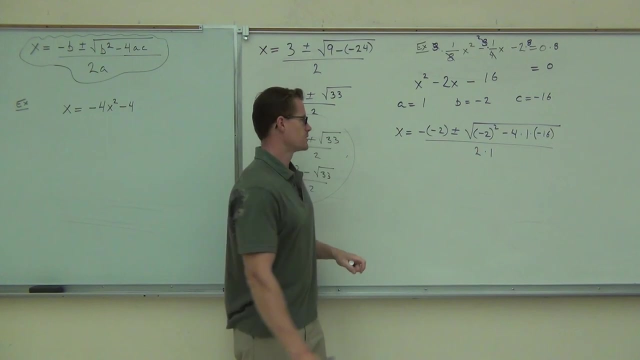 Now we're going to plug it in appropriately. We're going to have X equals negative negative two plus or minus the square root of negative two in parentheses squared minus four times A times C. All over two times A. Check your work against my work. Do you have exactly that on your paper? OK. 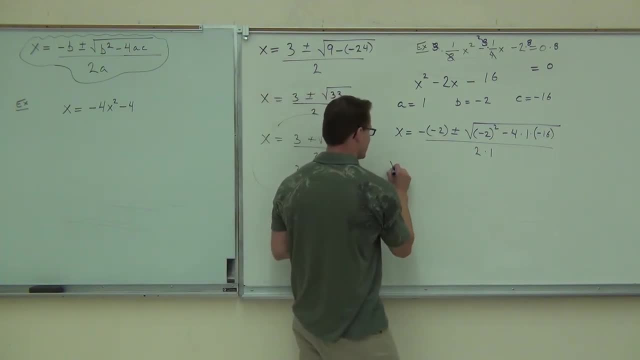 Hopefully we both did it right. So negative negative two, well, that's two. Plus or minus the square root of negative two squared is positive four minus, you're going to do four times 16. That gives you 64. All over two. 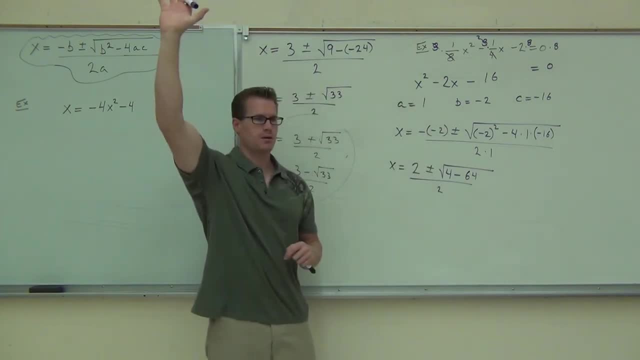 Raise your hand if you made it that far. What? OK. I hope not. That far? Yeah. OK. With parentheses? Yes. Fantastic. It's even better. You just automatically raise your hand. Don't you know? There you go. Four minus negative 64. True? 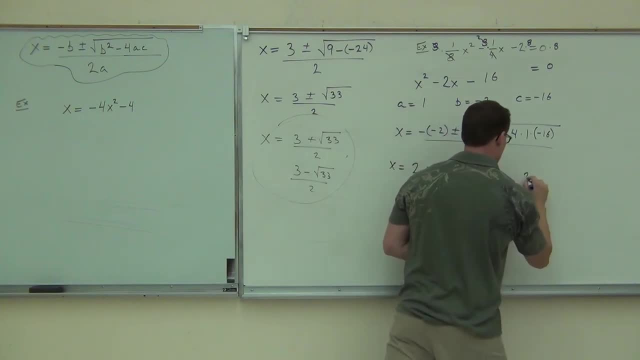 Yeah. OK. Well, that's going to give us two plus or minus the square root of, how much is inside my ? 60. 60. Yeah. OK. All right. 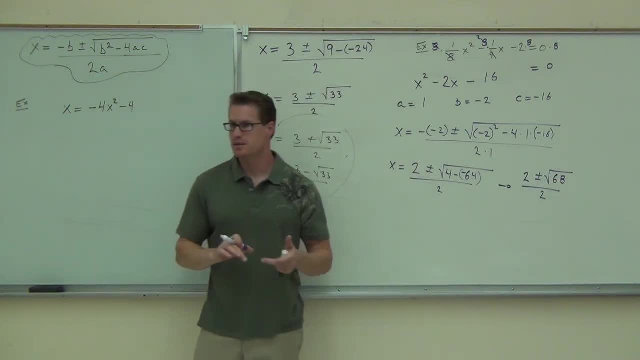 So can I break up, can I simplify the square root of 68? Yeah. Four and 17. Four and, so you try to divide by a perfect square. The only one that works here is four. 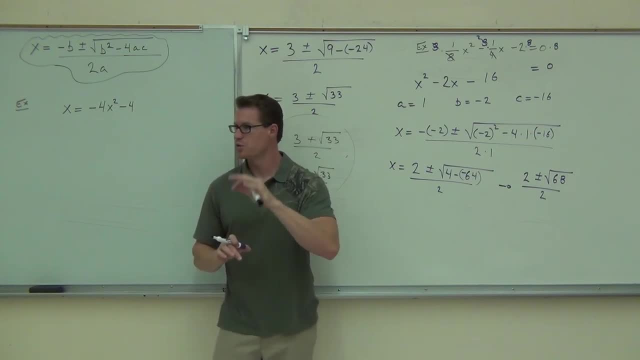 So you're going to do the four times the 17 or you're going to get two root 17. Did you get two root 17? Yes. If not, well, work on your simplification. 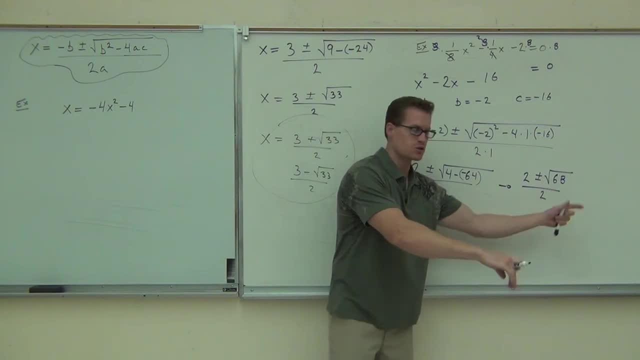 If you made it this far, you should be able to make it down to simplification. So this is two plus or minus two root 17 over 64. 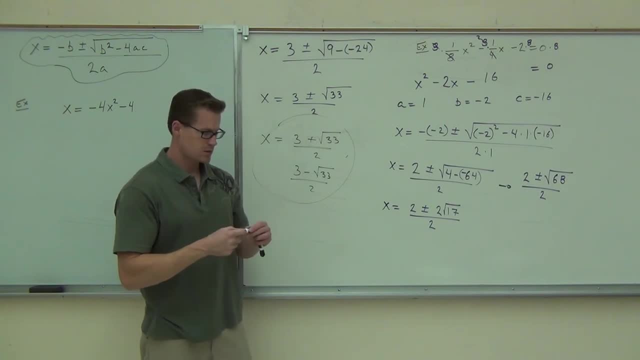 Two over two. Right side of the room. Can you go any further? Yes. What can you do? Factor. Factor how much? Two. Notice. 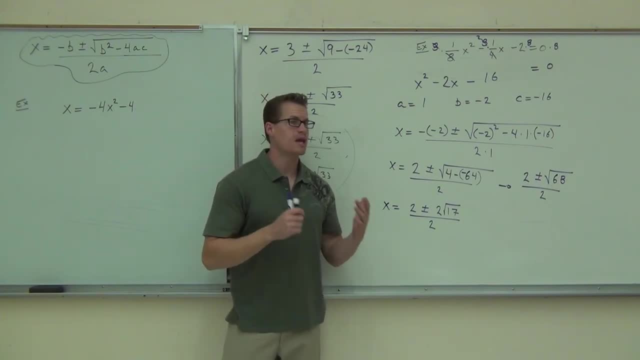 Please watch up here. What you can't do, this is one of the most common mistakes. I see it in calculus. What you can't do, if you're not watching, you're going to make this mistake. You can't do that. You can't do that. That's connected by addition and subtraction. It's a double whammy. You're double messing this up. And two negatives don't make a real difference. So you can't do that. You can't do that. That's connected by addition and subtraction. It's a double whammy. You're double messing this up. 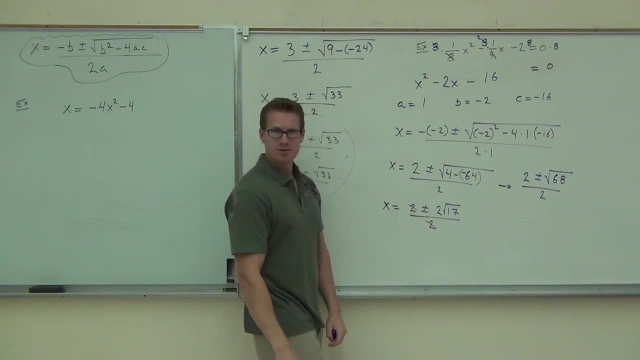 And two negatives don't make a real right here. You can't do this at all. 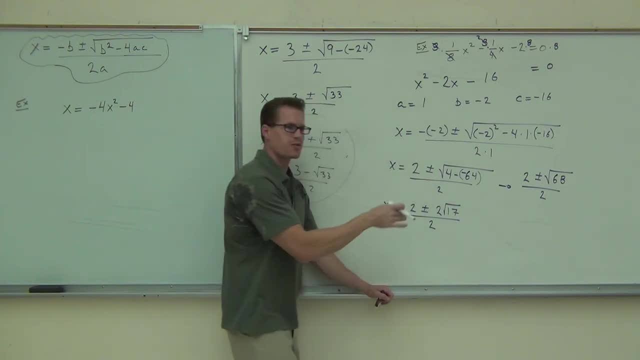 Factor the two out? You have to factor. In order to simplify, you have to factor. 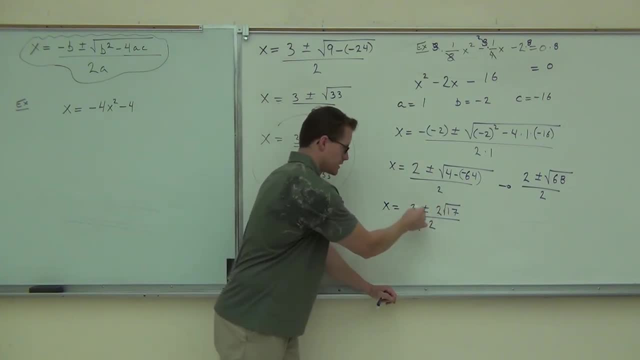 You have to. You can't cross these two out either by subtraction. 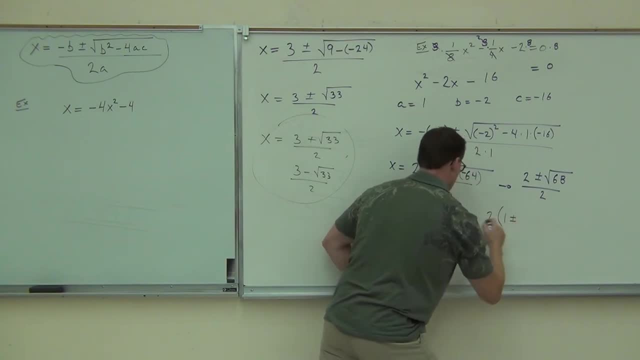 So you have to do one plus or minus the square root of 17. Notice the difference. 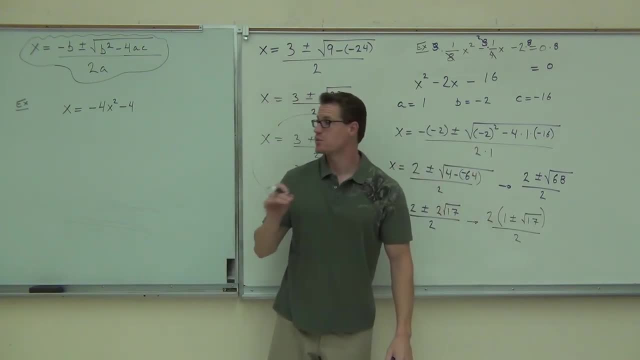 Now, that's been multiplied. by the entire expression, that's what you can simplify. 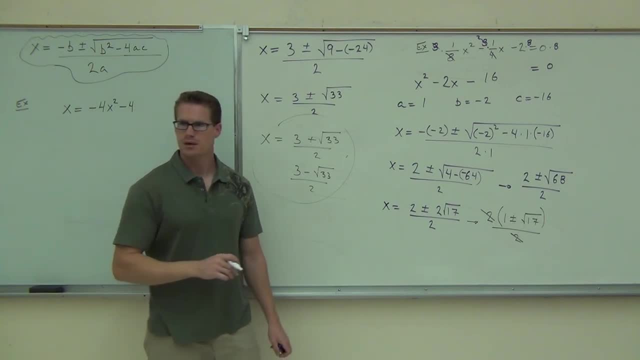 Those are now gone. What's on the denominator of a fraction? One. Do you need to write the one? No. 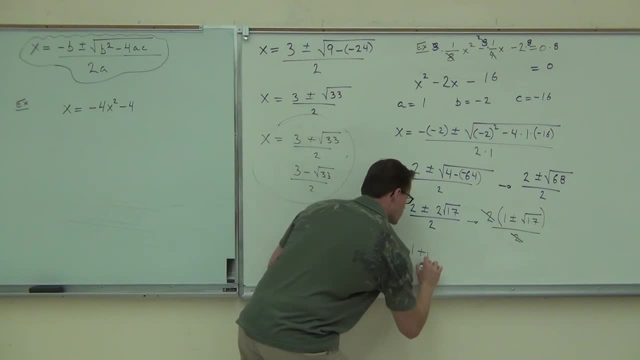 Not really. You've got one plus the square root of 17. You've got one minus the square root of 17. 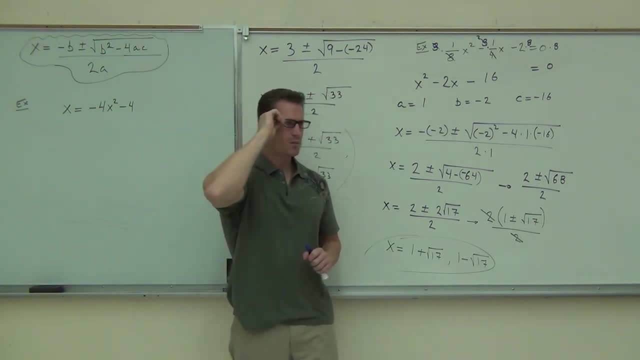 Would you raise your hand if you feel okay with this problem? Now I'm gonna take a moment right now to talk about what we're doing. Because a lot of times people can do the math, they just don't understand exactly what we are doing here. 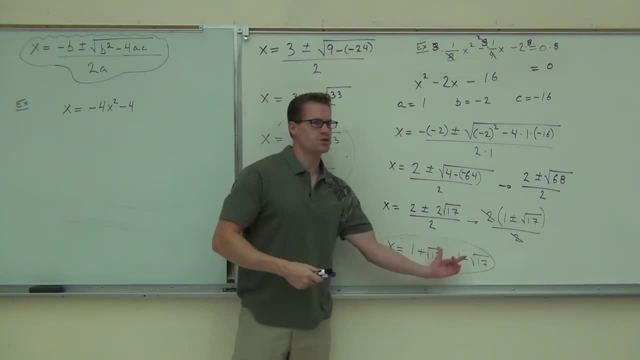 What you're doing, when you're finding these two solutions, you're identifying part of a graph. 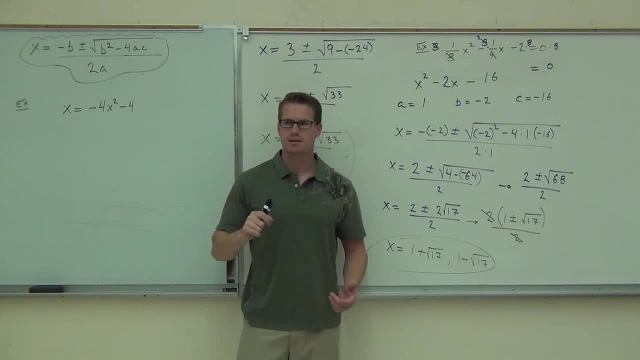 Do you understand what type of graph an x squared makes? Parabola. Parabola. Do you remember the parabola? No. The u-shaped graph? 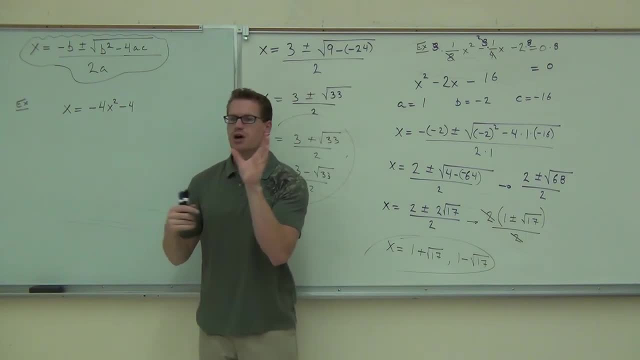 What you're doing when you're finding this, when you're finding these two solutions, you're finding out where that graph crosses the x-axis. Where that graph crosses the x-axis. 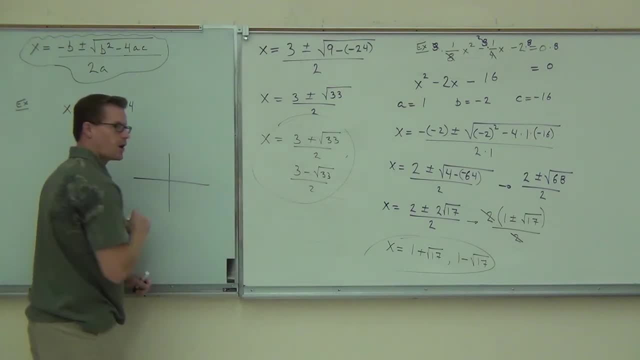 So, the options you have, are you can, how many spots are you normally gonna cross the x-axis at with a parabola? Well if you go down, you have to come up somewhere, right? And it's not gonna go back down, it's gonna go up. Or if you're upside down, you're gonna cross the two spots. That's what you're doing when you're finding two solutions. You're finding where, according to the x-axis you're crossing. Here and here. Or here and here. Are you with me on that? 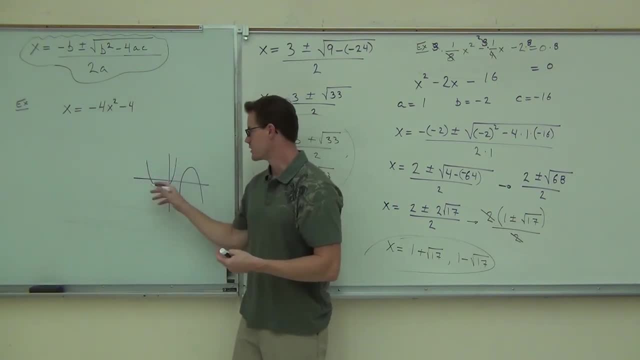 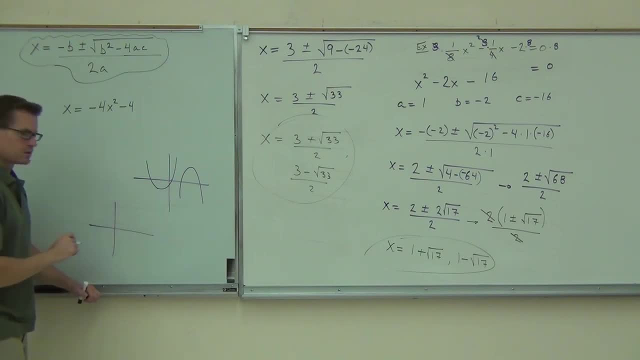 Now there are a couple more options. Could you not cross at all? Yes. That doesn't cross at all. Yet, we're still gonna get two solutions. However, you know what's gonna happen. I hope you're listening here. 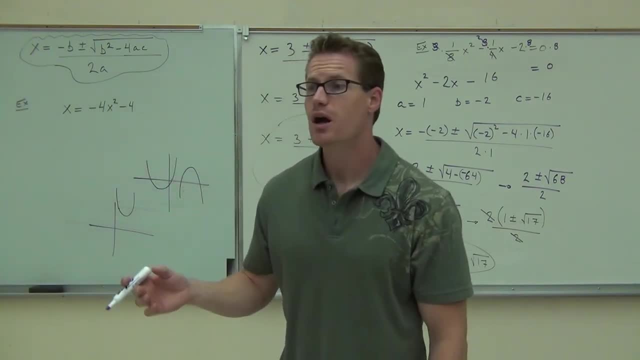 You're gonna get complex numbers. Complex numbers means you don't cross at all. It means you have two solutions, there's not real solutions. This would be two real solutions. This would be two complex solutions. Or that one. Is there ever a case where you can get one? Yes. 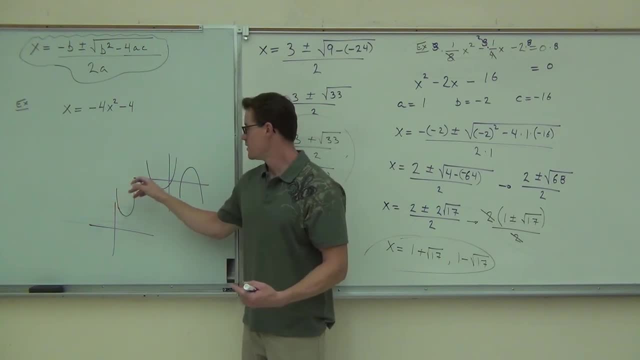 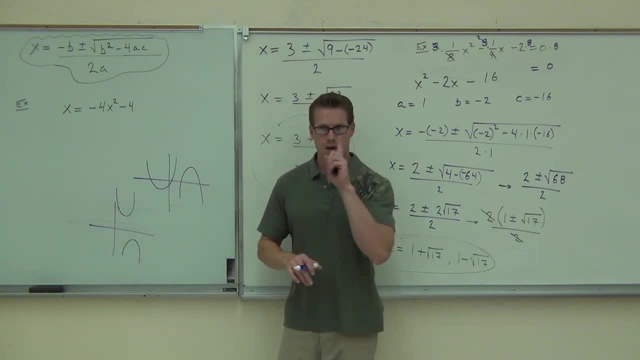 Yeah. Yeah. Yeah. Yeah. Yeah. Yeah. Yeah. There's not really one. You cross it, but you don't come back up. 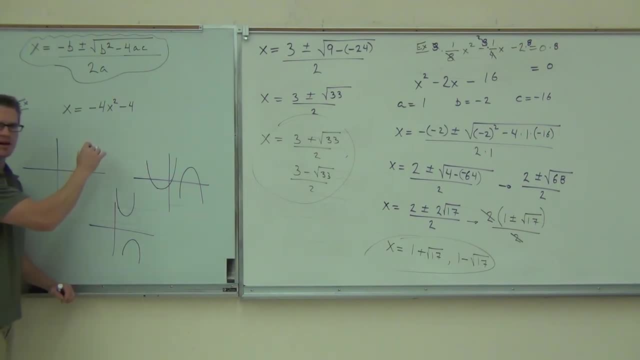 Is that possible? What is there another case? Is there another option for you? Yeah. Side bended. Not a side. You can't do that. That's not a function. Where? 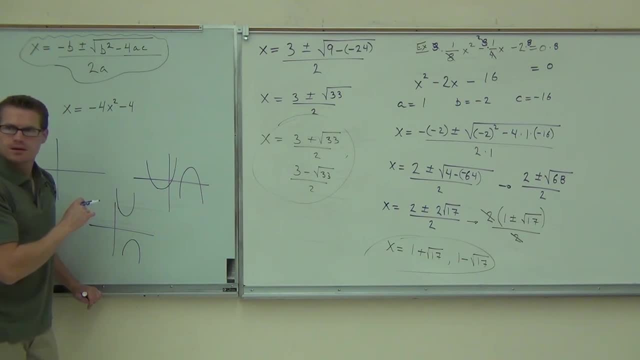 At the position of the bottom? Can you possibly touch this at one point? Yeah. 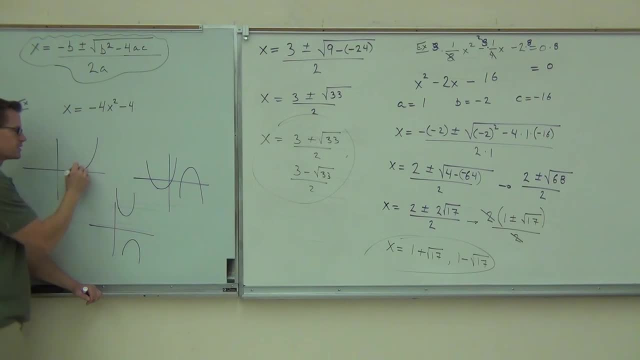 What if this is resting right on it? Does that hit it at one point? Yeah. 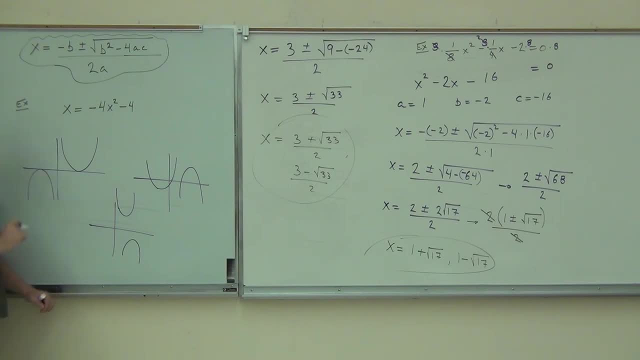 Or upside down. Therefore you have three options. You have the option where you cross it twice, those are two reals. You have the option where you don't cross it at all, two complex. You also have the option where you touch it at one spot, the vertex is on that graph. This is called a double root. 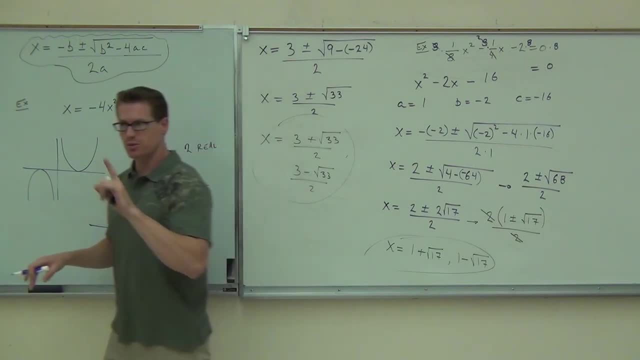 It's technically two real roots, they just happen at the same point. So we're going to say this is one real. 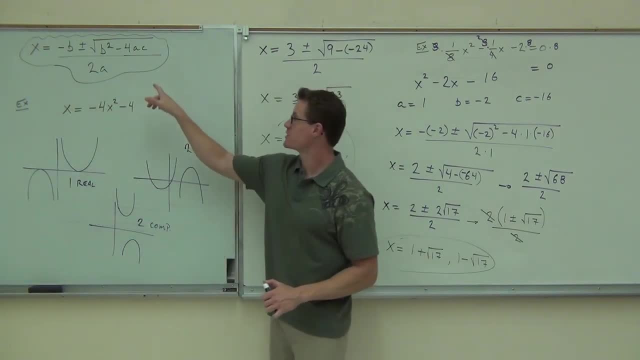 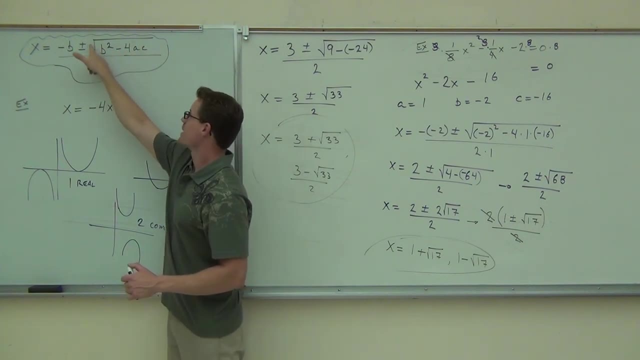 Now we're going to talk about the discriminant and what gives you these things. So look up at the discriminant. Hey, if this is, look at the board with me please, if this is positive, that means you're 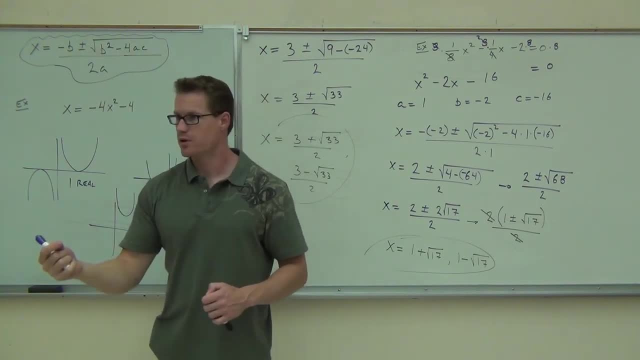 adding and subtracting some number, some real number. You with me? Some real number. 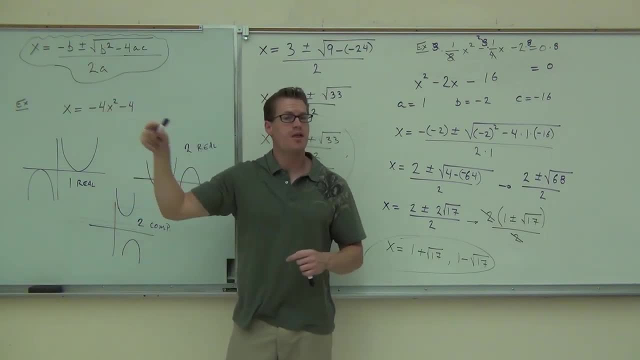 If you add and subtract a real number, you're going to get plus and minus a real number. 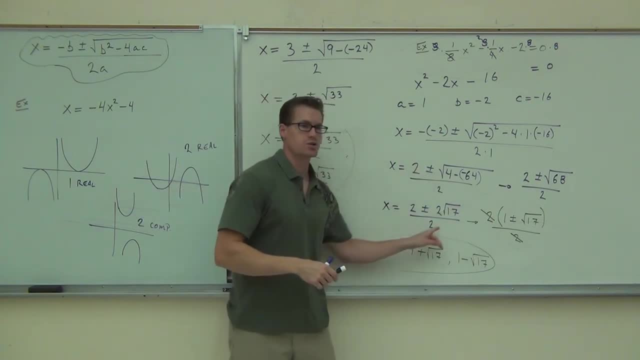 That gives you two real solutions. These things are real solutions. Follow? 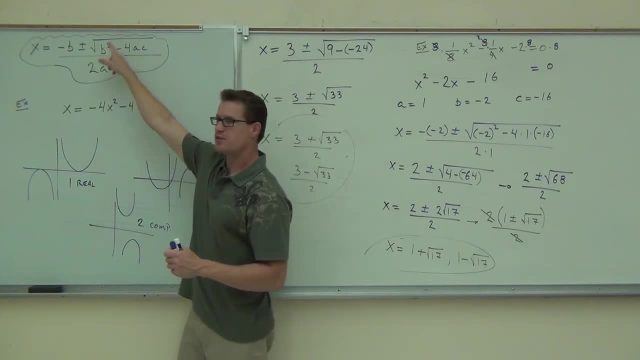 If this is negative, what's the square root of a negative number, what's it going to give you? I. The square root of a negative is I. That's going to give you two complex solutions, you're going to be adding and subtracting the complex. That would be this space. 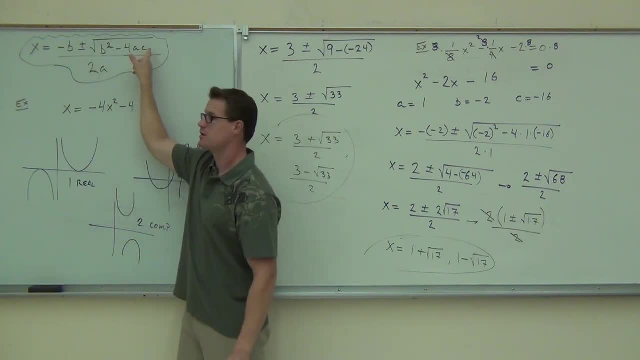 What's the only time you can get one solution? How much would this have to be? One. Remember, if you add and subtract a real, you get two reals. If you add and subtract a complex, you get two complex. What does this have to be to add and subtract it? You still get only one thing. Say it again. I heard someone say it. Zero. If you add and subtract nothing, you're just going to get one number. You're going to get just B, negative B over 2A. That would be your one solution. If this happens to be a zero. It does happen from time to time. Now, we're going to talk about one more example, this one. I'll show you what to do with it. We'll talk about how to apply it to one instance, and that will be our section. 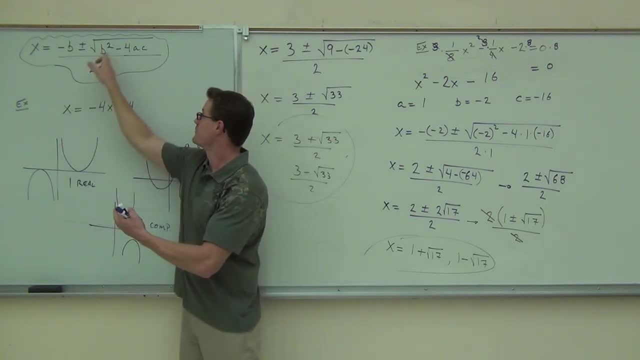 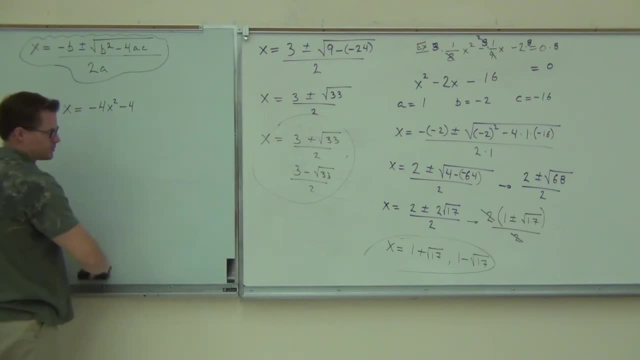 But you're going to have to deal with all negatives. That's going to suck. Otherwise, these over here. Add them. So, add 4B. 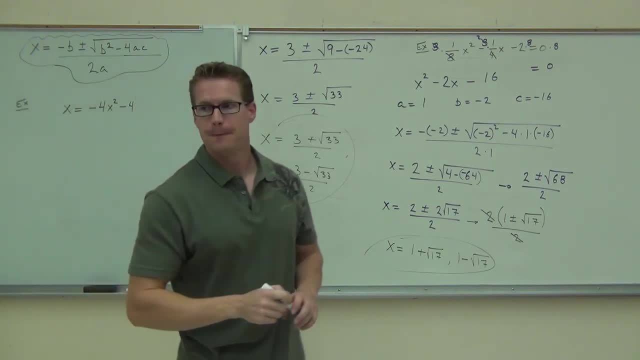 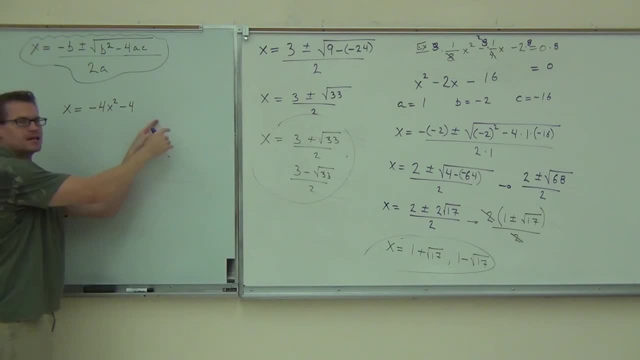 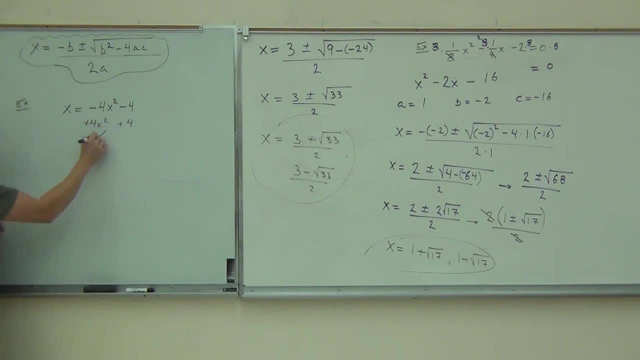 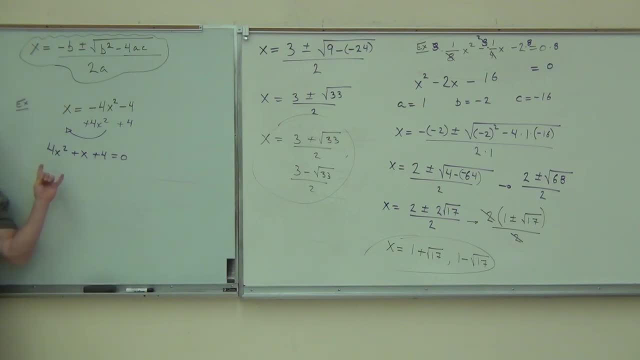 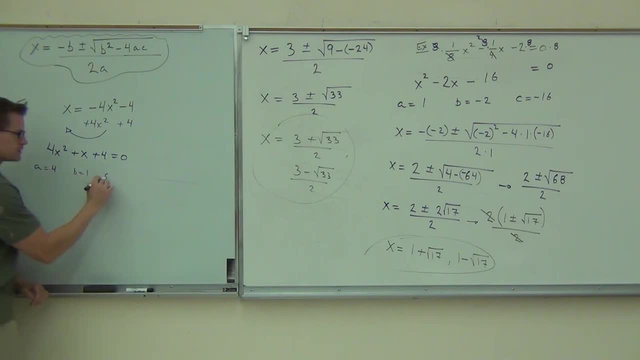 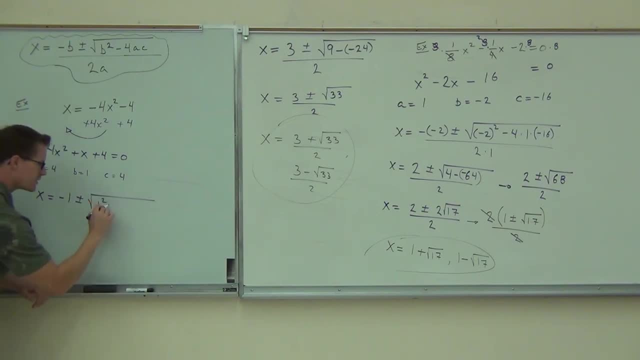 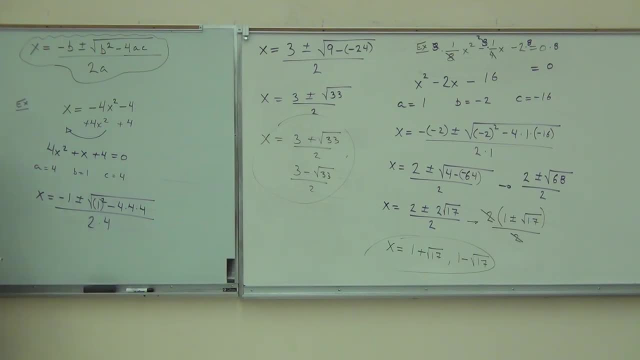 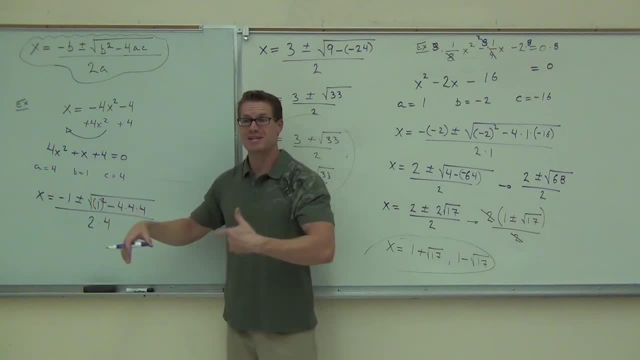 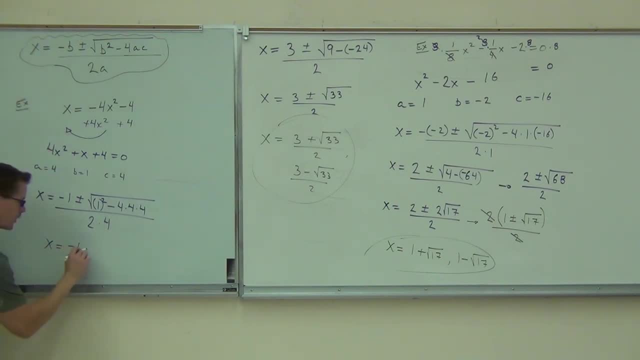 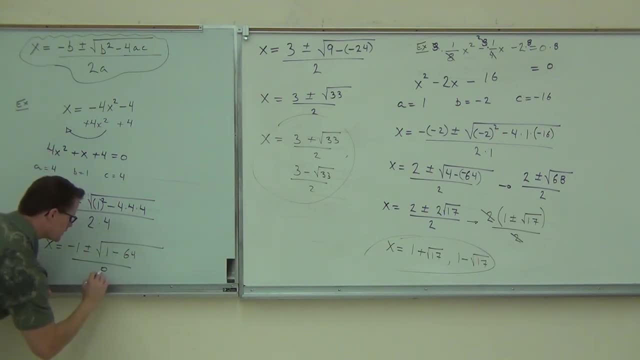 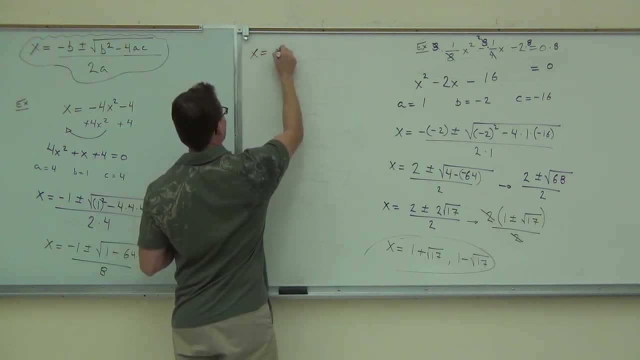 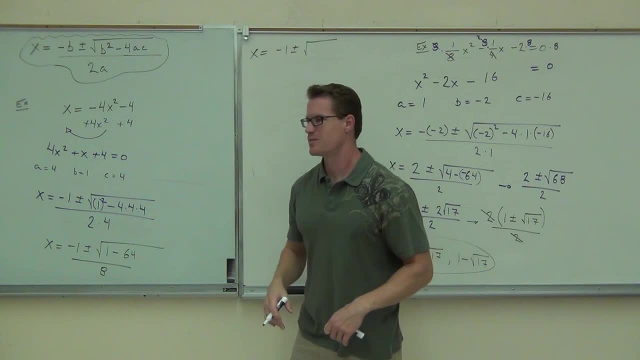 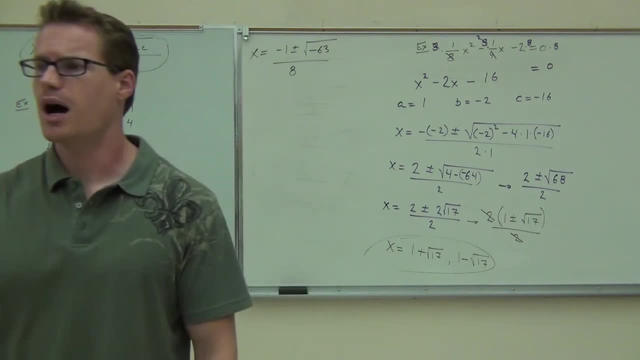 Now, the square root of negative 63 is something we should have focused on with our i's. 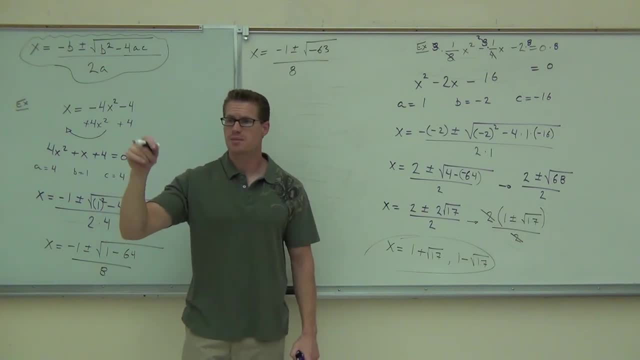 You know the negative gives you an i. 63 is 9 times 7, that's going to be 3i root 7. Are you with me? If not, work on that again. 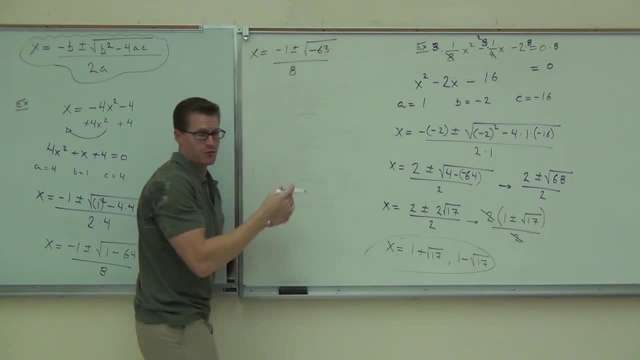 This is 3i root 7. Don't forget about your i. Remember, get your i's. You can't really see the problem, ha, ha, ha, ha. Too much? What do you use to sleep? It's Friday. 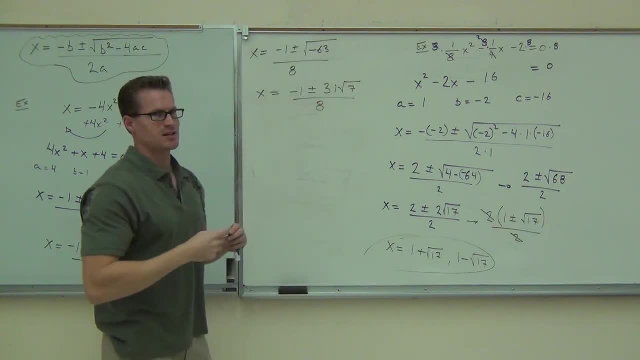 I actually had a drink this morning. Just kidding. 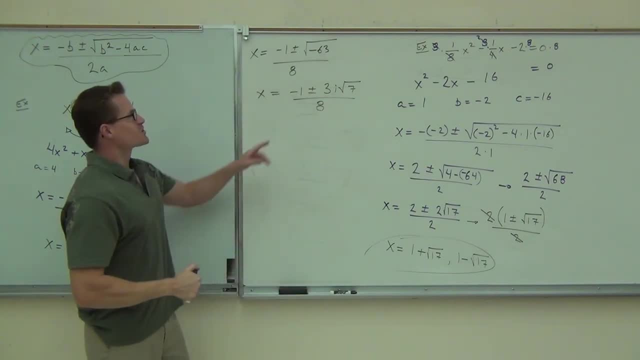 It is Friday. Coffee, I drank coffee this morning. 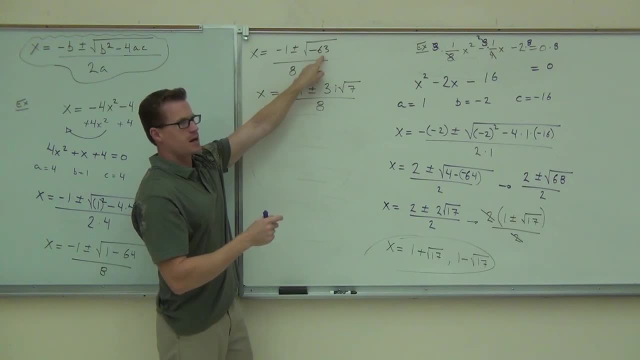 So this is the negative 1, that's our i. 9 times 7, that's 3 root 7. 3i root 7. You can't simplify any more than this. You're just going to write out your two solutions. 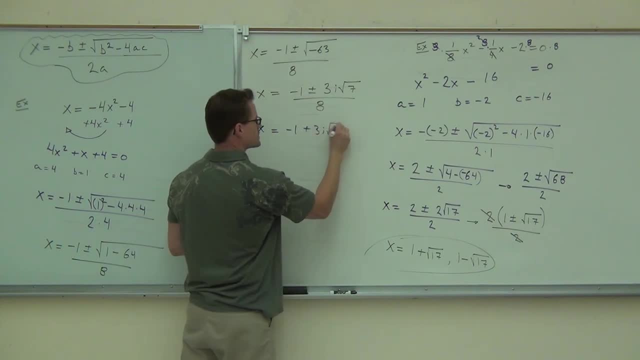 Negative 1 plus 3i. 3i root 7 over 8. Negative 1 minus 3i root 7 over 8. That's it. 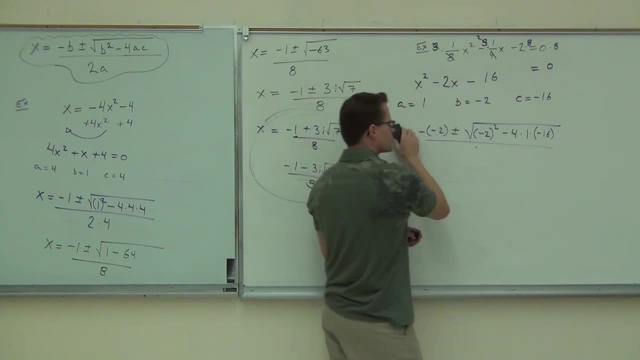 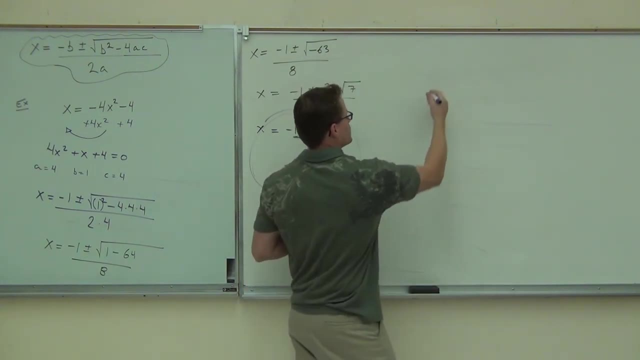 Would you really have to be a little careful what we've talked about so far? So just a lot of manipulation. There's only one thing I've got to do that's going to take you 10 seconds, but I promise it's going to help you on your test and your homework. 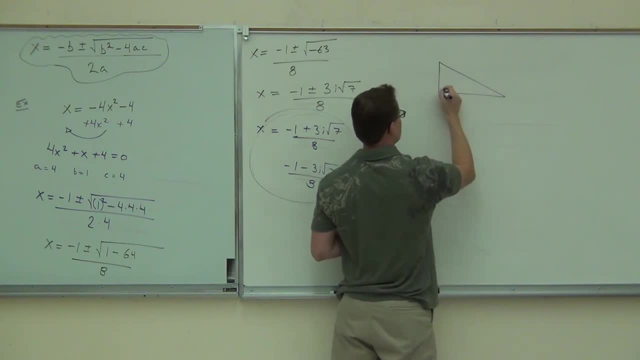 Do you remember the Pythagorean theorem? Yes. 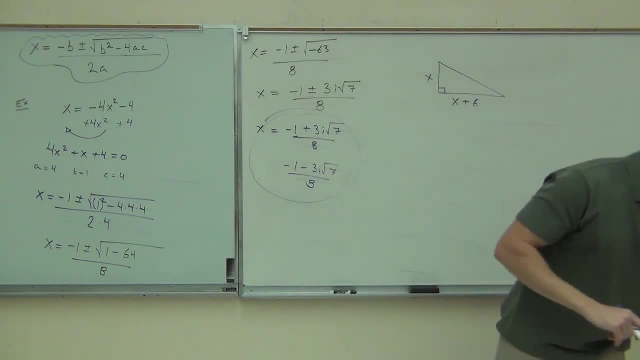 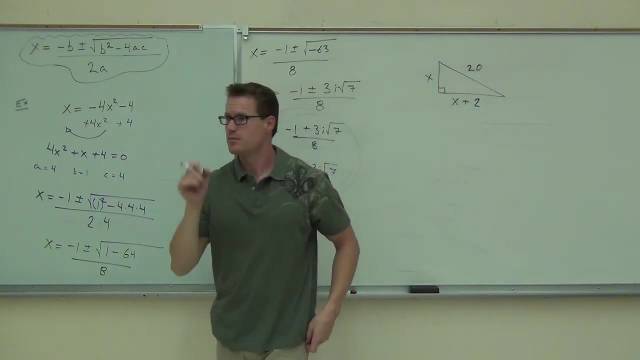 If I give you something like this, now let's make it a 2 just to make it easier. 2 and 20. Could you set it up? 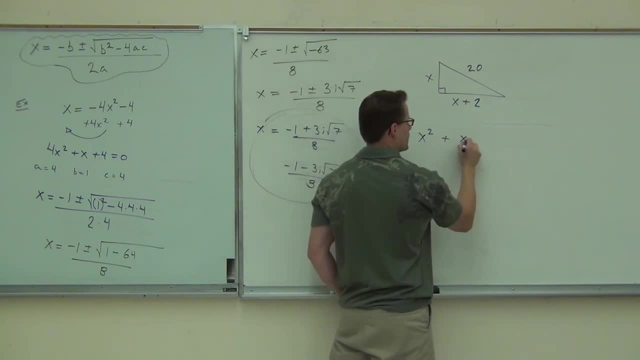 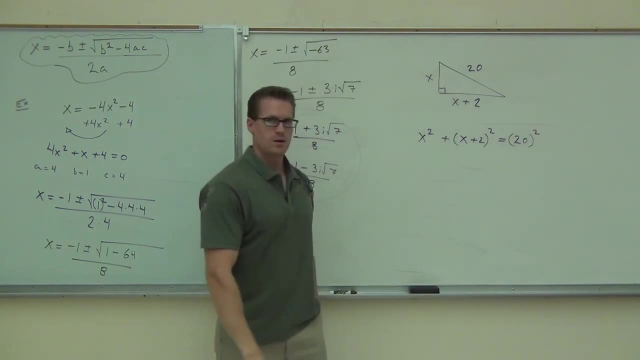 Pythagorean theorem says a leg squared plus a leg squared, notice the parentheses, equals the hypotenuse squared. You OK with that? What would you do now? 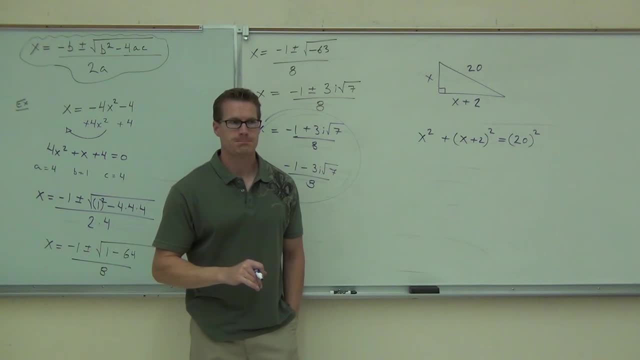 Put the FOIL method on the x plus 2. FOIL method. Yes. FOIL that, sure. 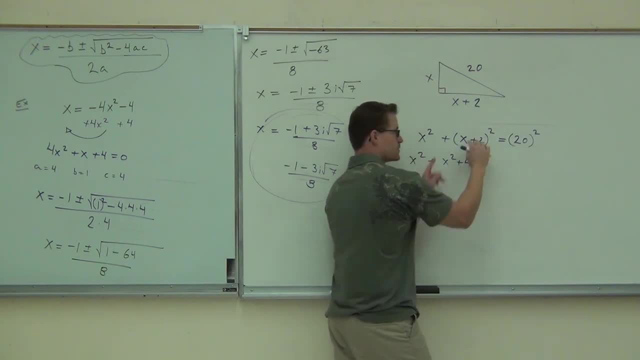 x squared plus x squared plus 4x, notice the little terms, you're going to FOIL, plus 4 equals 400. What now? Combine like terms. Combine like terms and get everything to one side. Get everything to one side. You need a 0 to use a quadratic formula. 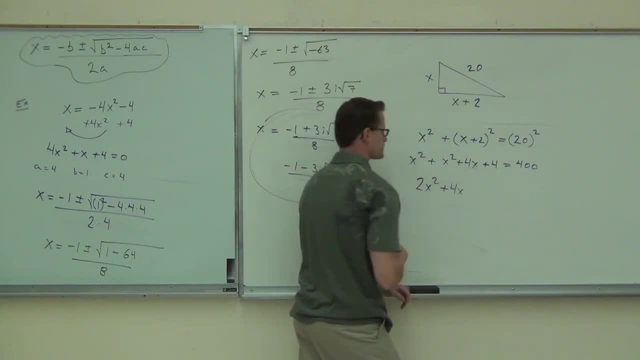 We'd have 2x squared plus 4x minus 396 equals 0. Yes, no? 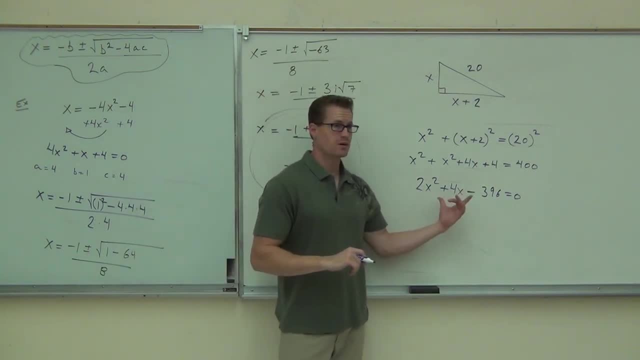 Now, could you use a quadratic formula? Yeah.